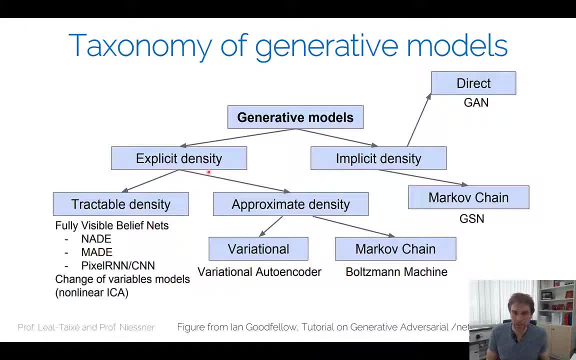 autoencoders. These kind of things fall into the categories of explicit densities, because here you have a loss function that explicitly models it. At the same time there's other generative networks, such as implicit densities. Generative adversarial networks is the main thing we will talk about. 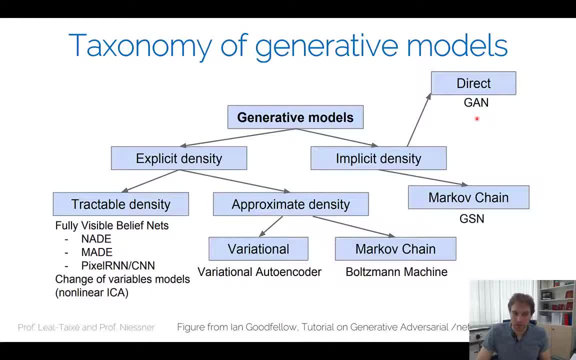 mostly today. that falls into that category. Here we are still learning a density, but it is not explicitly modeled. So we're going to talk about the density of the image And we're going to talk about a loss function And there's certain implications. if you do that, You have certain 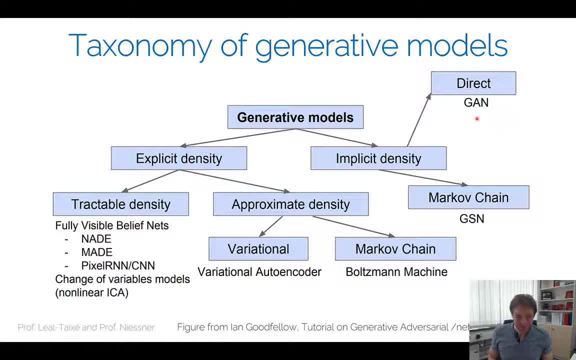 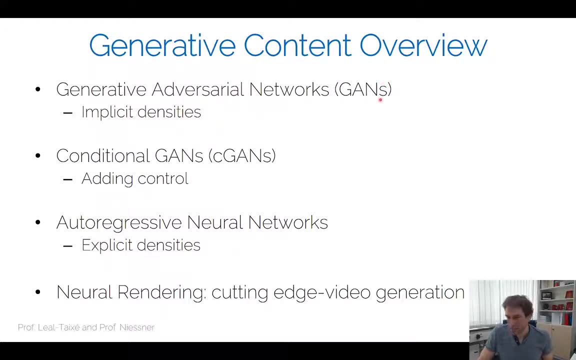 features, but also certain drawbacks, if you're having an implicit density. I would first like to give you a bit of an overview of the generative models or the generative neural networks we're going to talk about. And first of all we're going to talk about GANs, because most of you 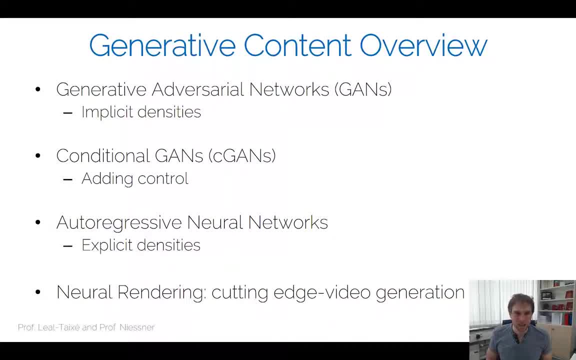 might have heard about them, But I still want to talk about it because they're just so relevant today. There's so many methods and so many different research works around GANs that, in one way or another, build on generative adversarial networks. We will also talk about conditional GANs. 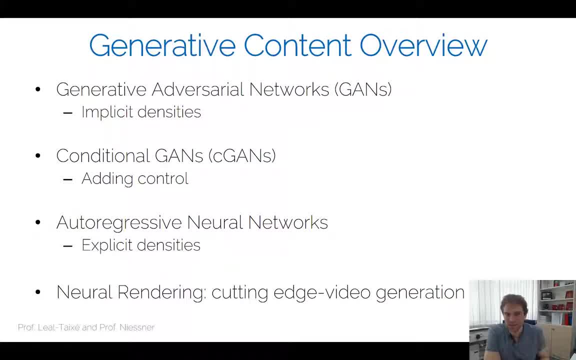 meaning that at some point we have learned some sort of implicit density with a GAN. At some point you want to control the generation process. If you're talking about a plain GAN, you don't have a lot of control. But we will talk about how can we actually make GANs useful for certain. 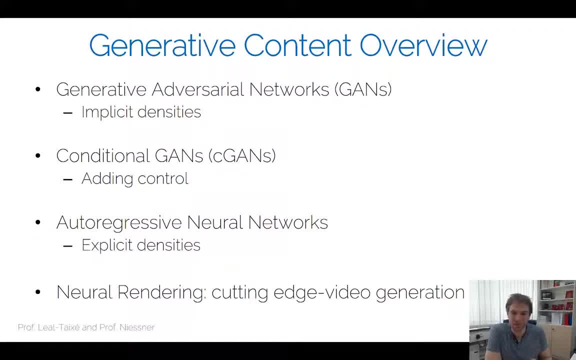 applications. How can we actually make GANs useful for certain applications? How can we force certain styles of images to be created? How can we force, for instance, a video or certain animations to be created, and so on- And I think this part here is pretty exciting specifically. 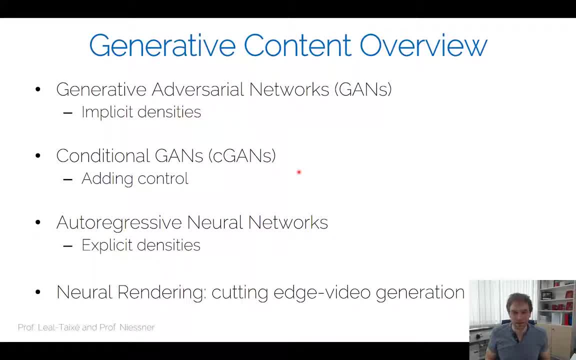 for, you know, content creation applications, artistic applications and so on. So when you're going to make GANs practical, this is very interesting because here you can basically give it the right control, depending on what your underlying task is going to be. We'll also talk. 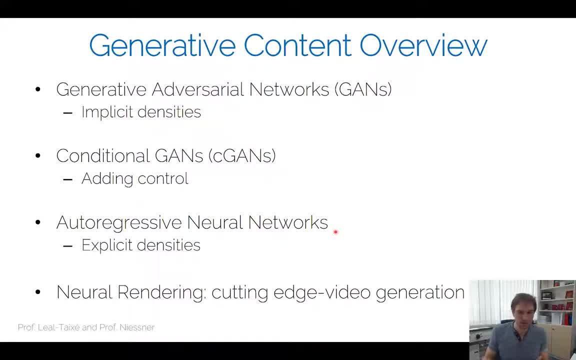 about autoregressive networks mainly because I think they're theoretically very interesting, because these are the dominant generative models right now that actually have explicit densities. They might not be as popular right now as GANs, but I think you know that comes and goes. There's. 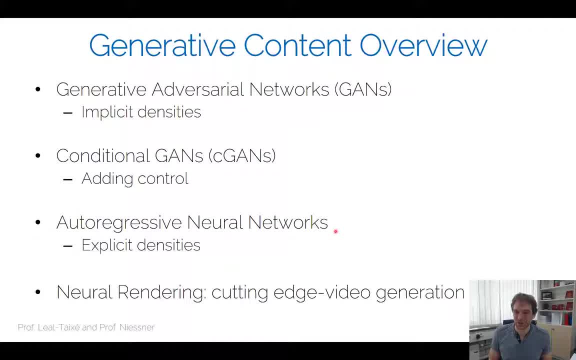 like certain research trends, and I think autoregressive networks are pretty important for various reasons, and not just in the visual domain, mostly for audios. Most of the state-of-the-art networks actually are autoregressive there. at this point We'll also talk about neural rendering. That's kind of an interesting thing that a lot of the research 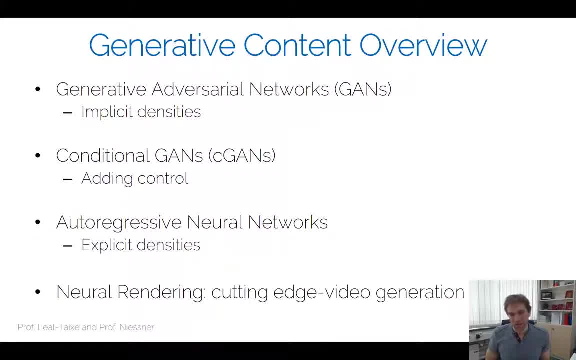 we're doing, for instance, in our group, and the idea there is: we want a couple. you know traditional generation methods, such as what we know from computer graphics, for instance, and want to combine it with generative neural networks. I will go into a little bit of detail later on what I mean by that, but I think it is fair to say that you know if you're looking at. 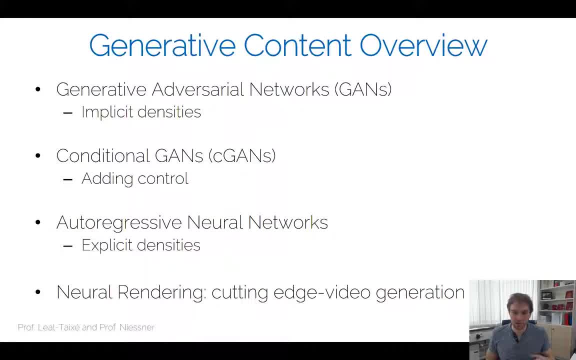 some of the progress in the research community in the last like two or three years. neural rendering has become a really big thing, basically, and you can now, instead of having explicit 3D graphics methods, you can use neural networks in order to to kind of generate cutting. 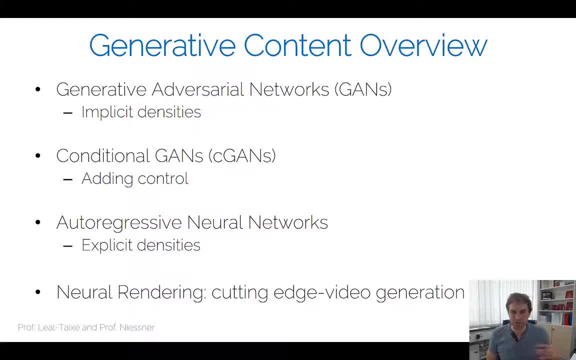 edge content, especially for video generation or for capturing 3D environments. This is currently one of the state of the arts. So, in a sense, we have basically two theoretical blocks. we want to go over the GANs and the autoregressive networks, and then we have the conditional GANs and the 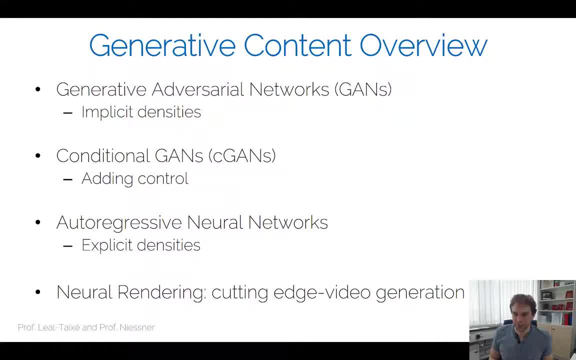 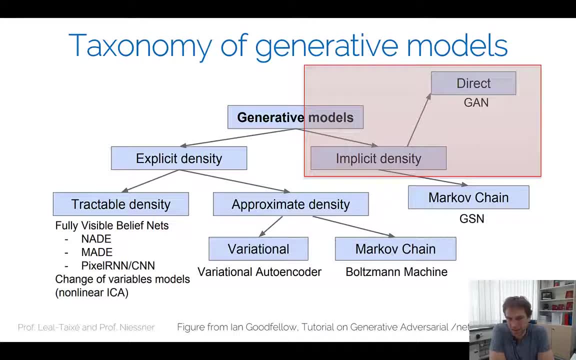 rendering techniques to make things a little bit more practical. Now I mentioned, I wanted to start with the GANs, and these are, as I said. they have the implicit densities and the idea is that we can learn these from a given training data set and then we can draw new samples from certain distributions. 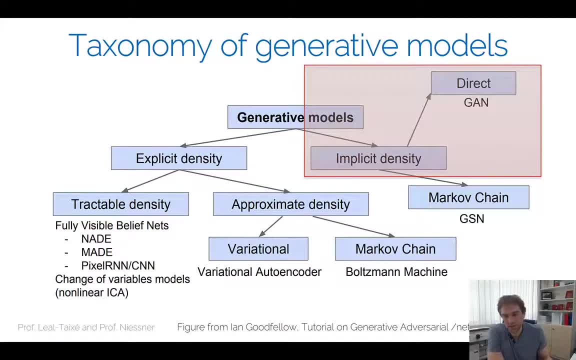 right, and then we can. these samples lie inside of the distribution, but they are new samples that are not identical with any of the training samples, right? So, for instance, if you have a data set of faces, you can draw a data set of faces and then you can draw a data set of faces, and then you can. 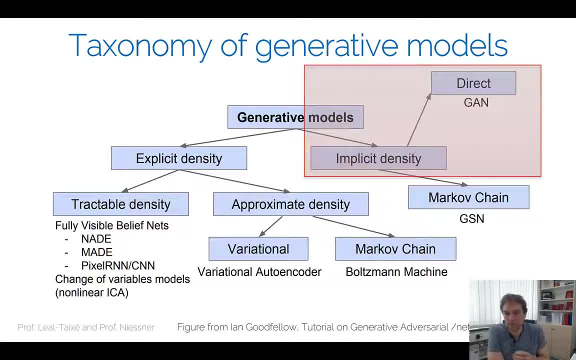 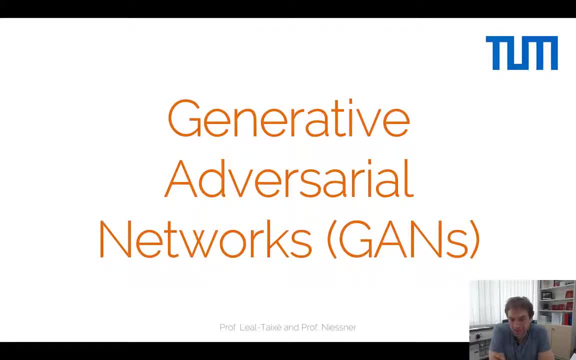 basically generate new faces. They still are faces, but you can generate new variations of the different people in these faces. Good Yeah, generative adversarial networks. I will probably always refer to them as GANs in the next few slides. They have reached a lot of popularity. 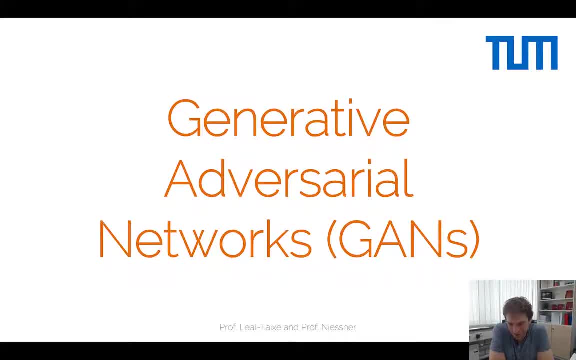 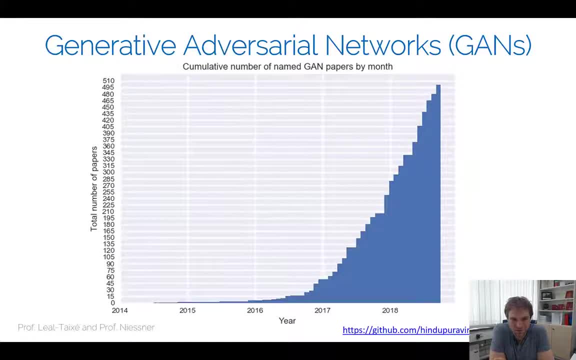 actually, and one thing to measure popularity is if you're looking at the number of research papers that have appeared. This is not quite up to date, this graph, it goes until you know, early of 2019, but you can see here is the the time period of papers, right, and here's the number of papers. 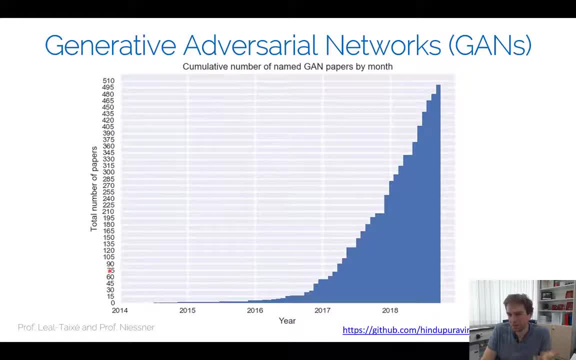 that have appeared at the respective publication venues. In this case, I think they're from archive. You can see, you know, like 2014, you had barely any GAN papers and now you have, per month, you have- almost 500 papers, right? So this is kind of a very- this is the very rapid growth rates of papers that 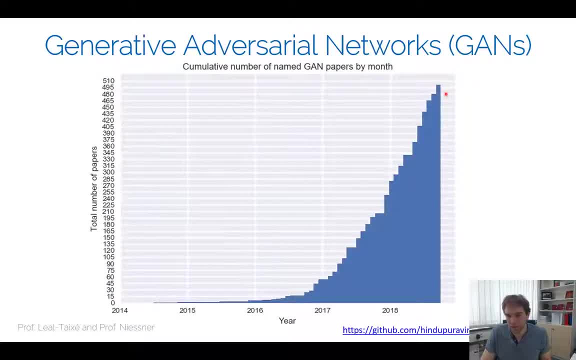 GAN in the title And this is pretty impressive, I think. so you can see there's a lot of people looking into it. Yeah, the reason why I think it's so interesting is because it kind of showed different ways now how to generate images compared to to standard pipelines and opened up a lot of 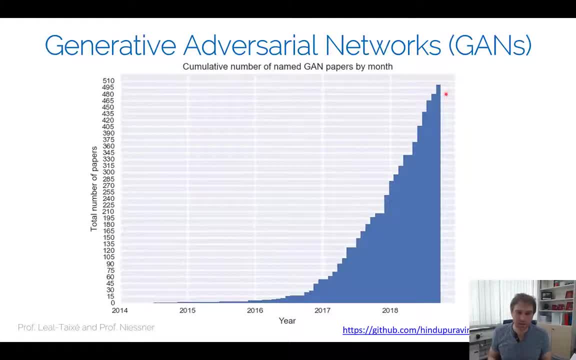 possibilities for practical reasons And we'll talk about this in this lecture and I hope at the end of the day, you know, we can all use GANs and and various generative models to do kind of fun stuff. Now I will. I want to quickly go. This is a very interesting topic. It's kind of a very interesting. 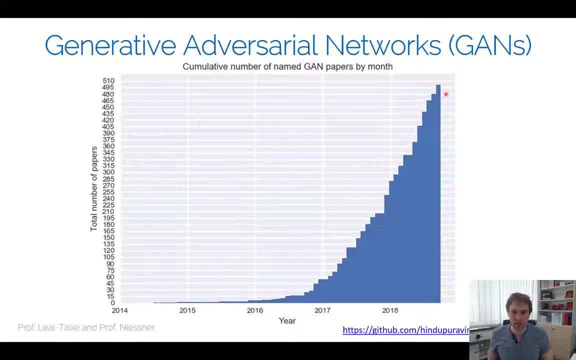 topic to me And it's really interesting to me because it's kind of a very interesting topic And I over the basics again, I know some of the things we have already covered in the introduction to deep learning course but just for completeness, not everybody might have heard it in the last. 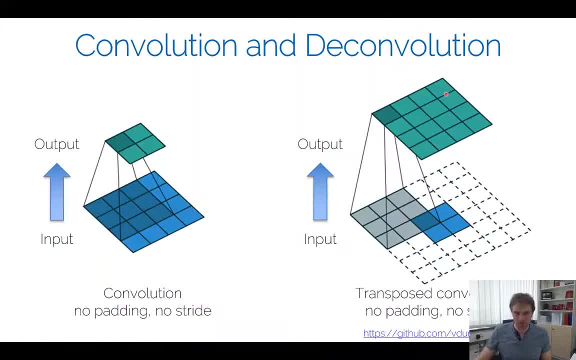 semester, so I still want to quickly do a small recap here. We have talked about convolutions and deconvolutions. I understand everybody knows what a convolutional network is right now. right, So we have here some input image. right, We're going to here have the output and we have this. 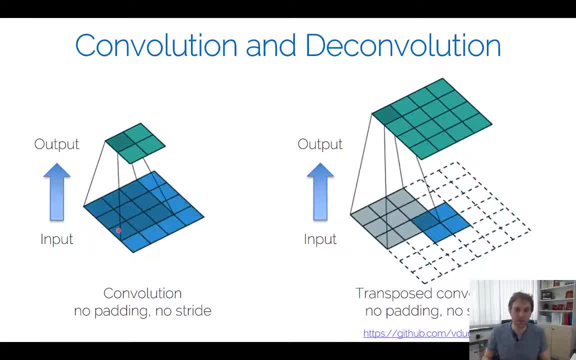 3x3 conf kernel that is being shifted over the input image and in this case we have four welded locations. There's no padding, no strides. so with this 4x4 image we're going to generate a 2x2 feature map with this conf kernel. Now the transposed convolutions are essentially the: 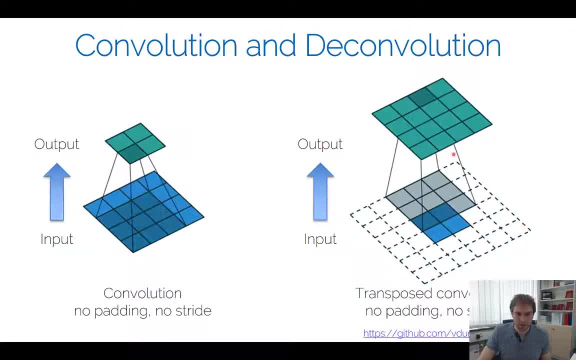 opposite, right. So here we have the input, here is this grid, here We have basically 2x2 welded pixels here in the input, and what we want to do is we want to make out of 2x2, we want to make. 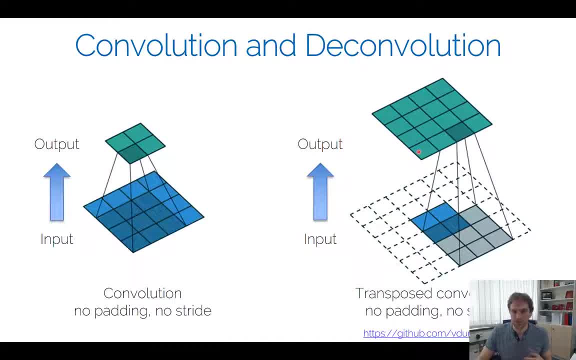 4x4 pixels as the output. Yeah, and the way you do this is kind of this learnable upsampling. In this case, again, we have no padding and no stride. In this case we have these four feature locations, but basically we just expand the values, right, And then we run this conf kernel. 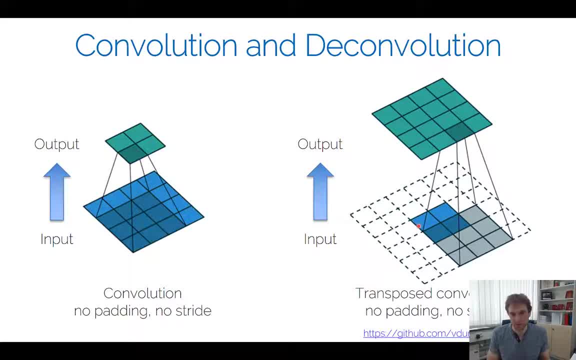 over it. Same thing as convolution, except now we have a transposed kernel and this way we can basically have: instead of going down the resolution, we can go up in the resolution Now using the. well, I should say one thing right: Obviously in the literature, deconvolutions are. 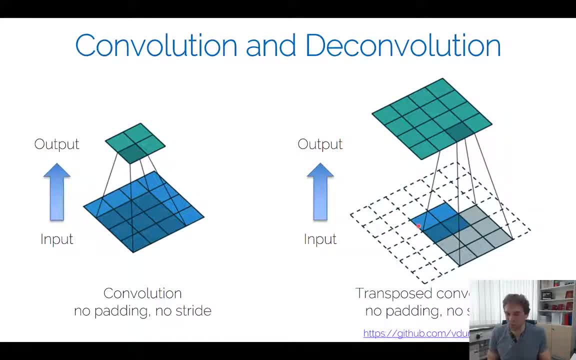 often renamed in various different ways. We have seen them as upconvolutions, transposed convolutions, deconvolutions- same thing, different people call them differently. I don't have a strong preference. Most of the time I will just say it's a deconvolution, but that's just because I got 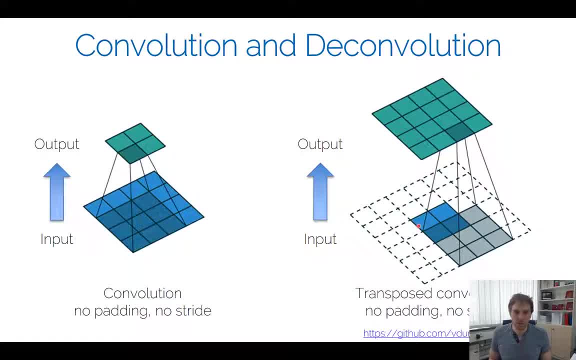 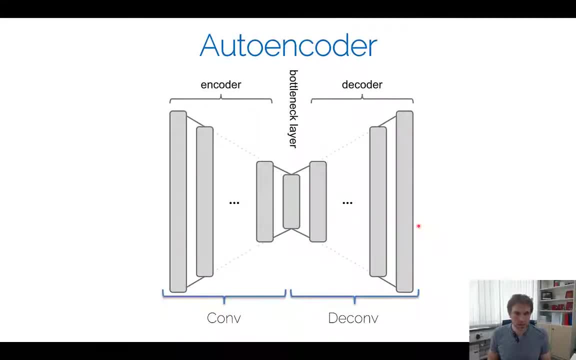 used to it, but it's not like the other terms are necessarily wrong. Yeah, with these building blocks, with convolutions and deconvolutions, you can devise architectures such as autoencoders. The idea of an autoencoder is we have a series of convolutions that go from a higher resolution. 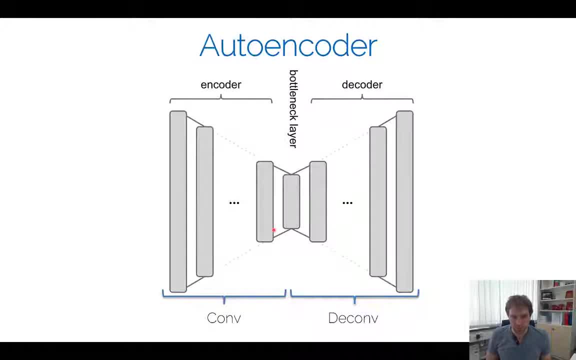 input to a lower resolution feature map. This feature map here in the middle is called the bottleneck layer. It's doing what it says. right, It's a bottleneck. Basically, it's compressing the content to a smaller dimensionality of the features here, meaning that you have to learn some. 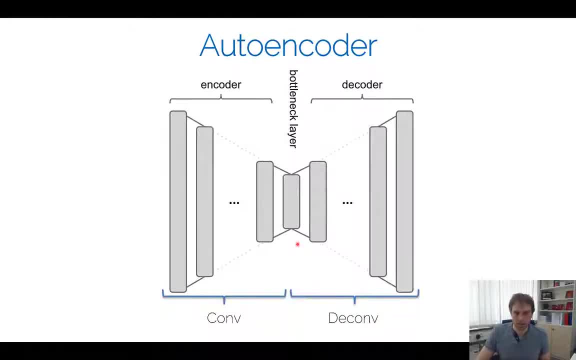 sort of encoding of the image. Then what you do is you have a decoder. This is composed of a series of deconvolutions, so we have this learnable upsampling. We go here from this bottleneck layer again to the original resolution. The idea is that we have these convolutions, we have these. 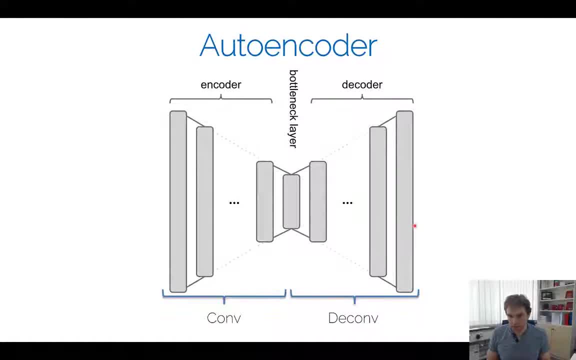 deconvolutions. This can be a fully convolutional architecture, right? Sometimes you have a couple of fully connected layers here in the middle, but often you don't have that. You just have a fully convolutional architecture. With that, you can design this architecture now, right. The question is: how do we train that? 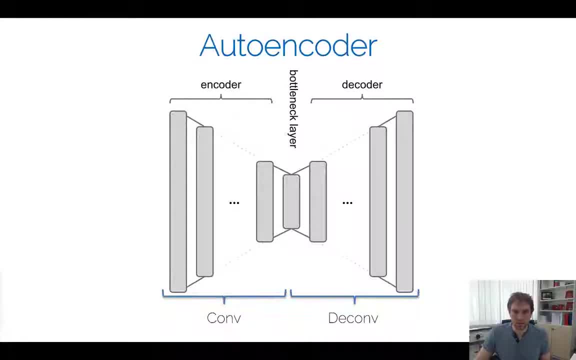 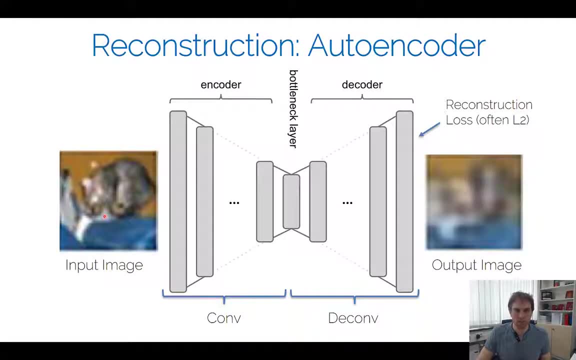 Well, the most common thing for autoencoders is we're going to have a reconstruction loss. What we're doing here is we have some sort of input image on the left-hand side. We're feeding this into our encoder. with the bottleneck layer It's being compressed down to a lower resolution. 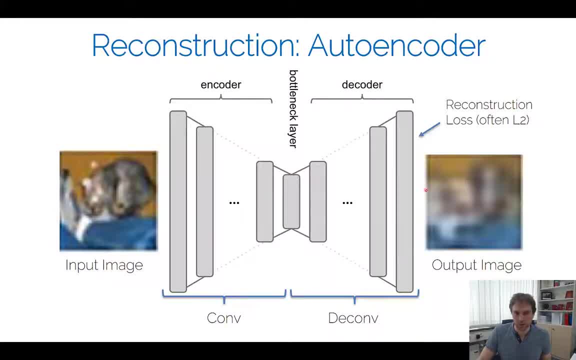 feature map. We have a decoder that goes up to the original resolution. We have an output image. What we do is we have a reconstruction loss that says: oh, this output image should be similar to the input image. You can use an L1 or L2 loss here. It's a very simple regression loss, basically. 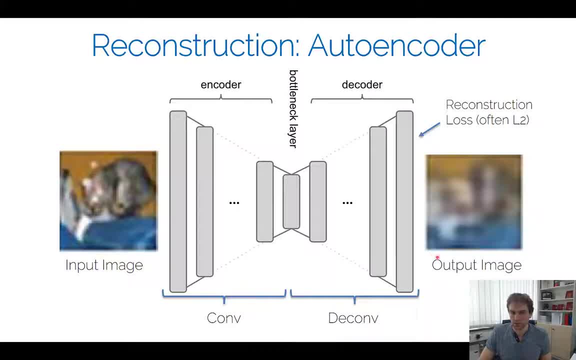 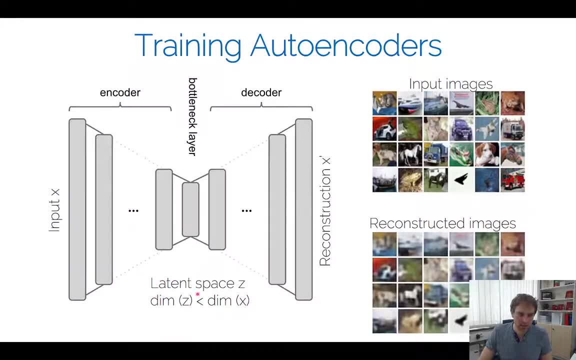 The network is being optimized such that it wants to do this reconstruction. Practically. what you have is this latent space Z here This is what we get in the bottleneck. This dimensionality is typically significantly lower than the input. Of course, the spatial resolution gets smaller. the feature map resolution gets higher. 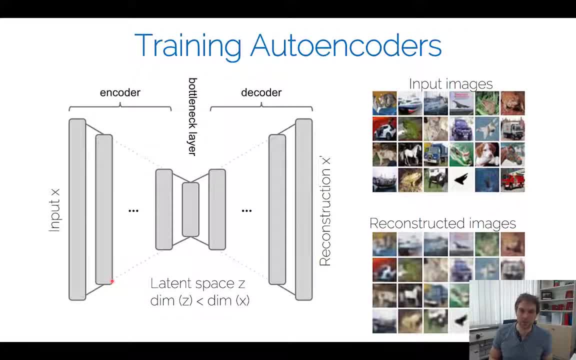 but the total dimensionality of the latent space Z is supposed to be significantly lower. If you do this and train this, you have here a bunch of input images and you're training this and you're getting a series of reconstructed images. There's also the distinction right now if you're saying you have a training and a validation set. 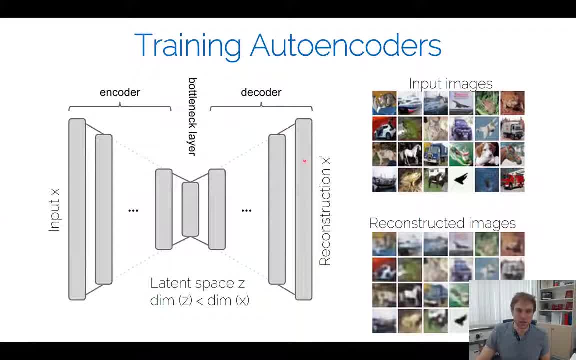 if you're taking a training set, essentially what this network here is learning. it's kind of learning a lowering approximation of the input. It's actually very similar to what a PCA would do, except that this is not a linear but a non-linear model. but you have the same idea. 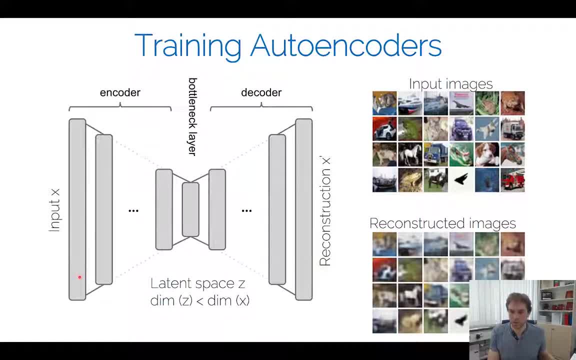 that you have kind of this encoding of a higher dimensional input, in this case an image, into a lower dimensionality in the bottleneck layer. Then you can do the reconstruction by having the loss at the end. At the end of the day it's a self-supervised learning. A lot of people call it unsupervised. 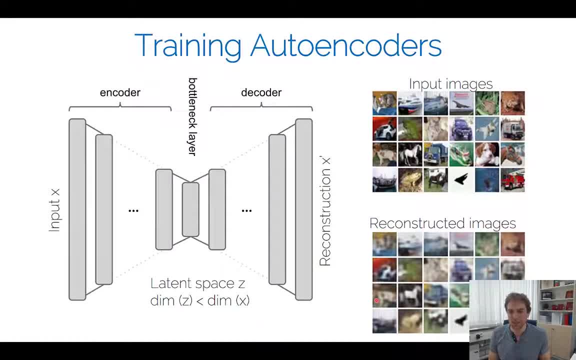 learning. I like to call it self-supervised, because you still have a loss here. but the nice thing is to train an autoencoder. you don't need any additional annotations or labels. It's completely self-supervised. You're going to feed in an image. you're going to 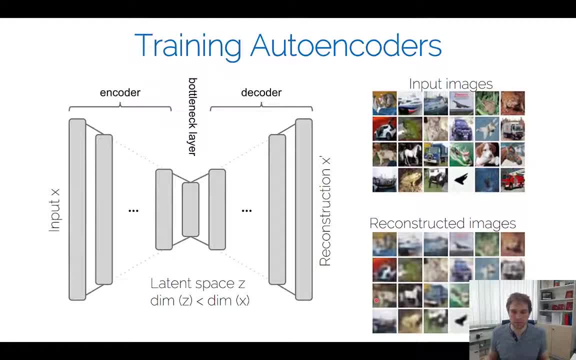 reconstruct the image again. so all you have to do is you have to have a data set of images, in this case to train it. Now we can argue: what are we learning? The whole, at least what we would assume. what we would learn- is we learned kind of a compression. 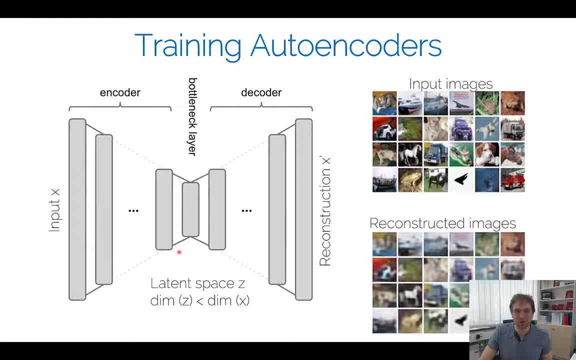 network. We're compressing this high-level input into a lower-level feature map and then we are going back to the original resolution. In a sense, it's like learning some sort of compression. It's not perfect. It's not a lossless compression, as we can already see here. 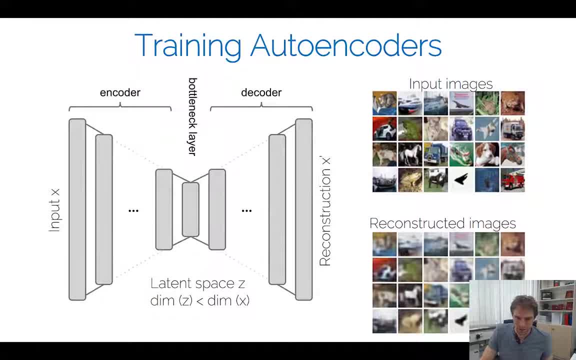 We have here the input images and we have here the reconstructed image. You see, these images are a little bit blurry. That is based on the fact that, well, depending on how we do the optimization, it's based on what kind of loss we're going to use. We will very quickly see that the loss 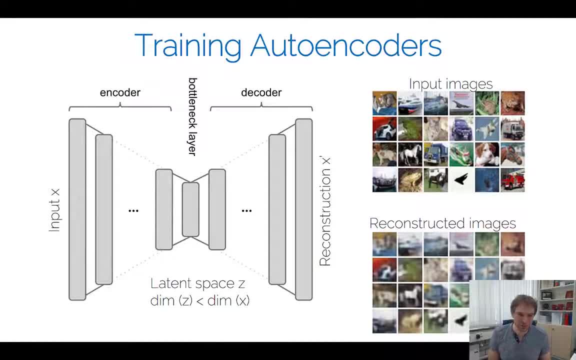 the L2 loss might not be the ideal one because essentially learning some sort of mean average over the training set and so on. But I'm sure you've heard of autoencoders in the context a lot for unsupervised learning. you can use clustering in this feature space. you can find dominant axes similar to principle component axes. So you can also use constant behavioural Baek Dur鍱 tea because we have pre- atmos coração part of the interface here. So you typically have to have a famous property here that brings theissa N England when working over. 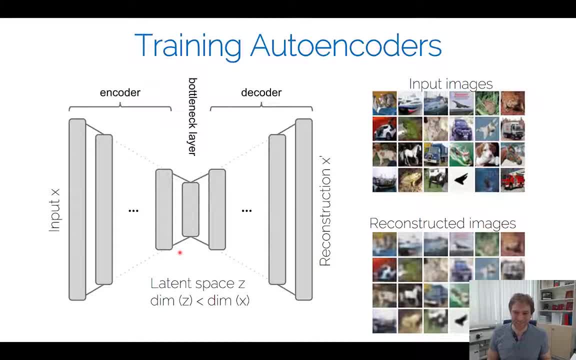 so many subdomain blocks and i think that might be one of the things you can. you mightค Be better involved with the sorting these desperatum Missions which have brought it across into our work here. similar to principal component access right. this is why i'm i'm making the comparison to pca here. 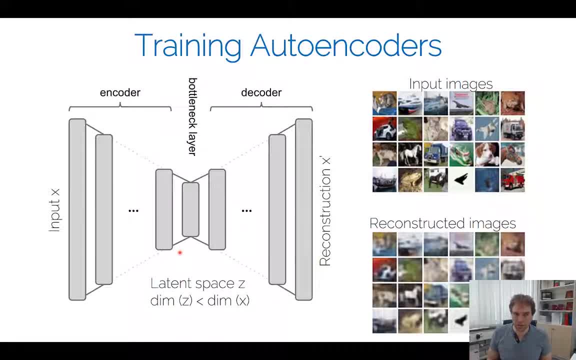 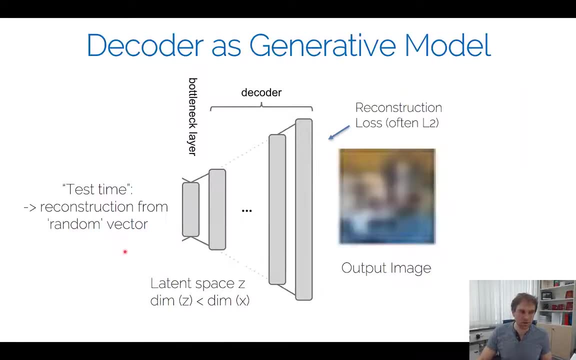 you can kind of find clustering in your data set. but now we wanted to talk about generative models. the question is: how is an autoencoder useful here? well, the idea is, what we can do is we can train this autoencoder at training time, with the training set, and then at test time. what we're 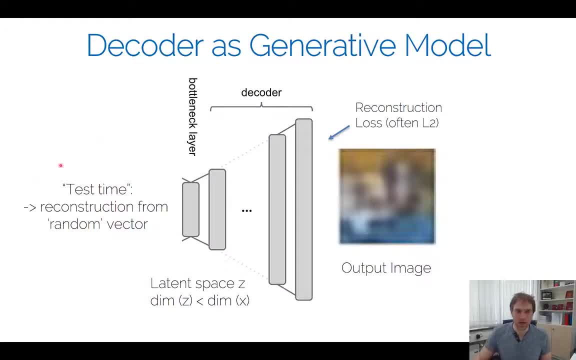 doing is we're simply- we're simply chopping off the encoder part, and now what we do is we just have a decoder, so this decoder was pre-trained in this case and at test time. what we do is we just feed in random vectors here in the latent layer and then we're hoping we're getting an. 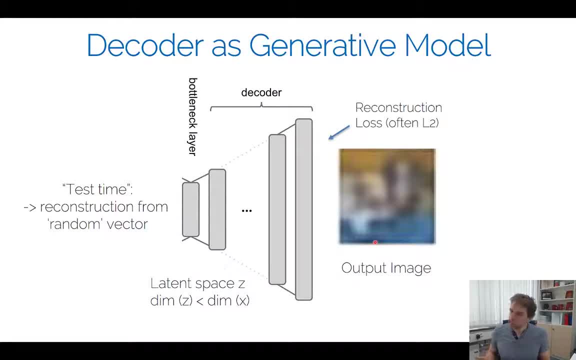 original image as output. again, right, and assuming we've done a good job at, you know, learning this, if i'm going back quickly at learning this latent space here from the input, we assume that we have a reasonable, we have a reasonable decoder that can kind of figure out how to make a real image. 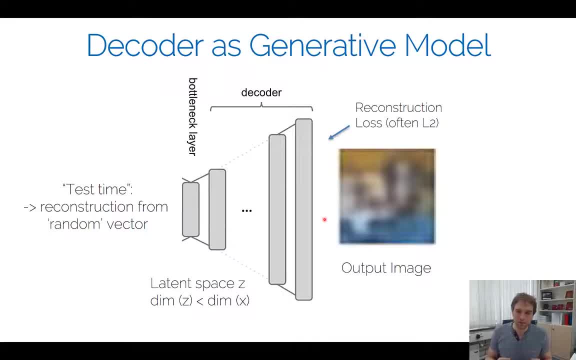 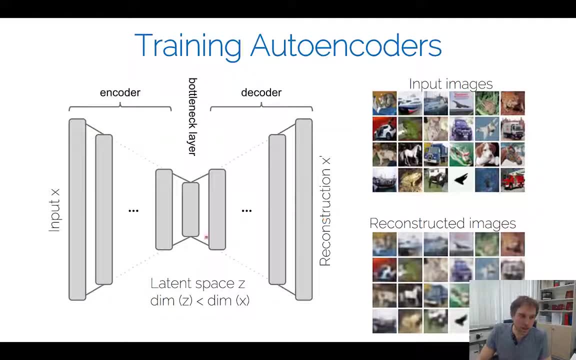 out of this one again, so you can kind of reconstruct from this compressed representation a real image, right? so the idea why i mentioned compression here is a good one, because if this is compressed then i can kind of have the space of all valid real images of a certain domain in here encoded. 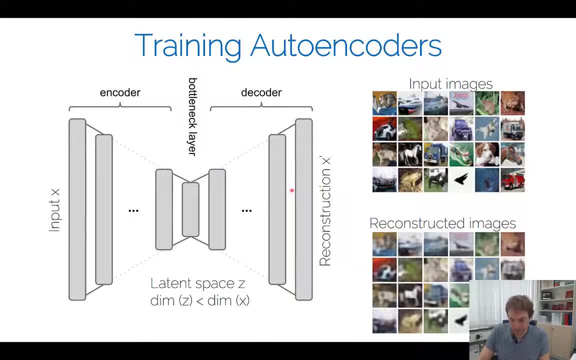 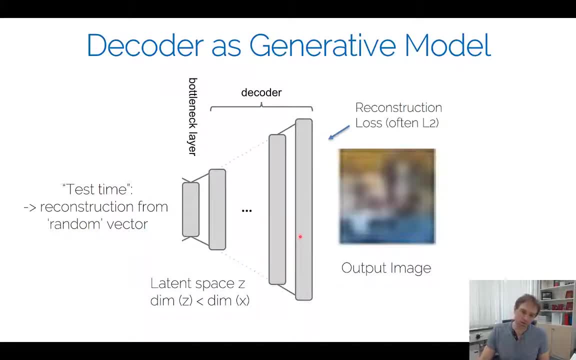 this is a very dense space compared to the possible output space, and if that is the case, right you, you would assume that whatever you're feeding in here, you're going to get a reasonable image as output. now, of course, in practice it's not going to be so simple. of course, this 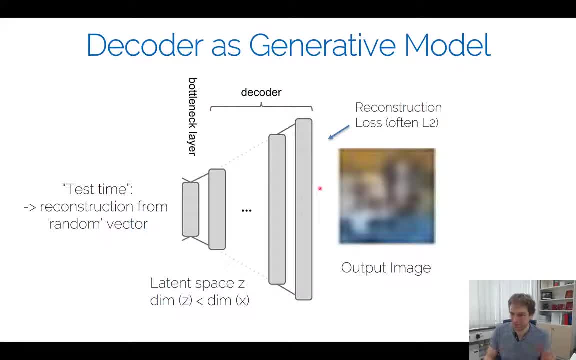 space is still pretty high dimensionally in the latent space and you can still, you know, get a lot of garbage as output. but that's kind of the high level intuition, what you, how you can assume this right, um, okay, but anyway, so test time, what we do is we? we just feed in a random vector here. 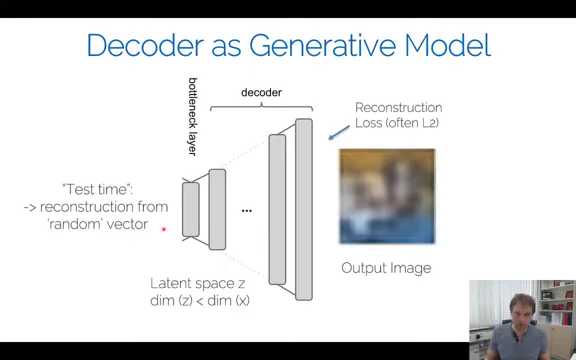 so, and we want to do reconstruction from this random vector, right, um, and then we're going to get um, we're going to get an output image, and what you can do also is you can say: well, you pre-train the autoencoder, but you can also go ahead and say well, 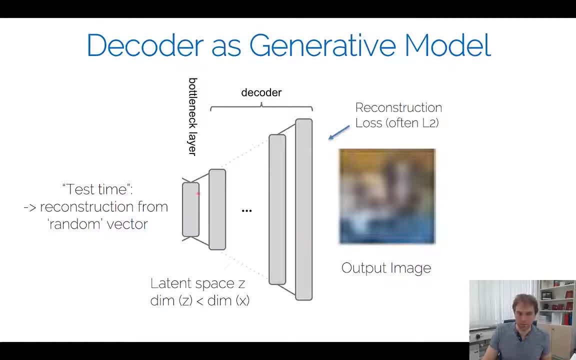 you know, instead of pre-training it, i'm just going to train it by, by feeding in random vectors here to begin with, and then you're reconstructing the output image. right, so you can also train directly on this one. so you don't have to pre-train on the autoencoder itself, but you can. 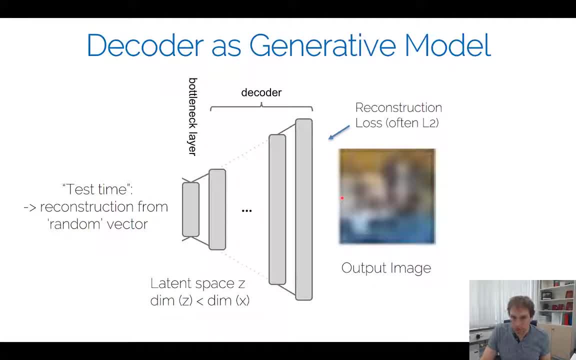 also just random vector, give me some output, and then you can also go ahead and say: oh, because i trained on this. i can also add some sort of semantic meaning into this here, right, um, depending on what kind of trainings that you have. so you can say: oh, if my first, my first component of my 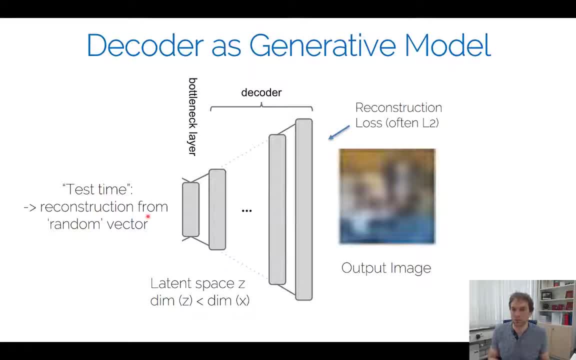 latent vector is a random vector. i can also add some sort of semantic meaning into this. here is going to be um having a high value that corresponds to certain semantic correlation, what we see later on, um in the output image. in this case, um, yeah, in this case, what you would 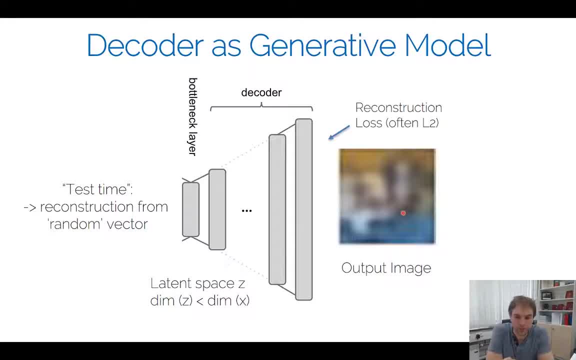 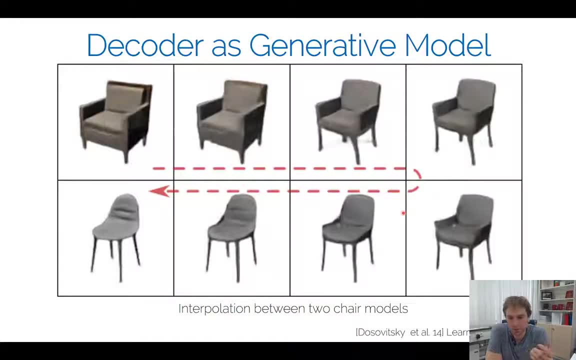 assume is that, you know, the network just learns a mapping from these, uh, from the latent space to the respective output um, and this is one of the very first works um. this is actually a paper from alex dasowitzky. he was in freiburg um at the time, and you can train a network like this in the 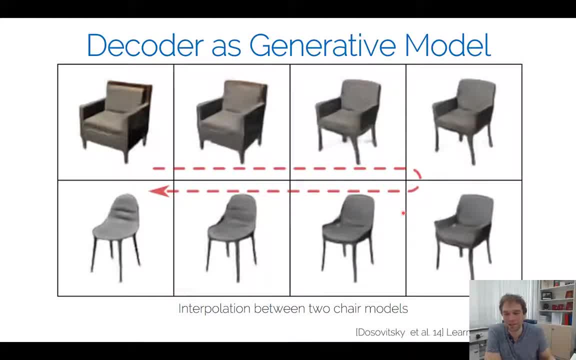 data center. and then you can go ahead and say, oh, i'm going to interpolate between my latent space, right. i can go ahead and say, oh, i have a latent space of this image, i have a latent space of that image and i just want to do a linear interpolation in this latent code that i've just optimized. 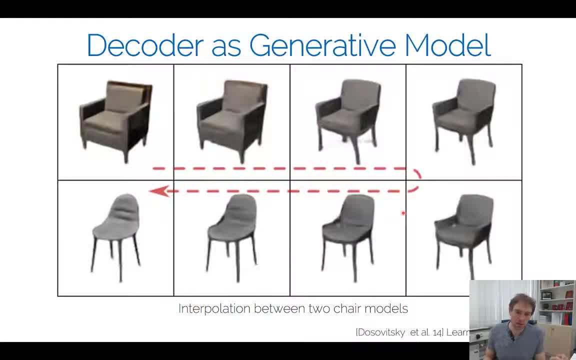 for, uh, and then i'm getting intermediate results that show kind of a natural transition between the two images. and these guys have been doing this on um. well, we, these guys, have been doing this on single on single shapes. so it was a very, very early paper. you see, it was 2014. 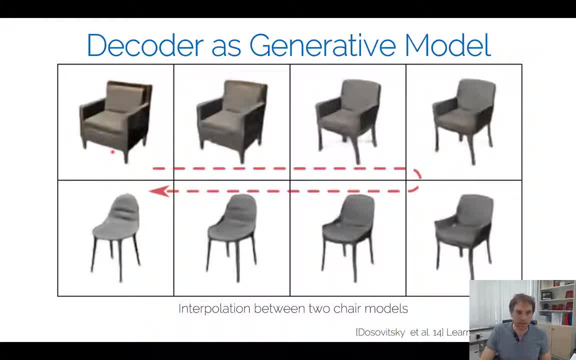 is the publication date? um, so they could basically interpolate between these two chair models. this is the source, this is one image that they have. they compute a latent code for that and they have another one here: uh, this is the target, and then they simply interpolate in the latent code and 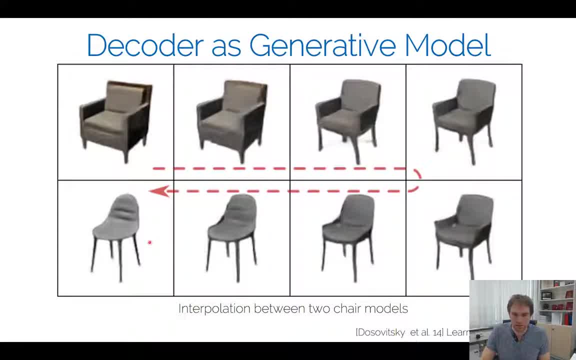 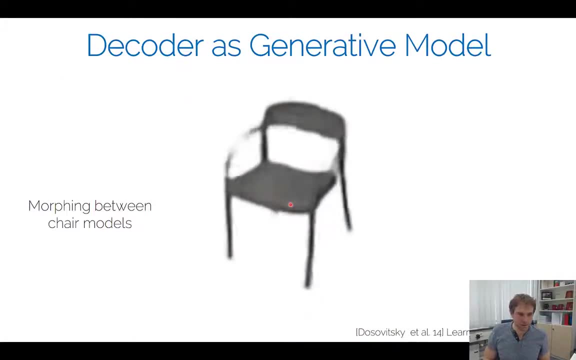 this like, gradually, transitions between these chairs, and the nice thing is, now we have our first generative model, meaning that we can now, based on this latent code, we can control or we can generate new images here. very good, um yeah, practice, you can also change viewpoints here. you, you can, uh, morph between. 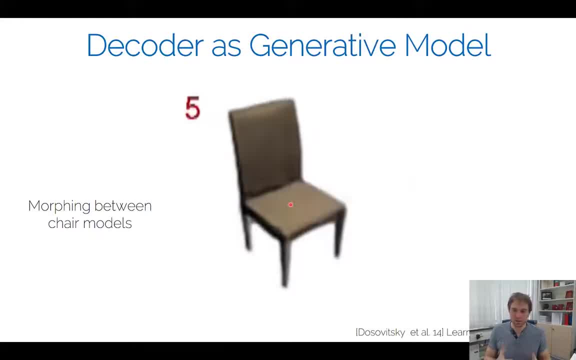 the chairs right, um, and you have some certain control of the appearance. you see, this is not very sharp. this is not an artifact right now in the video, this is actually um, a little bit low resolution, um, um, but again, this is a paper from like six years ago, um, but i wanted to. 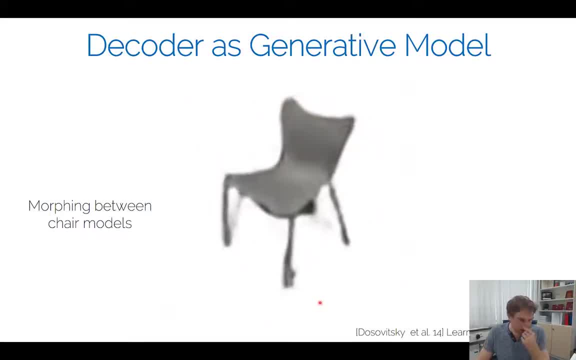 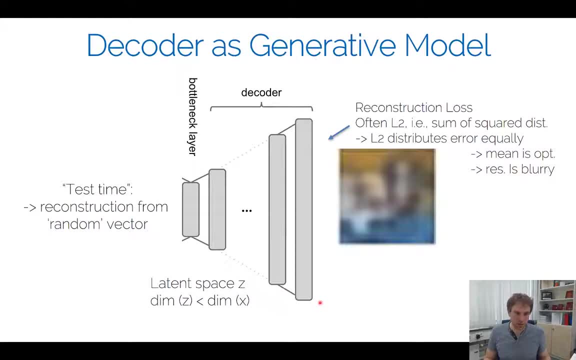 highlight. this was one of the first papers that actually had this explicit control. now there are a few other papers that are available and they're very similar to sort of you know therell and the little bit and a lot of the other papers that are available are. 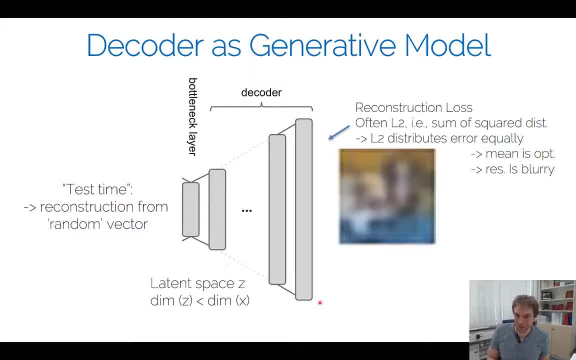 there, um, and i wanted to highlight that we have a kind of a very different approach to this um example, and that is, we have a lot of different models, and that's what we're really trying to do with this model here. so we have a very simple uh yeah, like we're creating some uh, uh, un-latent. 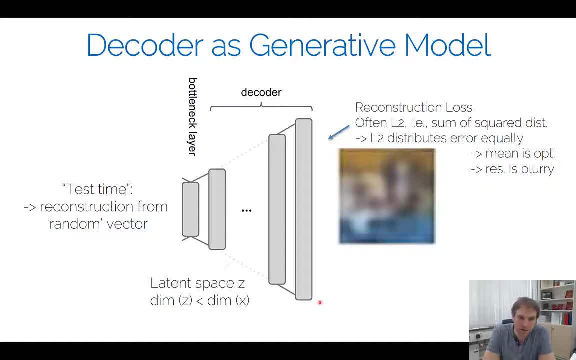 code to a respective target. um again, this is still the same idea. we still have this simple, uh yeah loss that i mentioned. that's what a lot of people do. you can use, of course, an l1 or hooper loss too, but in practice you have one of these losses and if you're having an l1 loss, um the optimum. 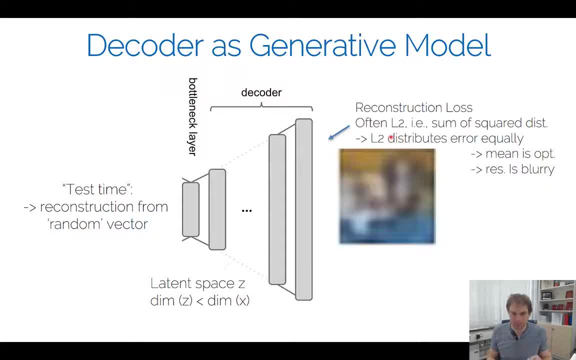 is kind of the mean right, like you always tend to blur, because if you have one outlier, you have like a sharp edge that gives you an outlier in the loss. the network will favor like smooth transitions over sharp edges. it's just naturally when you're using an l2 loss, that's by definition. 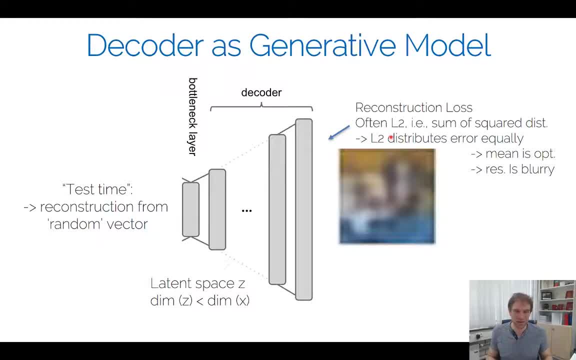 what an l2 loss is doing. so it's not gonna gonna favor like outliers um, but in this case we care about these outliers because this is where we get sharp edges that make an image look, look realistic, right and less blurry. so the idea now is, the problem is we want to replace this l2 loss. 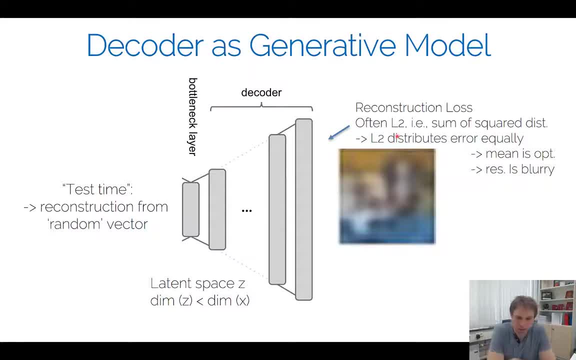 and well, ideally, what i would like to do is i would like to go ahead and tell you what is a good loss function that tells me, is it a realistic image or not? right, what, what, like? how do i do that? well, i'm going to look at the image and i just know it immediately, because i have a good sense of what. 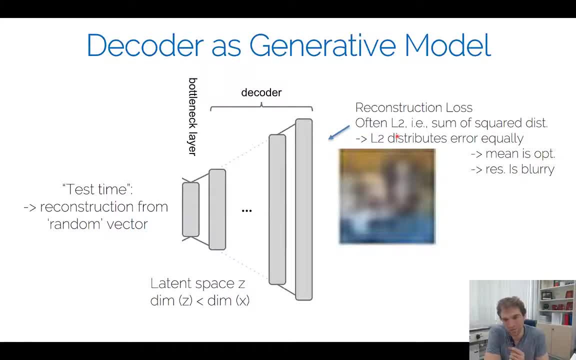 makes a real image and what's a synthetic image, right? um, but if you're telling this a loss function, this is more more difficult, right, and the core idea now is, instead of using like a fixed function here, what we would like to do is we like to learn that function. so, in other words, we, in other words. 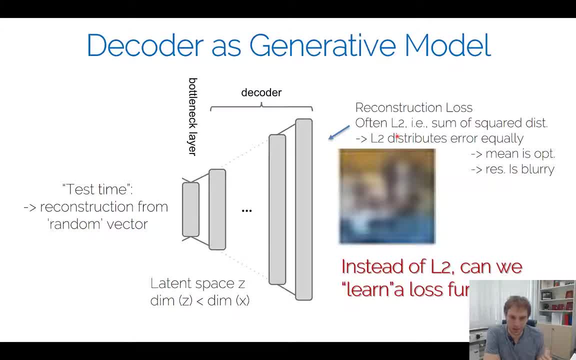 we want to have, um, a function that tells me how realistic is the image, or maybe not even realistic, so so how much does it match a certain distribution? so if i have a training distribution, i would like to train a loss- that tells me, oh, like, how, how, how good or how well does it match my distribution? 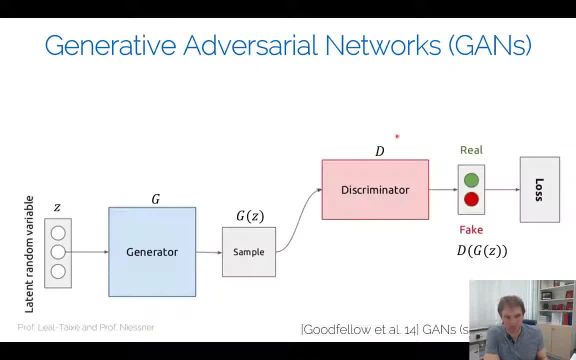 and this is the core idea of gans, this is the the core idea of a generative adversarial network. so here, what we're doing is, well, this part here is our, our decoder of an autoencoder. basically, it's the decoder part and we have in here our laden vector. 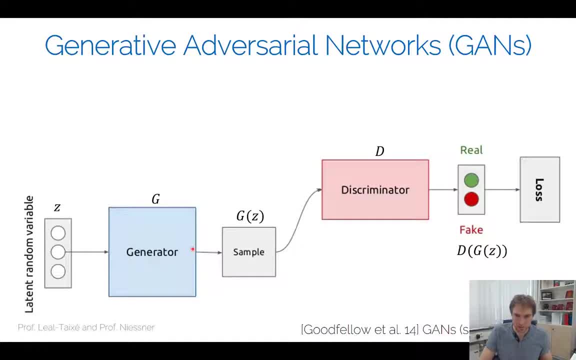 which we had before. we have here our generator, which is nothing else but a decoder network. right, it goes from a lower dimensional feature vector. in this case, it's a random variable, but it could be a lower dimensional feature vector too. it goes to an image, in this case. that's our sample. 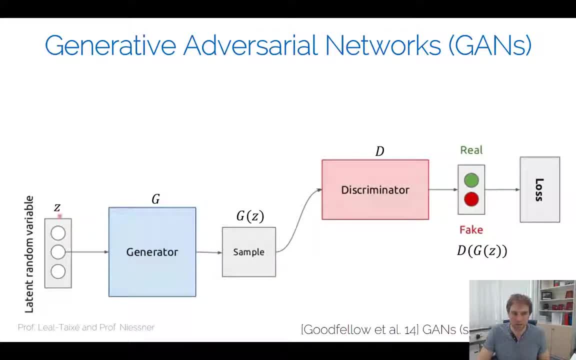 so the generated g takes us input the random variable z, that's the latent space code, and then it generates an images output. and now, instead of having l2 loss here, what we do is we feeding. we're trying to learn: is this a real image or not? and since we have no clue how to define, 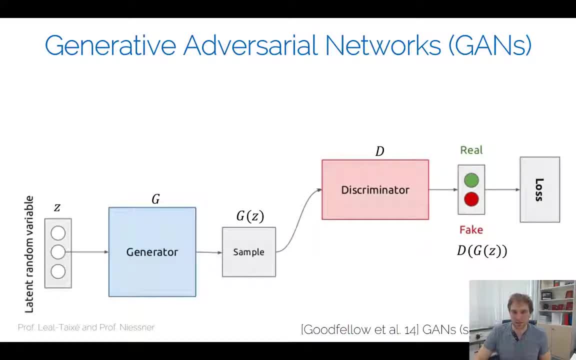 this loss function. we just use another neural network, in this case, our discriminator. this is a second neural network, that is a binary classifier that tells us: is this image that we just generate with g, is this real or is it fake? and this is our d, this is our discriminator. 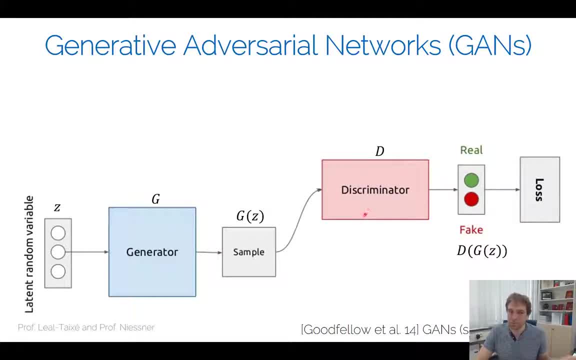 now, how does the discriminator know whether this is real or not? he needs to have some comparison to a real image. um, so what we're doing is we have a binary classification task and we're feeding in real samples and fake samples, and the discriminator tries to distinguish whether. 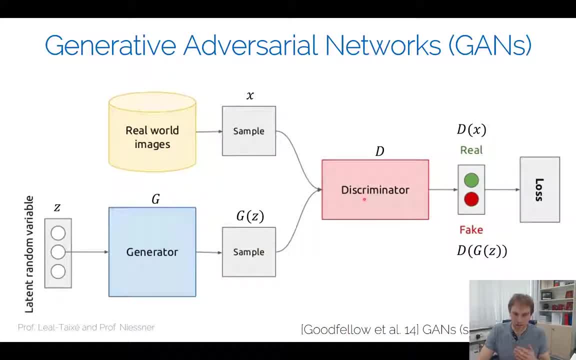 this one, or whether it tries to figure out for a given sample, is it real or is it fake? so what we do is we randomly feed in either real or either fake ones, and the discriminator is being trained. is it true or is it not true? with a simple binary cross? 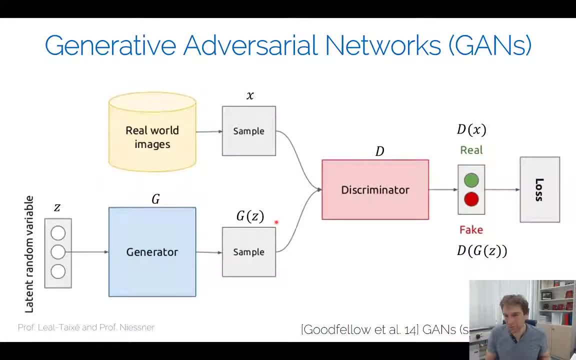 entropy loss. and the idea is, of course i'm not going to feed always this one in, so i'm just going to randomly feed in fake and real samples, right? so the discriminator um has to figure out based on the content of the image. is it real or is it fake? um the idea why we do have the discriminator, though. 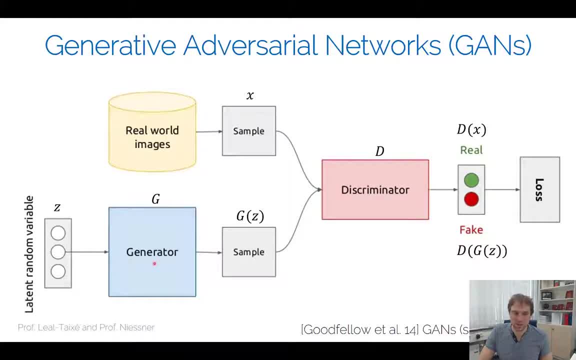 is not that we have a discriminator at the end. the idea is that we training both generating discriminator at the same time, and the goal of the generator now is to make sure that it fulfills this kind of learned loss function from the discriminator. and the learned loss function means i want to trick the discriminator, i want to make sure. 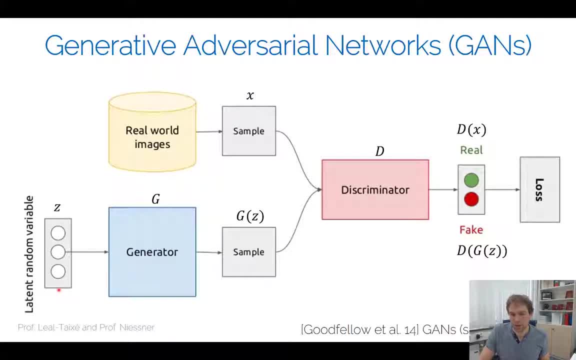 that this guy here can generate images that this guy here cannot distinguish anymore from these ones. right, if i had a perfect discriminator and i i knew exactly: oh, that's a real image or not, i can generate an image like that that this guy can't tell apart: it's real. 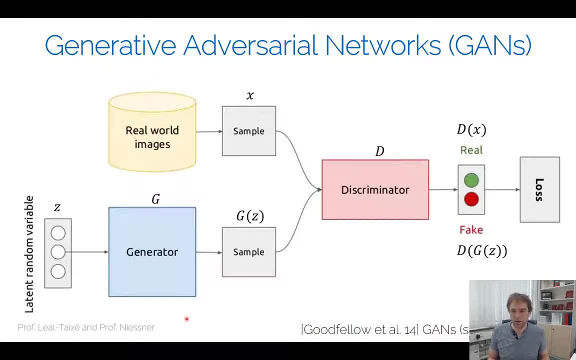 There is no reason. it doesn't work and it should be true or lie more than by definition, has to be a bill image. Now, it's a little bit more tricky than that, right, and the reason why it's a bit more tricky is because, well, if this is a fixed network, 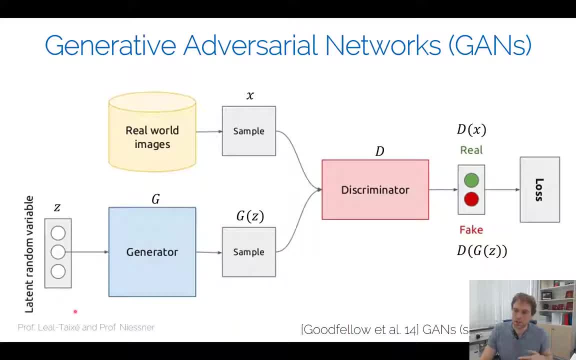 then you're going to have this problem that if I'm just training a generator, you will just generate some artificial noise- we call this adversarial noise- that will be generated eventually. that will trick this network. So you have to train these two things at the same time. you have to train 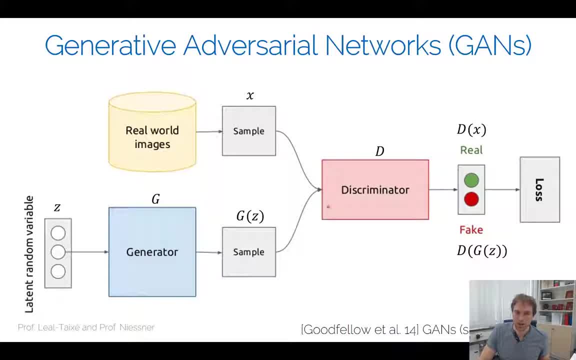 a generator and a discriminator at the same time, and eventually the discriminator will give you gradients that help to make the generation better. That's the core idea of GANs. This is why it's an adversarial network: The generator and the discriminator. they fight each other right. 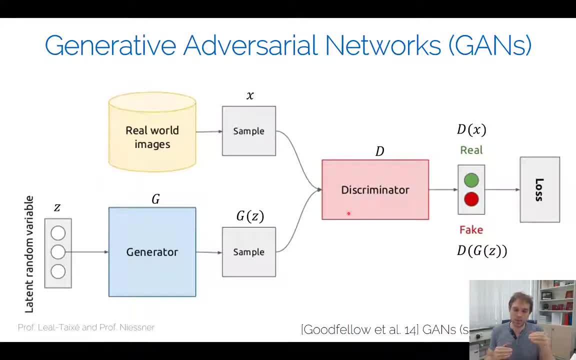 they try to trick each other. The generator tries to generate samples that look real, that the discriminator can't tell apart from the real images anymore, and the discriminator tries to tell apart whether this is a real or not a real image. Okay, typically for the notation here, we typically 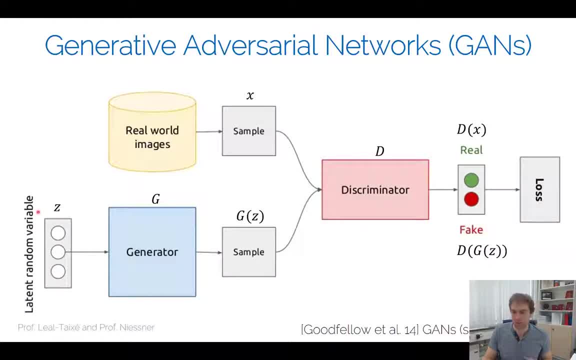 call the latent random variable. here is z. this is just a random vector, typically sampled from a Gaussian, or could be a uniform distribution too, Most of the Gaussian. we have a generator, g. we have g of z, which is our generated sample. we have x, which is our real world image, real world. 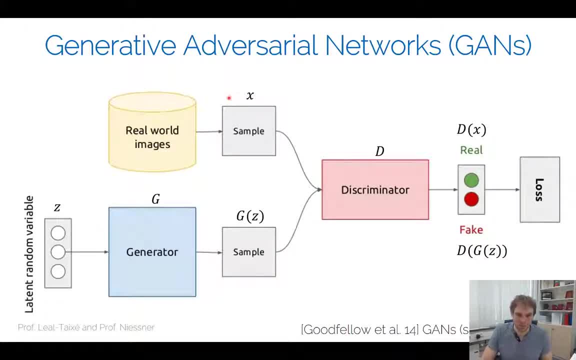 sample. again, it doesn't have to be an image, but for the real world sample we have a generated sample. we can mostly do it for images. right now we have our discriminator d and d of x, should you know, is the real sample and the discriminator should say, hey, it's real. 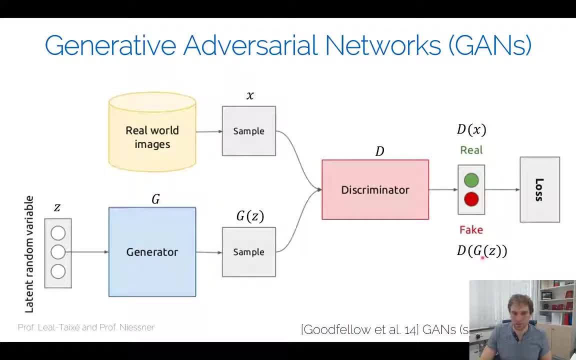 and d, g of z is the discriminator is now evaluating the generated sample and hope: well, hopefully, we'll discriminate. it's going to say it's a fake image, right, Okay and yeah, if you're looking at these two things, we have real data on one hand side and fake data on the other. 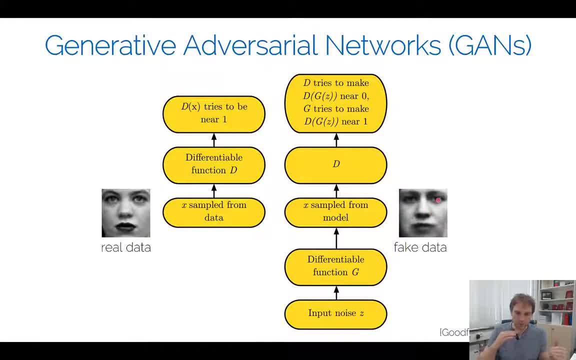 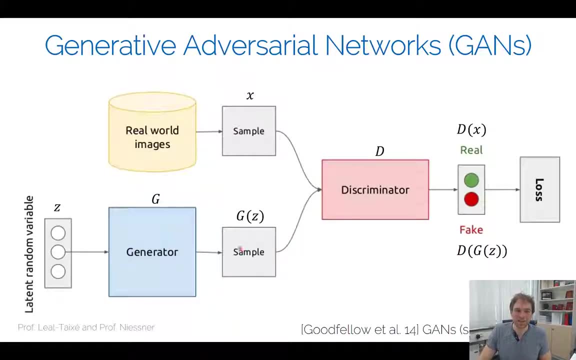 and the idea is: but by this- you know competing process, but this adversarial process, here we eventually getting good fake images, we eventually getting good images that the generator can do, and the idea is that this then lies essentially what we're hoping that we can. this is a certain distribution of real images. we hope that the generator will also. 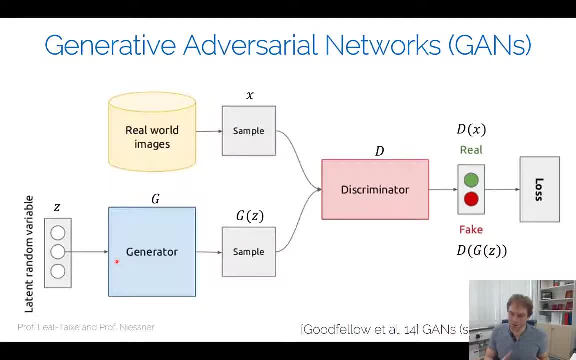 generate certain images that lie inside of the distribution. That's also why we call it an implicit distribution. what we're learning here- because we hope that we are not going to be able to avoid it in the future- have no explicit loss to match the distribution. here We're just hoping by training the generator. 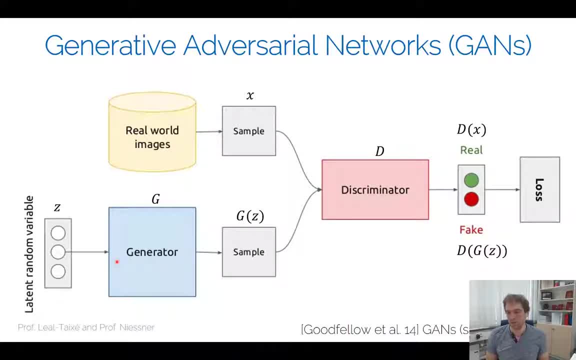 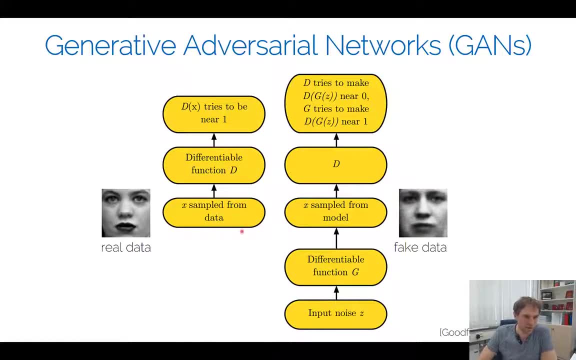 and discriminator at the same time. we hope that we're learning this distribution implicitly, Okay, yeah, but if you're looking at the two discriminator and generator processes, if you're taking a real sample here, right, we're putting a real sample here as input to our 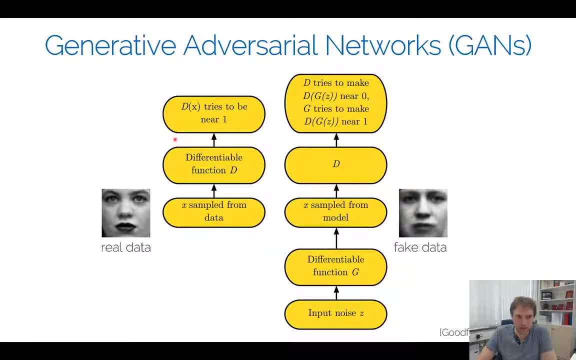 discriminator d and d of x tries to be near one right. it tries to say, hey, this is a real image. I try to recognize that this one is a real image. For the fake images, I'm going to start with some. 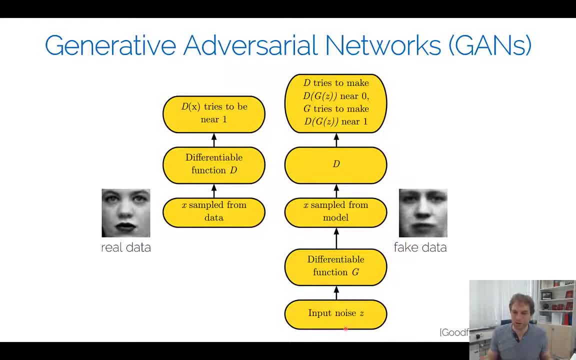 random noise. and out of this random noise, random variable, random latent code, I would like to generate an image, and this is what my generator g is doing, So it generates an image which is it's a sample from our model. 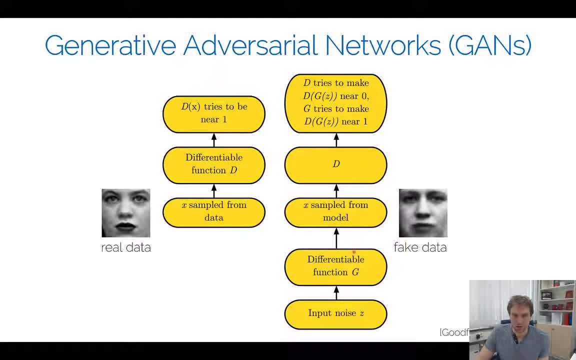 right This one. we're feeding it into our discriminator. and the discriminator tries to make sure that d of the generated sample is near zero and g tries to make sure that this one gets near one. right This one. the generator tries to make sure- oh, I'm fooling my discriminator, I'm. 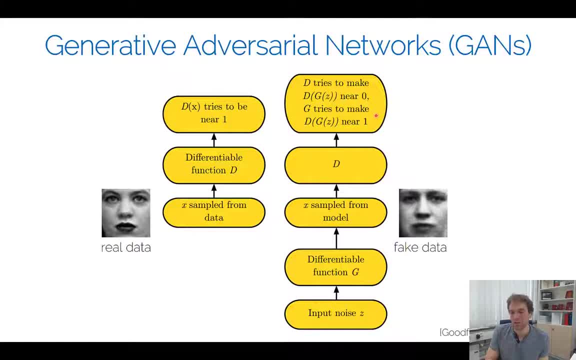 trying to make sure that I can generate something, but you can't tell apart anymore from the real world, And the discriminator tries to make sure. I'm going to nail you down, I'm going to know which one is real and which one is fake. right, And these two things run in parallel, right? so I'm 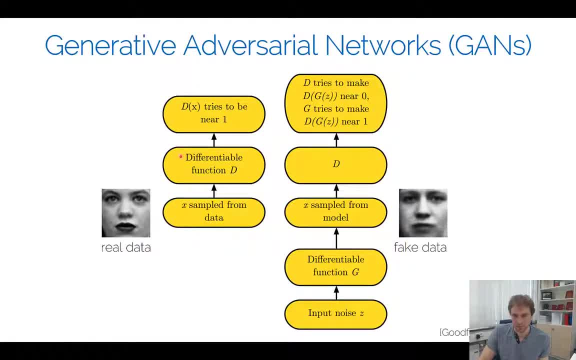 going to feed in real images, train the discriminator, and I'm going to feed in random noise variables to train both discriminator and generator at the same time. Now, if you're looking at the loss functions, we have here a discriminator loss and we have a generator loss. 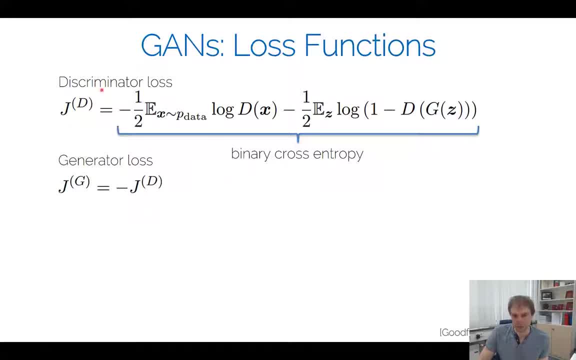 If you're talking about the discriminator- I mentioned this before- this is nothing else but a binary cross entropy loss, right? So if we are feeding in, so in this case we're having here the real samples x, right, this is our positive label, this is our one label, and then we have 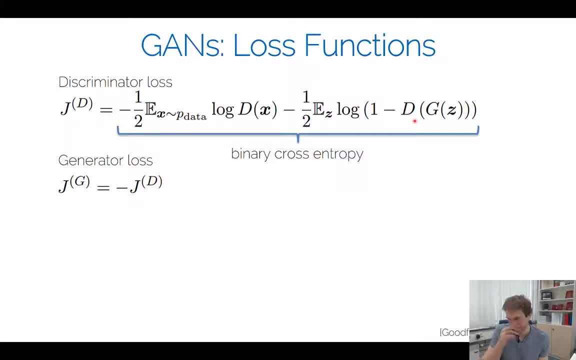 here our generated sample. this is our negative label where the discriminator should say: oh, this one should be wrong, right, this one should be one and this one should be zero. And the generator is just trying to fool the discriminator. 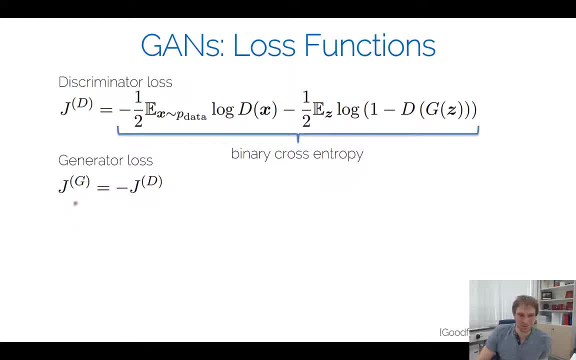 Right, we're just going to go ahead and say, oh yeah, just please, please, maximize the loss, basically, of the discriminator, right? Okay, and we're optimizing for these two things at the same time. So we're playing a little game, we're having this minimax game, So 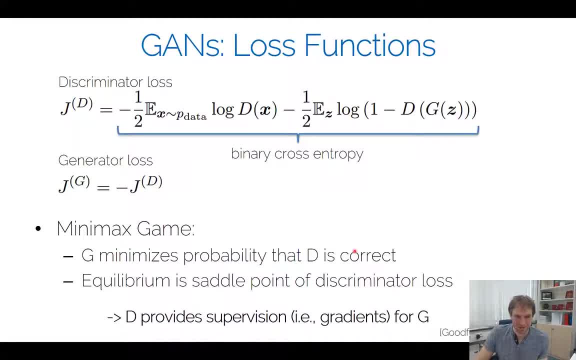 g minimizes the probability that d is correct. right, we want to make sure that our here, our generator, tries to fool the discriminator and a equilibrium is essentially the saddle point. right, There's no convergence in this case, like there's nothing, like it says: oh now I fooled the discriminator, but then I can train. 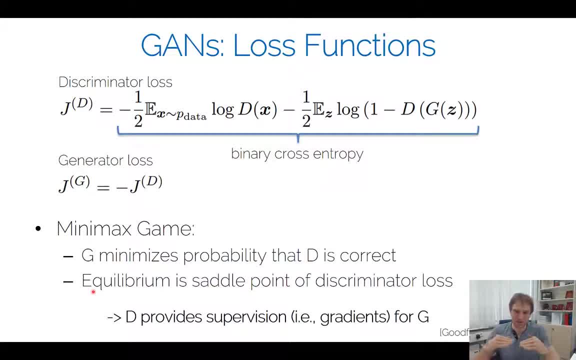 the discriminator again and it's going to say, oh, now I know it again. And these two things they mutually get better by helping each other to get better. And I mentioned this motivation before, where we're saying, oh, we have kind of this learnable loss function. 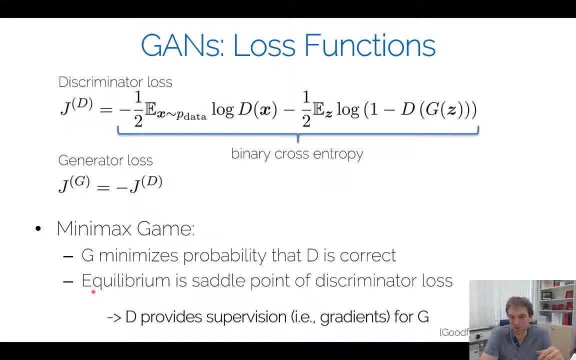 that what d is. d is essentially a learnable loss function, if you will want to say it so, and d then provides the loss function, or this learnable loss function. this discriminator provides the supervision for g, because we're training these at the same time. 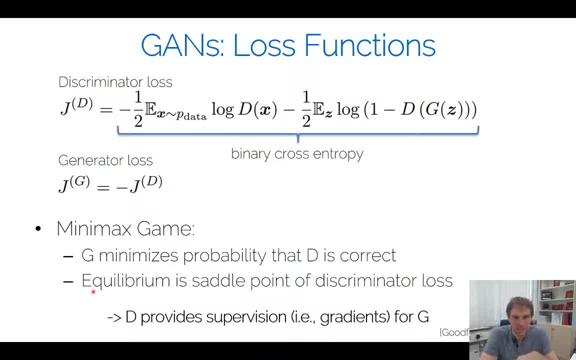 and because of that, we're getting- yeah, we're getting- the supervision for the generator. Now, one thing: what people have noticed: this was the very first formulation of the GANs here that Goodfellow provided in this very popular 2014 paper. 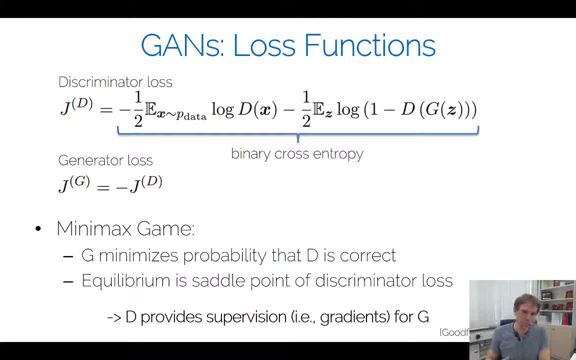 this idea of like subtle points and equilibriums is not necessarily something that was introduced in the GAN papers, but for this specific context it was, And the idea now is basically that we're having this discriminator here. One problem: what might happen is that the generator here 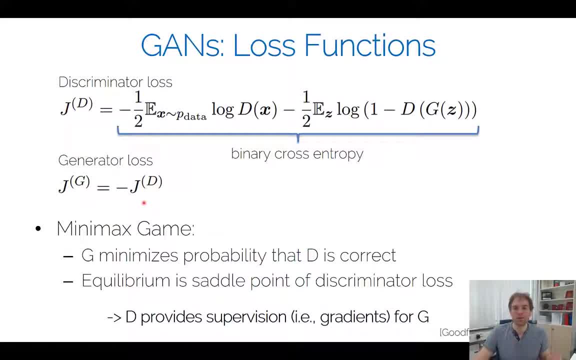 yeah, this might be still a bit of a problem because the generator might always be wrong, right? So, basically, if you're never going to get a good, a good real sample- sorry, a good fake sample- generated, then this loss from the generator will always be high. 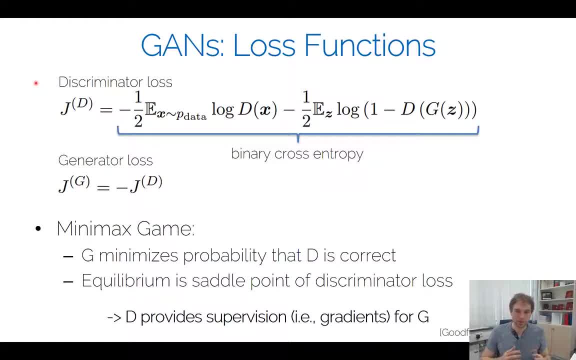 and this loss will always be low. And you? the problem is there's no like smooth function. basically, that tells the generator how to get better, And oftentimes what people do is, instead of having this like just the negative discriminator, what people do is. 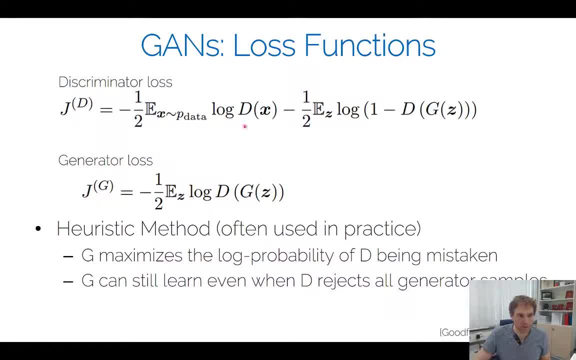 they use this heuristic method. If I'm going back, this one is still a binary cross entropy for the discriminator but for the generator. now we have the negative log likelihood that the discriminator of the generator is right, right Of the generated images is right, right. 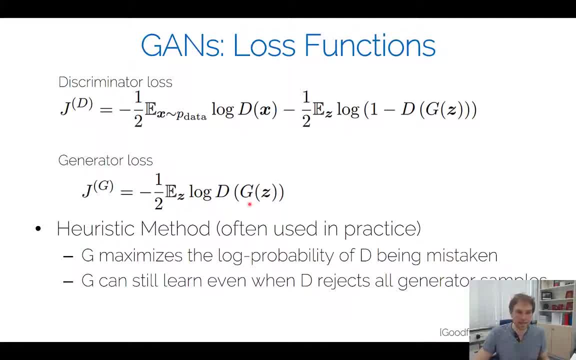 And this is a little bit different. In this case, we maximize the log probability of D being mistaken instead of just taking the negative loss function of both. The idea behind this heuristic method is that G can still learn even when the discriminator checks all the samples right. 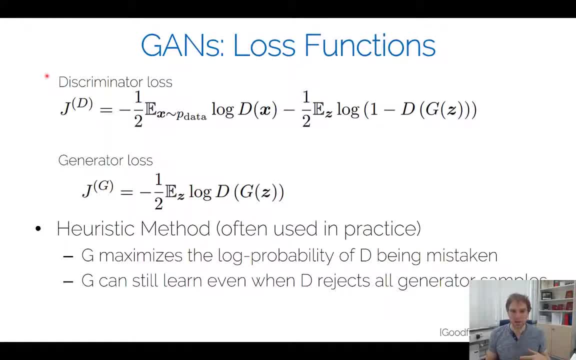 And that's often the case because, principally, we're going to have this issue- that generation is a lot harder than discrimination. If I have one wrong pixel, in principle I know it's a fake image. I mean, it's not so easy. 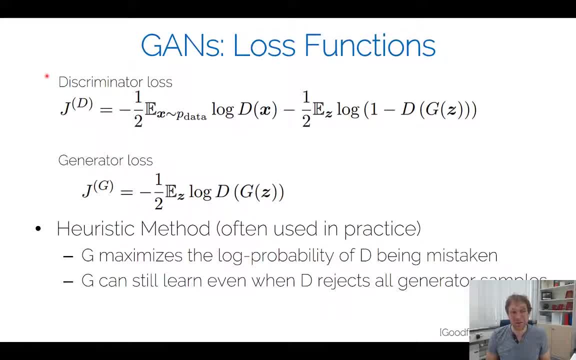 it has to still learn it, but generation is, in principle, harder than discrimination. Sorry, discrimination is easier than generation, And this one is why we have typically this negative log likelihood. And I can already say like: this is the standard Gantt formulation: 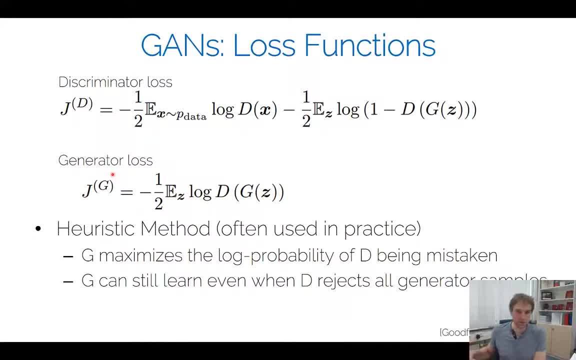 that most people use today. Again, we're going to go into a lot of different formulations later, but this is one of the formulations that a lot of people are using. Yeah, so the idea is that G can still learn even when D rejects all samples. 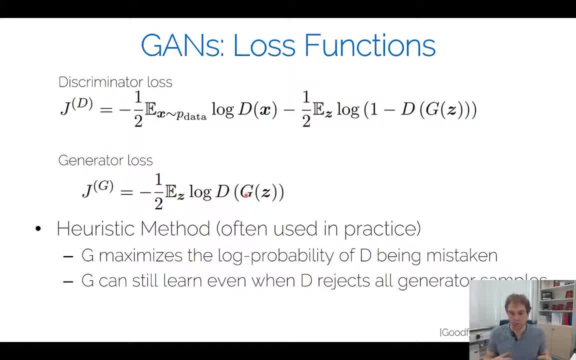 because this log loss will not be like so extreme. There's a log likelihood that makes it easier. Okay, in practice, when you're training this, you just have both losses right And you just train them at the same time. Now, if you do this, as I already mentioned, 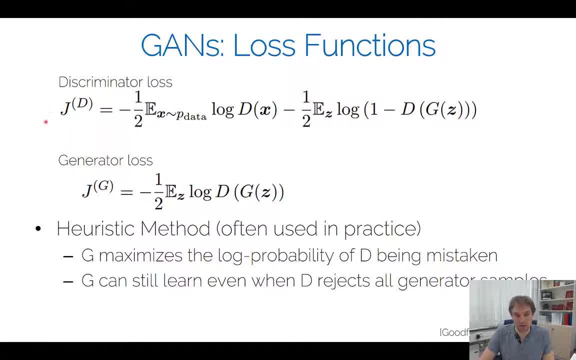 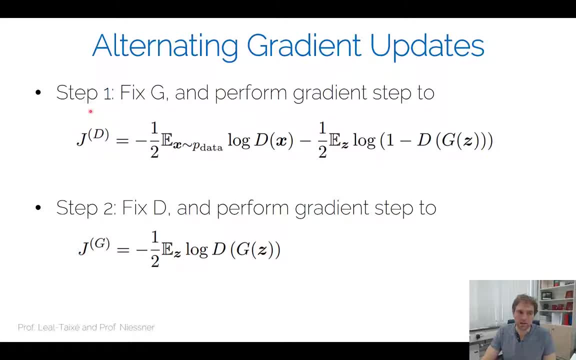 what often happens is the discriminator will just always dominate the generator and often you do an alternating gradient update, meaning that you fix the generator, you do an update to the discriminator. So you only train the discriminator for one step, And the next step would be: now we're fixing the discriminator and we're performing one gradient. 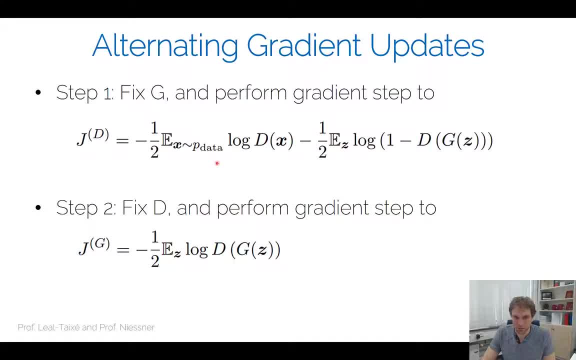 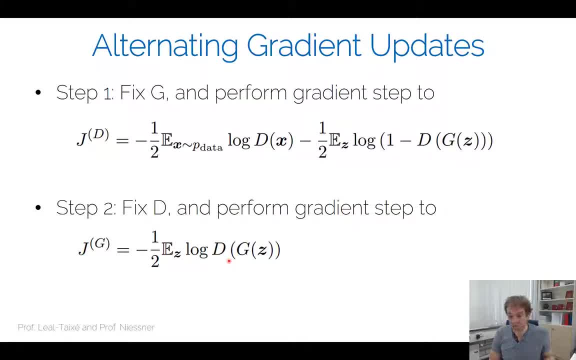 other thing is that basically we only have gradients for half of the network, So we either need to train generator or discriminator. We can have bigger networks. That's one advantage, But it's also a little bit more stable because you don't have so many unknowns. you're training. 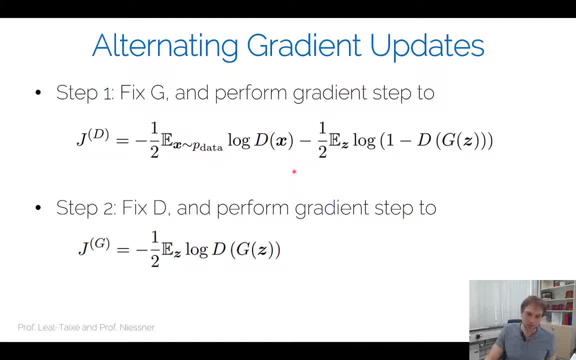 at the same time. So often this alternating update has been being used. I'm saying has because nowadays, I think, people mostly train it actually jointly. They figure out how to stabilize it with various tricks, right. But one thing you can do in this alternating update steps: 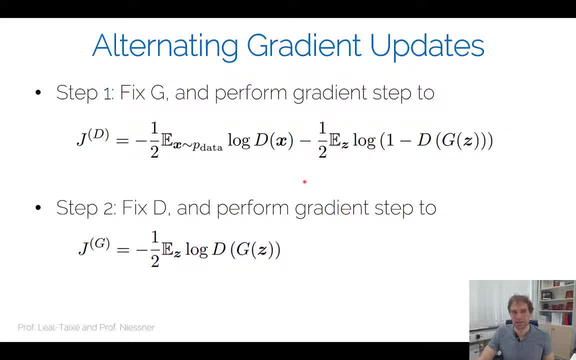 is well. if my discriminator is too strong, I can simply train my generator. here I can train the generator more often, So I can do one step here. I can, let's say, five steps here, one step, five steps, one step, five steps, Or I can also do it adaptively. I can check the. 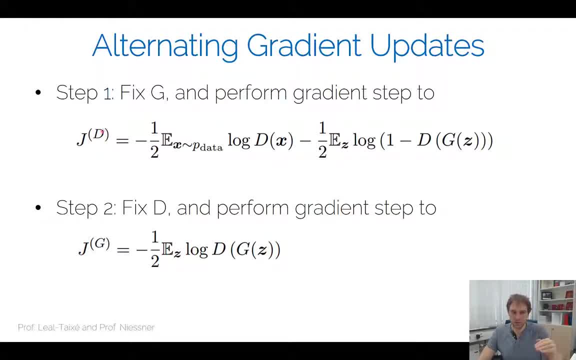 loss function until my discriminator loss goes down to a certain level. I'm gonna do these updates Now. I fooled the generator. Now I'm gonna go ahead and go to the generator again. I'm gonna generator until my generator loss goes down and this way you can balance the. 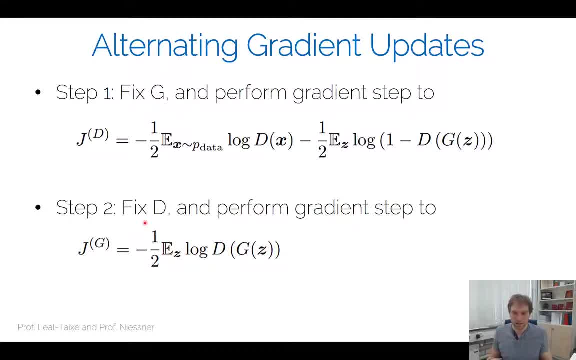 two losses, so you don't. you don't collapse, and I'm mentioning this collapse word now a couple of times. collapsing means typically when the generator is always wrong and the discriminator is always right, which is a problem. when you don't generate anything, you basically have a teacher that tells: 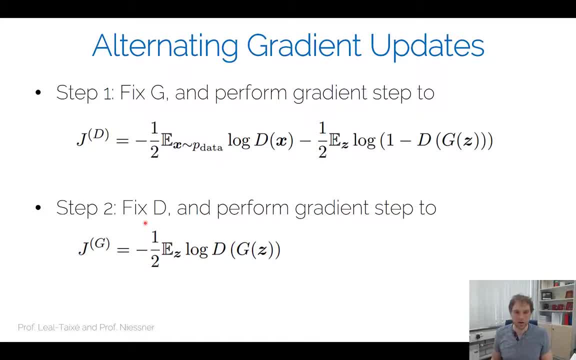 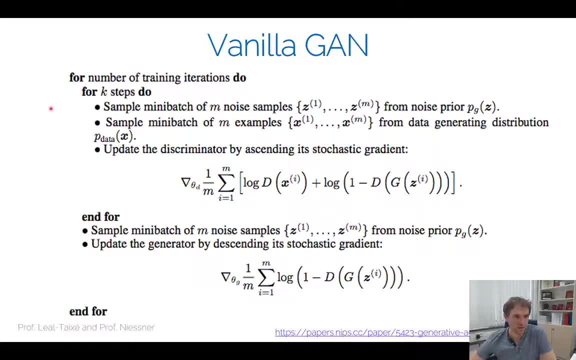 you whatever you're doing is wrong, but it doesn't tell you how. okay. so this is this vanilla again. so what you do is write for number of training iterations. what you do? you sample a mini batch of M noise samples. this is all latent code. so we have our random variable Z. we sample our, our real images X from the 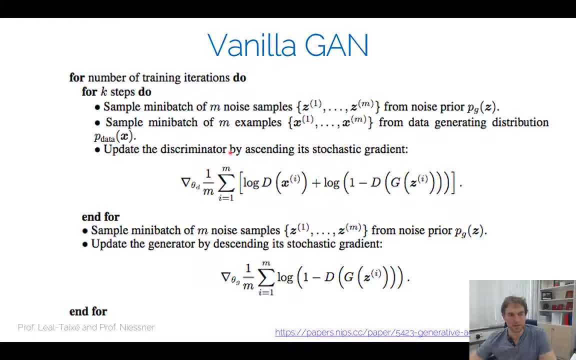 training data. and then what we do is we update the discriminator a couple of times, right, and in. in this case, we have this K loop here that goes over this one here, right, and what we do is we simply train, in this case, the binary cross entropy loss. 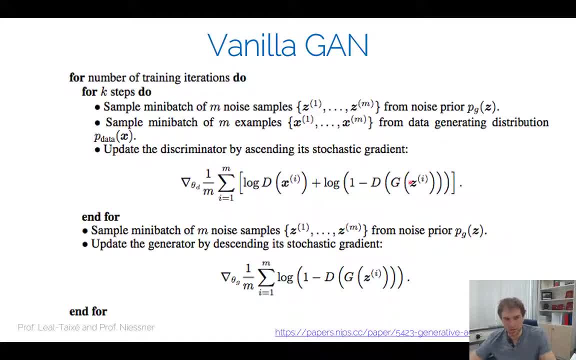 of the discriminator. now you can argue that you're still updating both weights here. you could also say, oh, I'm only going to update the discriminator weights. that's what I'm saying. like sometimes you can split this apart, depending on how it goes. the second part, then, is here. now you sample the mini batch of the. 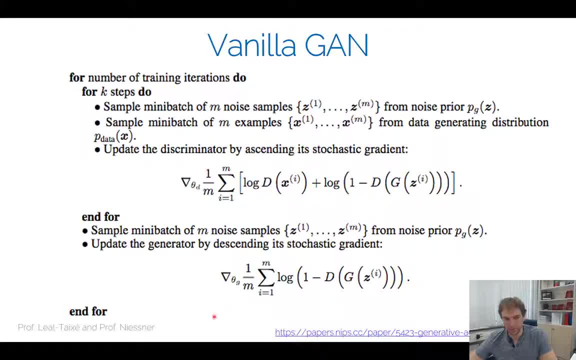 noise samples and then you're only training the generator part. in this case. here we actually training the discriminator a couple of times we only train the generator once. yeah, I should say this might not always be a good idea. it depends a little bit on how these noise functions behave, how these 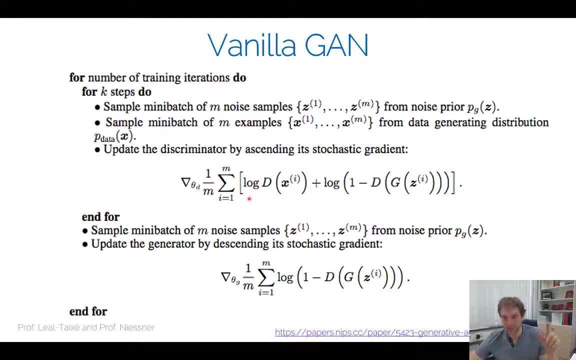 training functions behave. you can see in the losses if your training loss goes well. involved in this case means if my discriminator goes to zero, I'm pretty I did something wrong. a very good debugging stand at the beginning of training again is train this function and check that it goes down to zero if 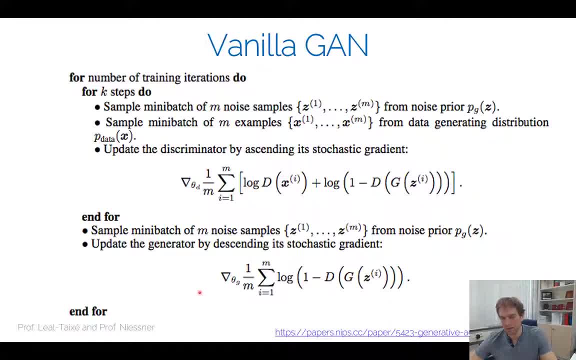 you, if the discriminator can go down to zero without training the generator, then something must be fishy. that's just a simple debug step, because we will see training is again bad. this is actually very, very tricky, okay, but anyway, what I'm trying to say is in: 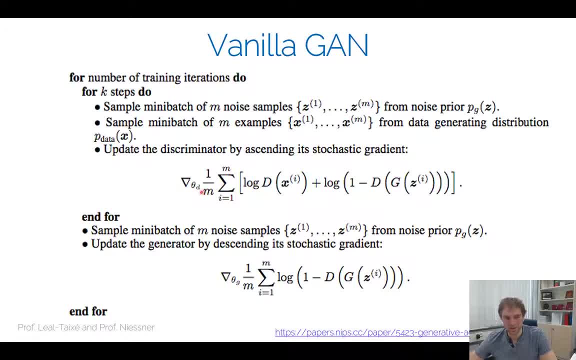 the vanilla GAN version. you can. you can decide, like there's various versions, how to how to alternate between these things. and typically what people do is they look at the loss functions they want to like in the training schedule to check already, like how, how strong are my updates? okay, if you're looking at a 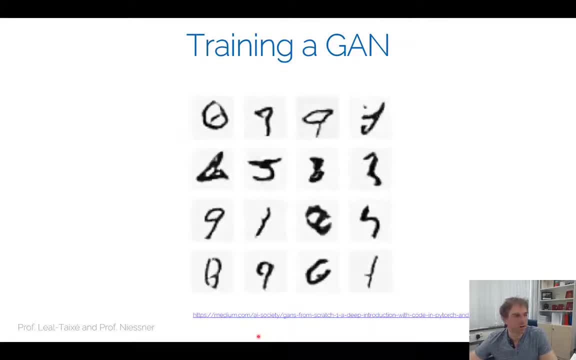 training process. it looks something like this: this train on MNIST, so we hopefully generate some real numbers for MNIST. this problem is relatively easy, right, meaning that we have a small data set right and hopefully after, after a couple of minimax games, we hopefully can we. 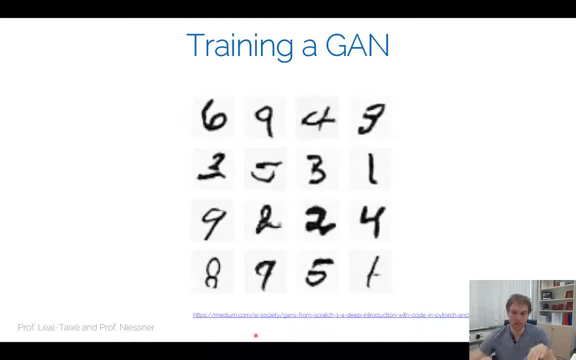 hopefully get something reasonable again. we're not converging here. we are still in this equilibrium state where the generator and the discriminator- they balance each other out. yeah, let's have a look at the loss curves, and that is actually something that is very interesting in this. oh, yeah, one thing I should say here, like whenever you're visualizing: 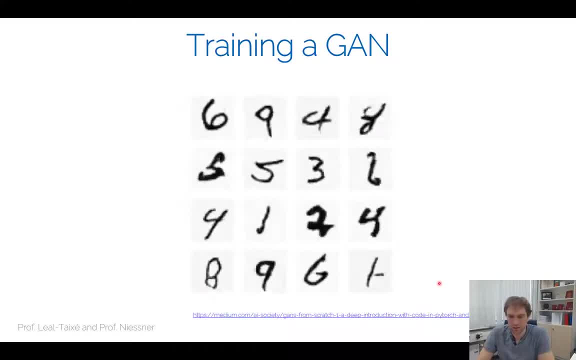 the GANs. what you do is like in your tensor board framework, for instance. what you're going to do is you have this: one is a fixed latency, so you have a couple of fixed random vectors where you want to want to display stuff and for every iteration you're displaying always the same random variable here same. 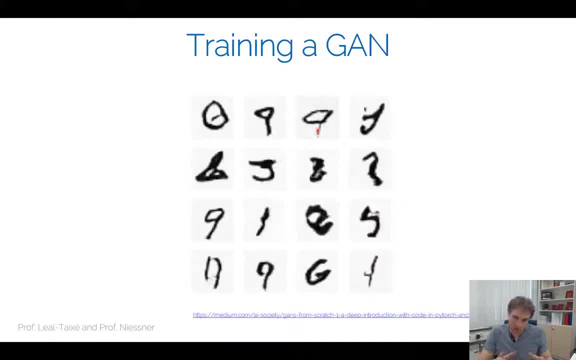 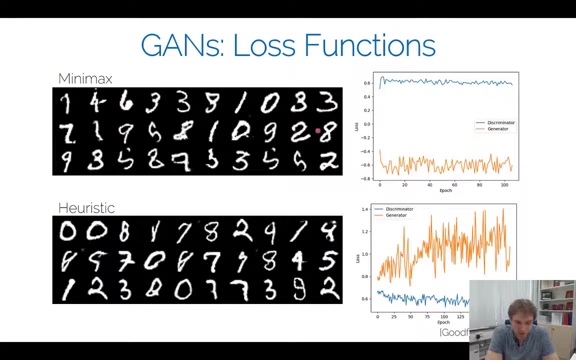 random variable here, same random variable here, so they will chitter around based on the training progress. but in principle we should get sharper and sharper results and ideally, in this case, you should see the visual appearance of these numbers. okay, and one thing that is very important: I'm looking at the loss. 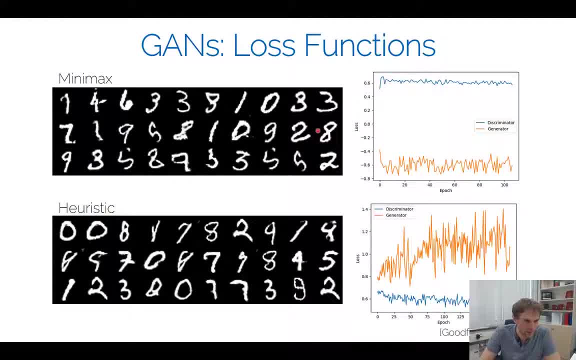 functions. we see here two examples. we see a standard minimax game. we see a heuristic method. again practice. most people use heuristic methods today. training losses should look something like that or can look something like that: right, you have here. ignore the loss curves here right now and 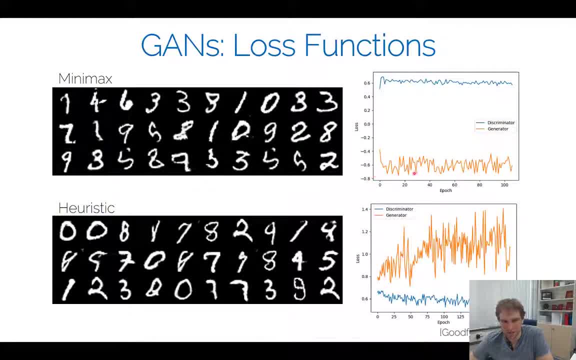 this depends, of course, how you, how you display it. but I mean, if the generator is like, like, if you're going back to the loss function here, this is just the plane loss in this case and this is just negative discriminator. that's why this loss is negative here. but um, let's ignore that for now. basically, like in: 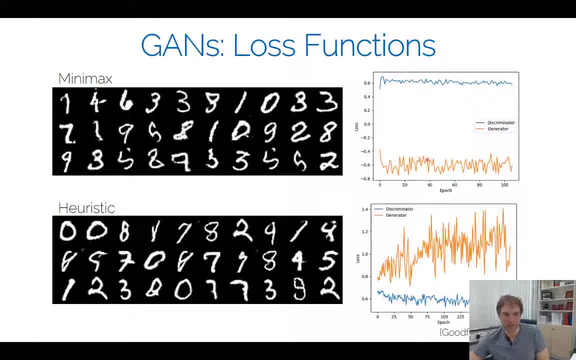 this case, the generator would- would like to go up here, right, sorry, generator would like to go down here and this guy would like to go down here, okay, but um, what we see in this training process is that we see a relatively stable training, right, so these two losses, they don't change. 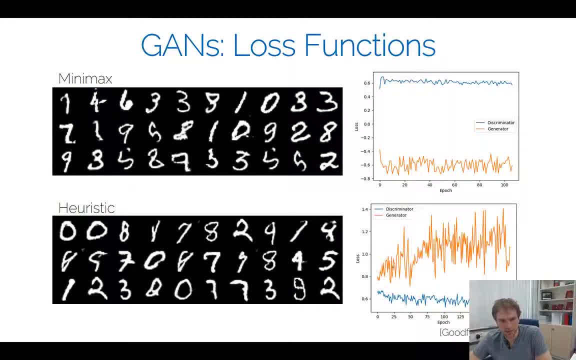 too much. and even in this case here, of the heuristic methods, well, yeah, they go a little bit apart, but they don't, they don't fully go apart. right, a little bit, yes, but not not too much. and after a few iterations, and you would expect that they they're relatively stable. this is an interesting thing. so now the problem. 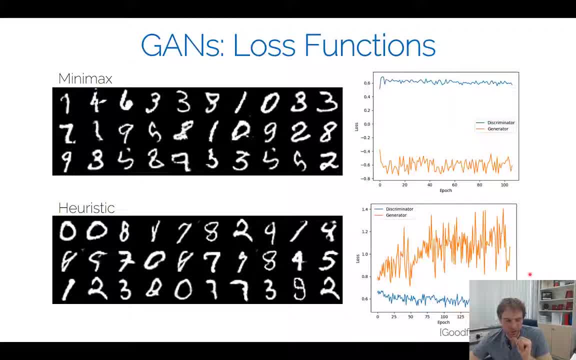 is when you're looking at the loss curves. I don't know when I'm converged right. I have no clue. like this, loss function doesn't tell me um how far am I my training process yet, or how good is the quality of my generated samples yet. um, a good learning, a good training curve for again, is that. 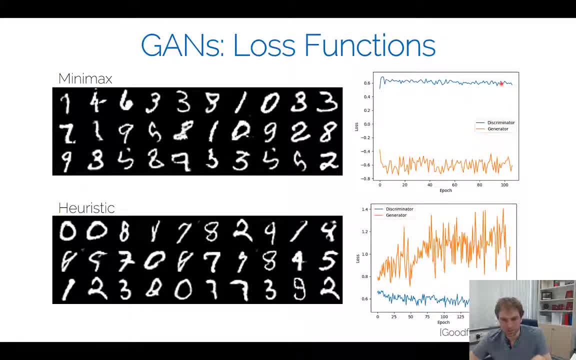 it's relatively stable. I will go into second, also about bad learning curves. um sorry, best training curves and bad training curves would be that if this discriminator here goes to zero, it's still at 0.6 here. if this one went down to zero, then you have a problem because that would mean that we are collapsed. 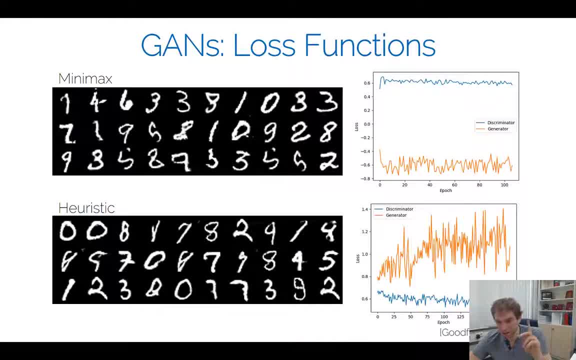 and the discriminator is always right. that's an issue, um. I should say also one thing: whenever the discriminator collapses to zero, there's no recovery. once this happens, then you can restart your training like, um. this often happens already, at the very beginning, which is in a sense good news for you. you don't have to wait two days, you know. 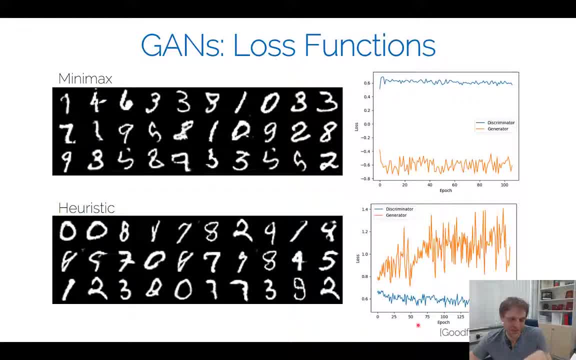 immediately when, um, when you collapsed, and then you can already go ahead and reach, uh, change some parameters, fix your box and so on, and restart the process. um, yeah, this is typically how these losses look like. these are some generated samples. um, I mean, on MNIST, everything looks kind of okay, so there's no big difference between. 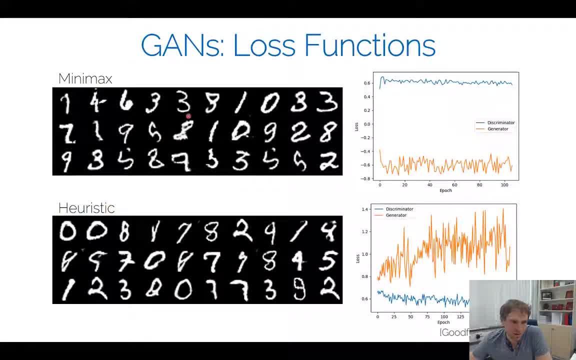 minimax and heuristics. you could argue: this one looks a little bit broken here, this one looks a bit broken. yeah, they look similar. I guess there's not so much of a difference here. okay, these are very simple loss functions right now for the game that we use. so we 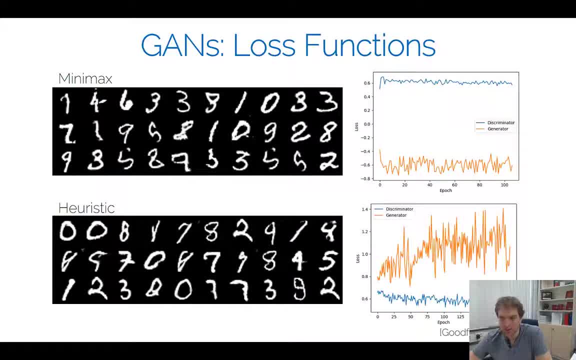 have a generate and discriminator loss right. we're trying to optimize them jointly, either with alternating or with joint training, and so on. now, what we want to do now is, of course, we want to generate something that is a bit more interesting than MNIST images, but we want to go. 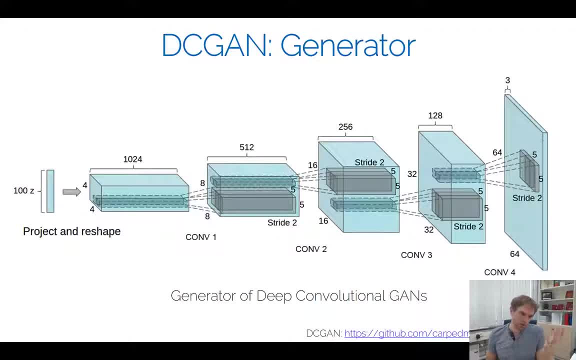 to real images. um, and there was this. well, one of the first architectures here and that people have proposed was a convolutional architecture. it's this DC GAN paper, deep convolutional GAN paper. the idea is we're starting with a hundred dimensional latent code Z. we're reshaping. 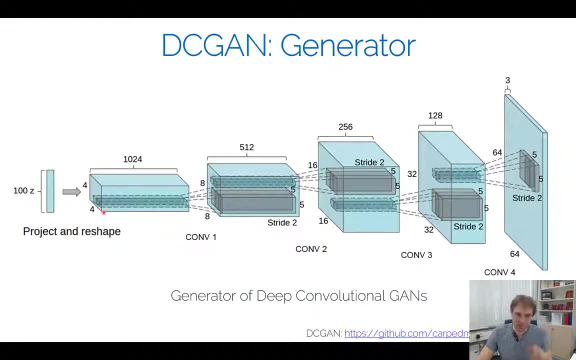 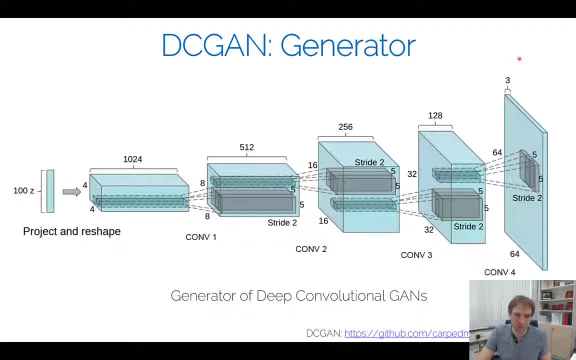 right until we have a feature dimension of three for RGB for our image, um, and we're gonna make our spatial size bigger from four to four to eight by eight to 16 times 16, 13, 2 times 32 and 64 times 64.. so this generator here generates 64 uh squared images and 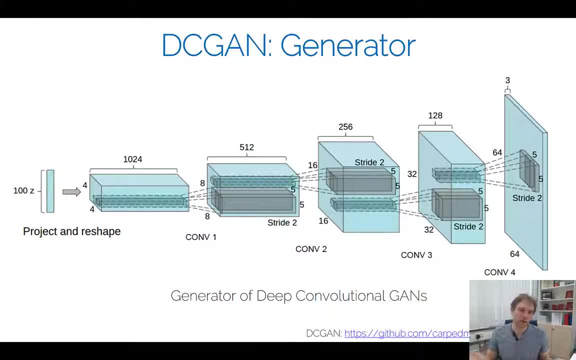 we can apply this to all kinds of data. so this again is one of the first architectures people have have used there and it's still being used today, so it's a reasonable architecture, right? it's basically? well, what are you doing? you're starting with a random vector, right? you're? 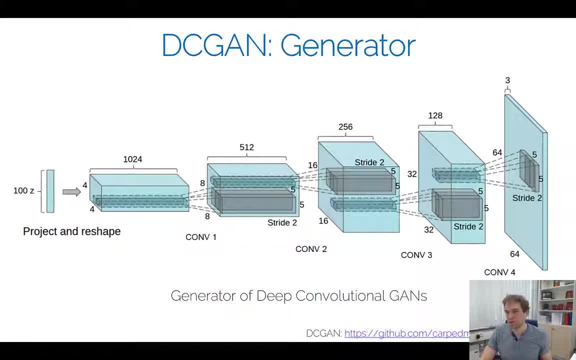 reshaping it, um, to a four by four feature map, and then you're doing deconvolutions until you end up with, um, your desired image size. um, oh yeah, by the way, the bigger the image size, the harder this gets right. um, in order to get a big image coherently generated, you have to do a lot of things right with. 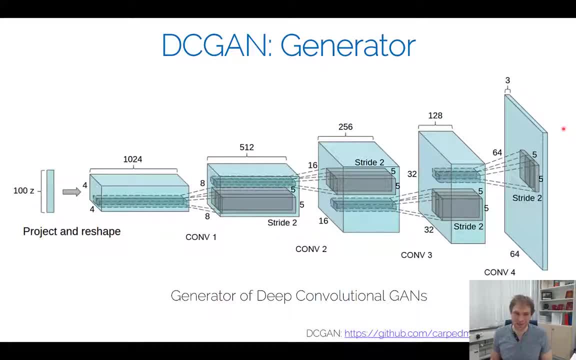 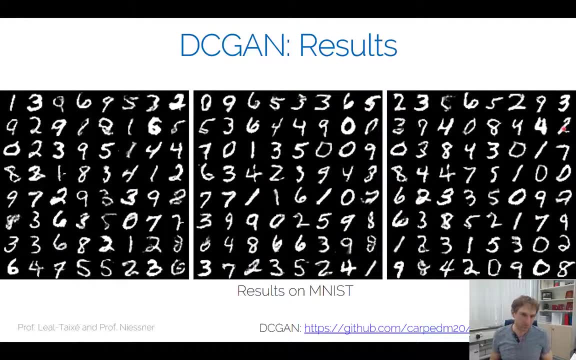 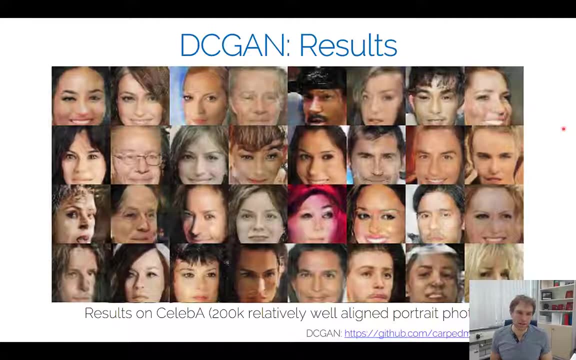 the generator, and we will see that later- how difficult it is to generate, um, yeah, bigger images, okay. um, yeah, here are some results on MNIST. um, again, looks pretty reasonable. um, here are some results on Celeb A. Celeb A is one of the data sets you will probably use a couple of times in. 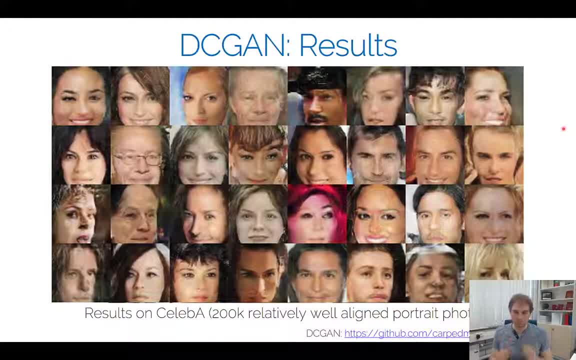 the context of GANs. these are basically portrait photos of human faces. where the face is relatively centered, it looks relatively straightforward, which makes the problem somewhat more tractable. right, basically, since we are trying to implicit, learn, implicit distribution here. if the distribution is smaller, the problem. 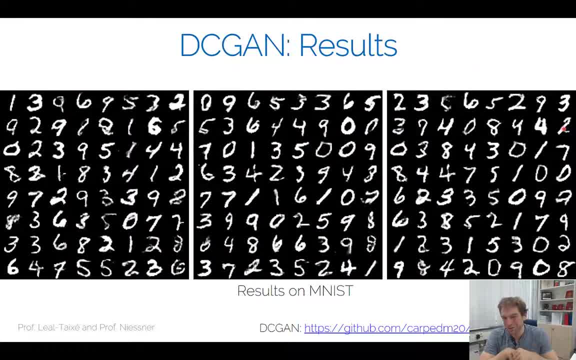 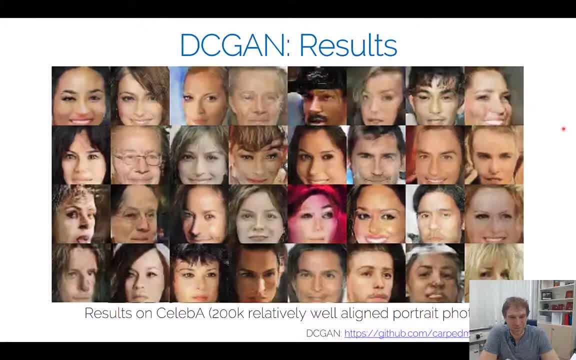 becomes a lot, a lot easier, right, and if I'm taking like this problem here for MNIST, my distribution of these bunch of like MNIST numbers is is pretty straightforward, so of course it's an easy problem. yeah, faces are more complicated, but the problem is here for Celeb A, it's a bit relaxed. 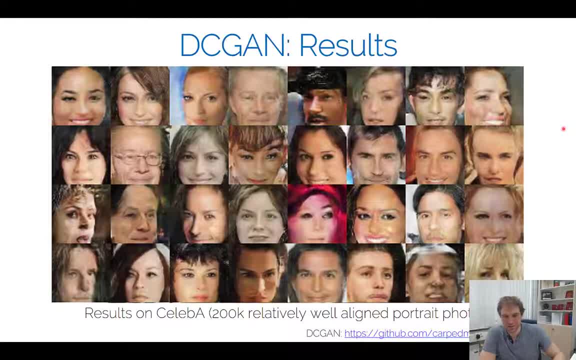 because they're all centered right and there's all sorts of biases. I'm not, I'm not gonna, I'm not going to go into too much detail here, but there's not, it's not a realistic representation of the human population here. right, these are celebrities. um, uh, that's what's a cel data set, um, and and. 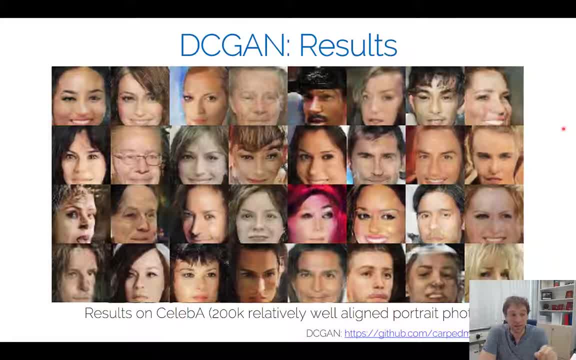 they are relatively small. distribution of people, basically okay. bottom line, though, is: this is a good data set to start training against, because it's a bit easier. um, and in this case we have right. In this case, these are the results that you're getting with DCGAN. Yeah, looks okay. 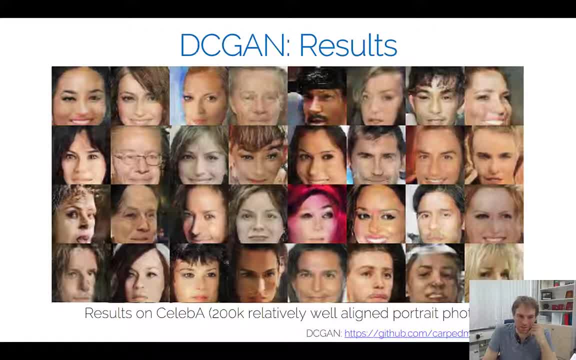 right, It's not too bad. We're getting some faces. They look okay. They're not perfect, But you can see already now we're getting to somewhat reasonably sized images. right, It's not like just simple MNIST numbers anymore. We can do something with faces. Here's another result on 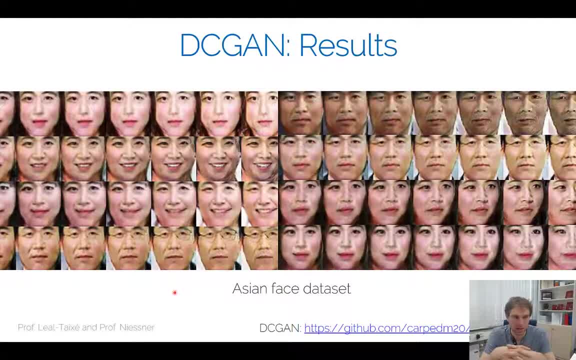 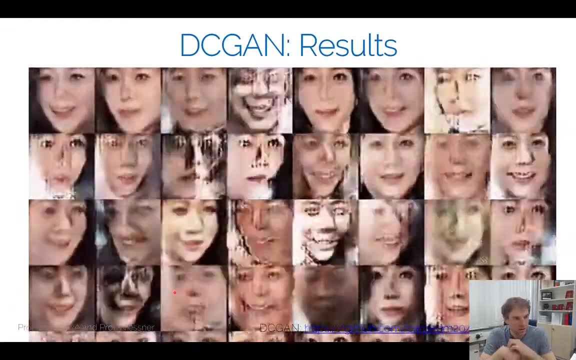 the Asian face data set. Again we get reasonably reasonable faces. Again, I would like to highlight it's also a relatively easy data set. Again, portray mainly face center makes it a lot easier for the network. Here is an example: when you sample through the latent codes, This is: 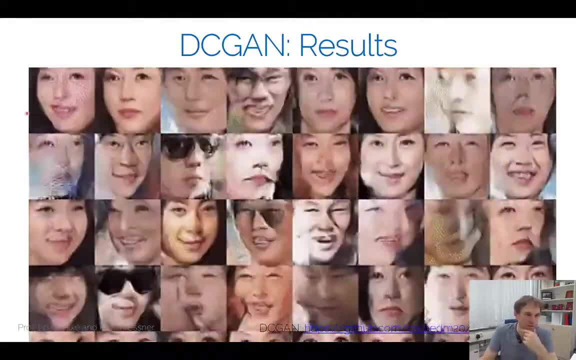 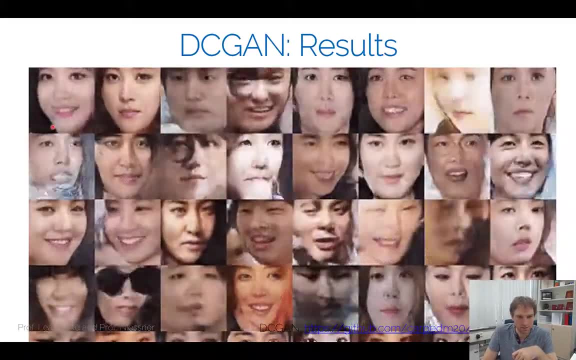 oh, no, sorry, this is actually the training process. I think this is basically. it starts here. It starts blurring- This is always the same latent code- and then, in theory, it gets sharper and sharper. Yeah, again same problem. We don't know when we're converged. All we can do, basically: 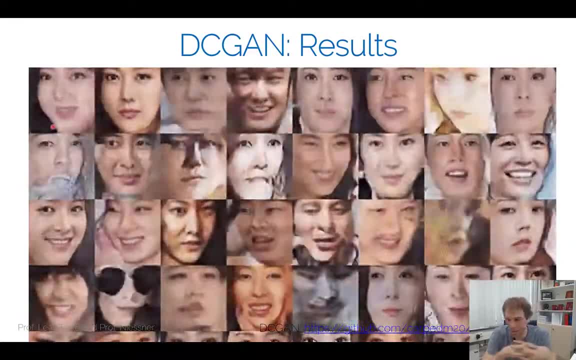 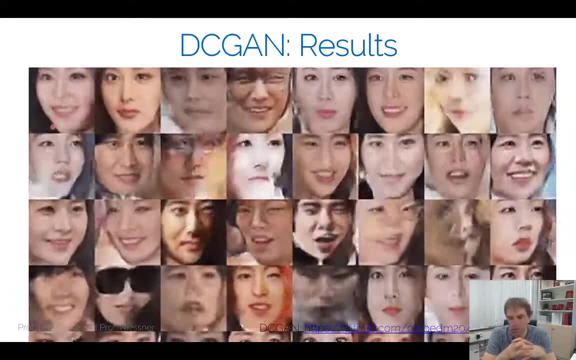 for debugging is be looking at these generated images. Yeah, I wanted to talk a little bit about that one right now. I wanted to talk about how do we know this stuff is working or not working and what do we do if it doesn't work. 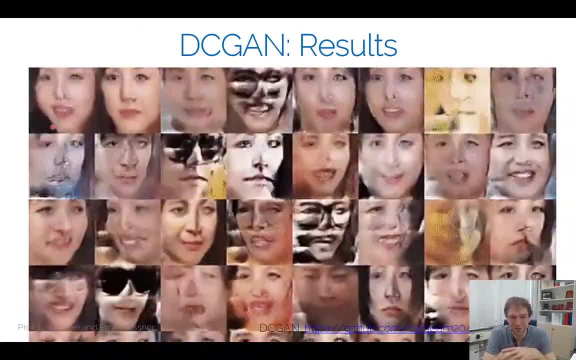 And I can tell you a fair warning at the beginning, when you're trying this out, a lot of things won't work because it's very tricky to pick up. It's very tricky to pick up. It's very tricky to pick up. It's very tricky to train these scans, And we'll get into this in a second why it's so tricky. 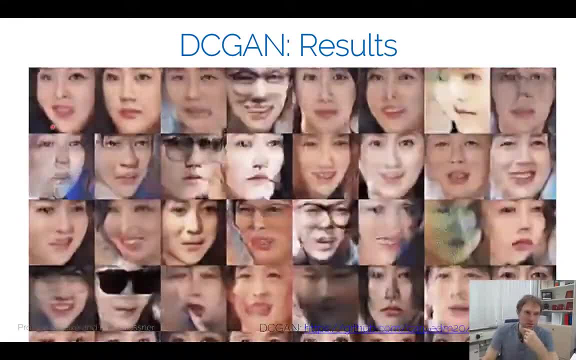 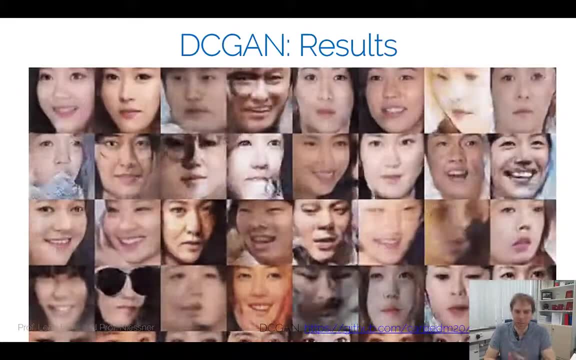 But let's look at the debugging steps, what we can do. Well, what we can do is: we can definitely do this here. We can again set up TensorBoard every any iterations. We just take a fixed number of latent sample codes, right, and we're looking up, always the same. 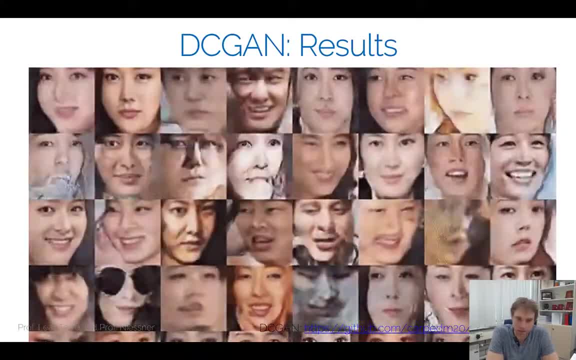 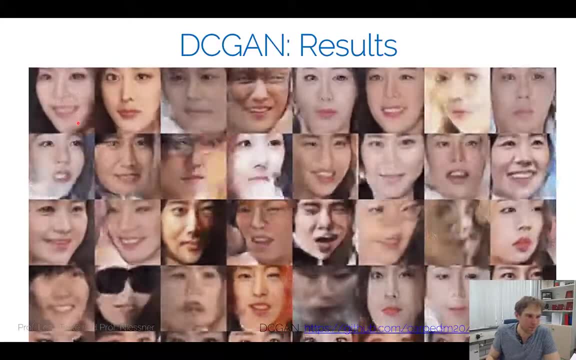 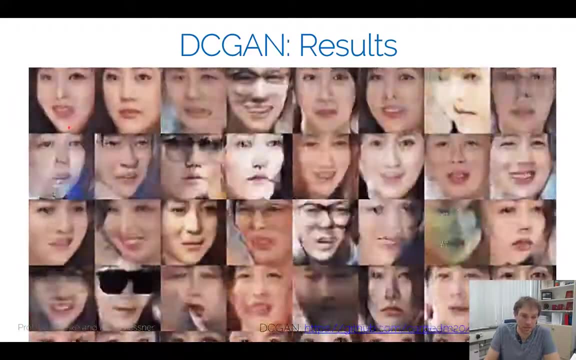 set of latent codes And ideally they're getting sharper and sharper and sharper, which I guess you can see here to some degree. But yeah, I guess this gif here starts at the very beginning. when it starts It's very blurry, and then it gets better and better. There's a few things we can. 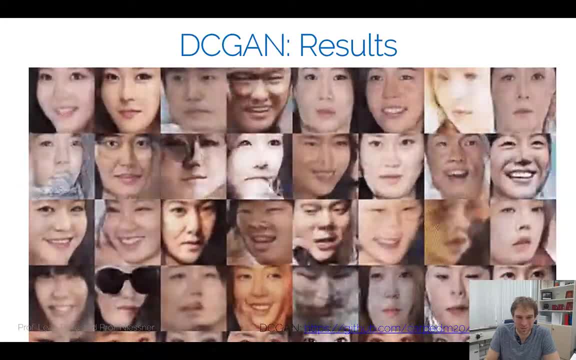 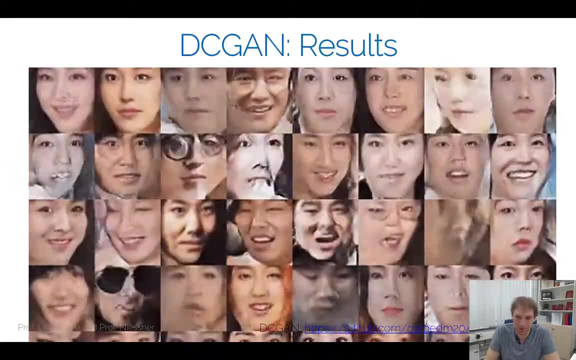 later talk about. One problem might be mode collapse. One problem might be that all of these ones look the same. eventually That's a problem. We'll talk a little bit about that one. That means, well, my generator generated one real image, but it's always the same image. That's also a bit of a 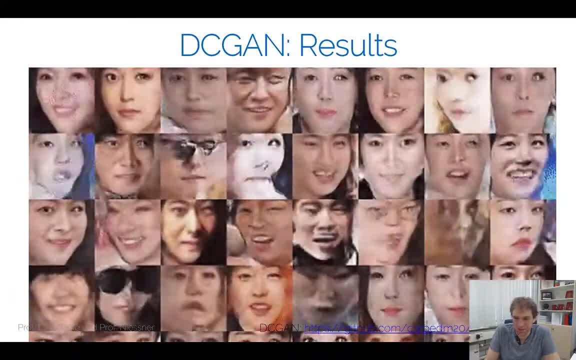 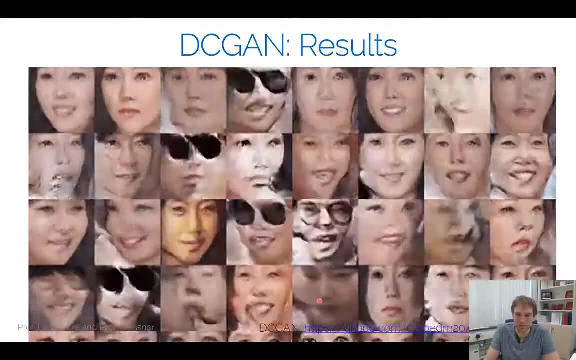 problem. Sometimes you can end up with a bunch of them. This is a common problem. you can see very quickly here: if you mode collapse- And if you mode collapse early on- I mentioned this- you can hardly recover from that during the train. We can look at the loss curves. Yeah, these are good loss. 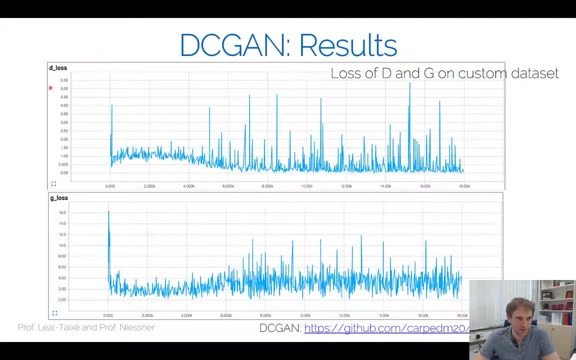 curves, by the way. Good loss curves meaning I have the discriminator loss here, We have the generator loss. It's a bit wild at the beginning, At the very beginning, right, it fluctuates a bit And then after a little bit, you know, this one goes a little bit down, This one goes a little bit up. 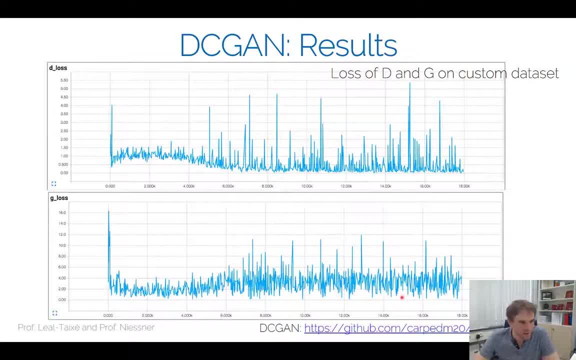 You know, they kind of stabilize here, Don't go to zero, none of them. They don't go well, There's a little bit of fluctuation, But in principle they're doing all fine. That is considered to be a good training curve, right? Because we don't have. we're kind of 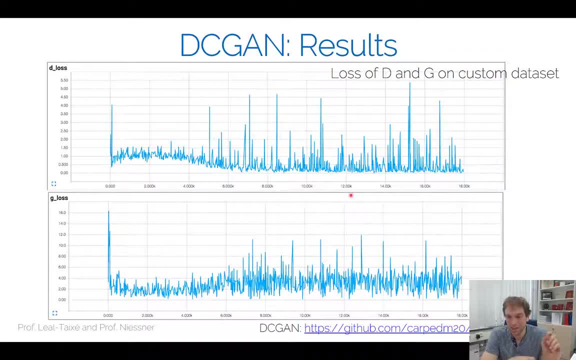 managing to hold this equilibrium, at least from a loss standpoint. That doesn't mean necessarily it works, But if the loss was not stable, then I know for sure it did not work. So it's one criterion you can do here to look at it. Yeah, when are we done here? We don't know. We can train for a long. 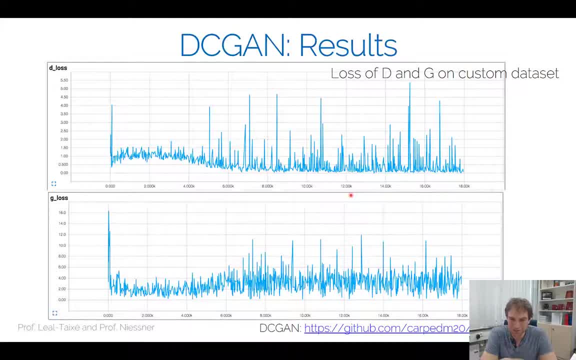 time. In principle, it's getting better and better And, assuming my model capacity is good enough and I have enough training data, my distribution should also get better. But I can tell you, oh, now I'm done with my training. right, For this one I have to go back, look at. 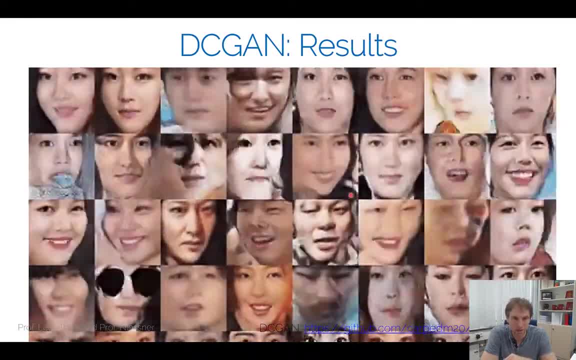 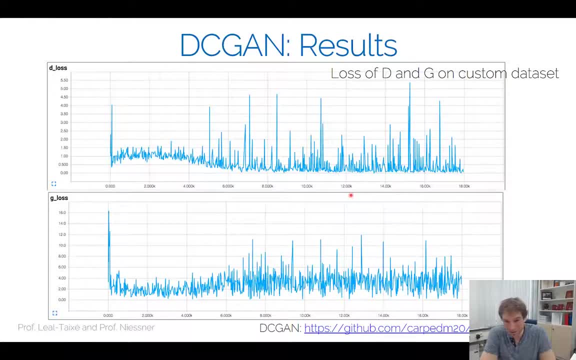 the images. I'll later go into a few details on how to evaluate. Is it a good image or not? Yeah, but I can already tell you it's difficult. Let me also show you some bad curves. Bad training curves would look like that. 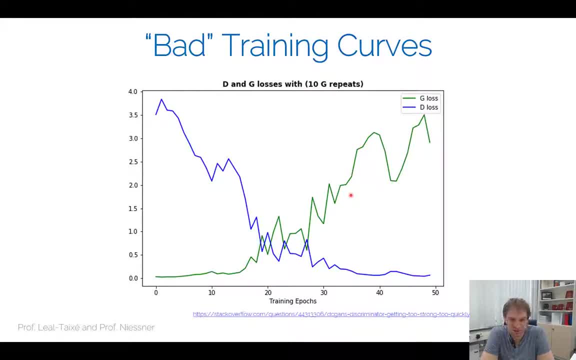 This is a canonical curve a lot of people will get when they try and GANs out the first time. What's going to happen is: this is our nice discriminator right. This is our again training epochs. And what happens? this one goes straight down to zero. This one goes up. It will. 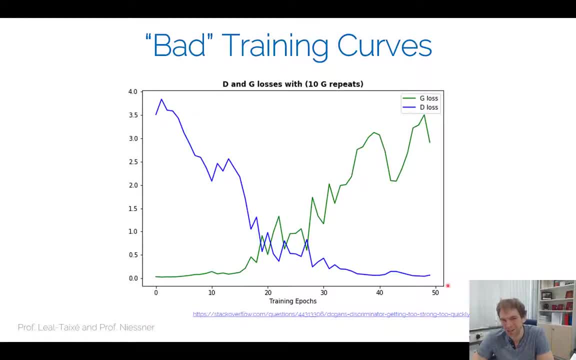 still stay here and go a little bit. There will be still a bit of fluctuation, But you can see this one collapsed, This one went to zero, This one went up. No recovery from here. Restart, fix your box, fix the training data, fix your schedule and stuff like that. In this case, something went. 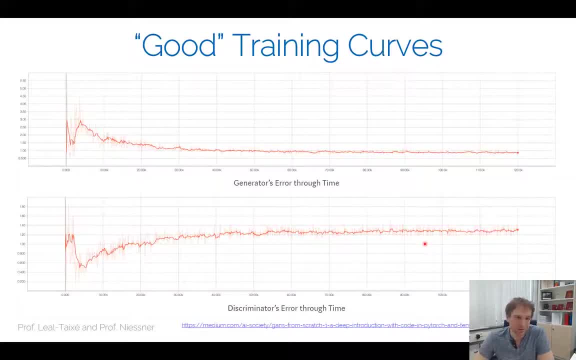 terribly wrong Again. good training curves look like that. I like showing them. They look pretty right. They start wild a little bit at the beginning, but eventually they're gonna balance each other out. This is what's considered to be a good curve Again. 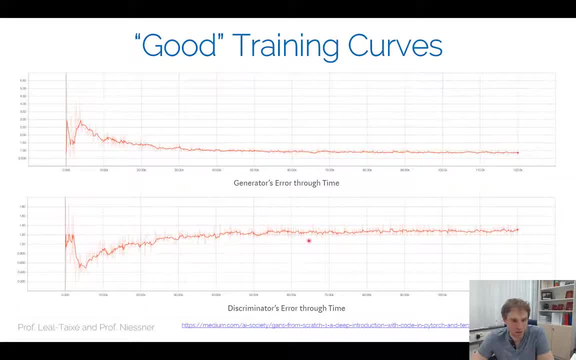 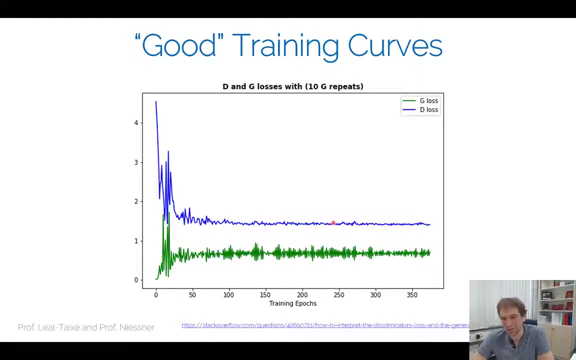 very important if you're looking at the discriminator. The discriminator should not go down to zero. If the discriminator goes down to zero, something went really, really wrong. Well, we have here another one. By the way, I just typed into Google: good training curves for GANs. Actually, no, I didn't. 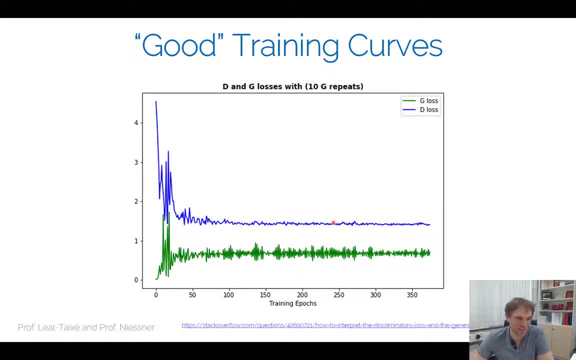 do that. I just typed in training curves for GANs and then I picked the good and the bad ones. Okay, again, good, one goes a little bit wild here, right, Discriminator stabilizes goes a little bit wild here. Generator also stabilizes. Again, very important that. 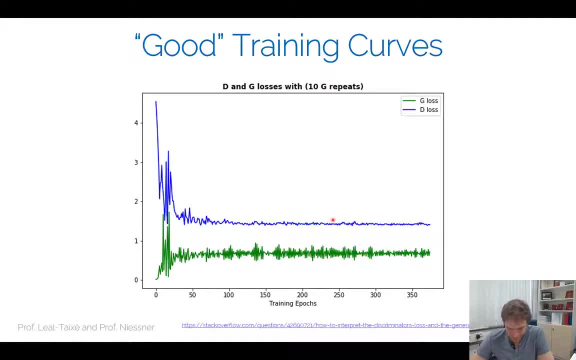 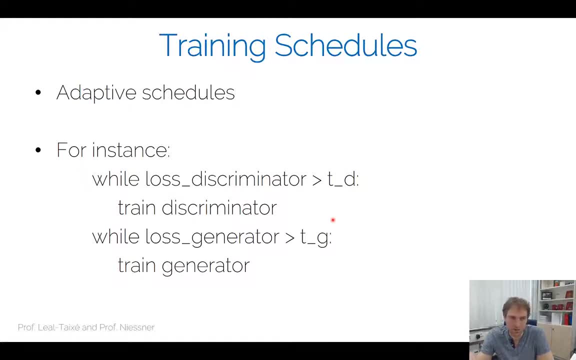 the stabilization happens. Okay, yeah, I mentioned the training schedules We've seen for discriminative networks. you need training schedules like how to adapt your learning and stuff like that. We have the same thing here Now. the problem is we have to adapt both of them. 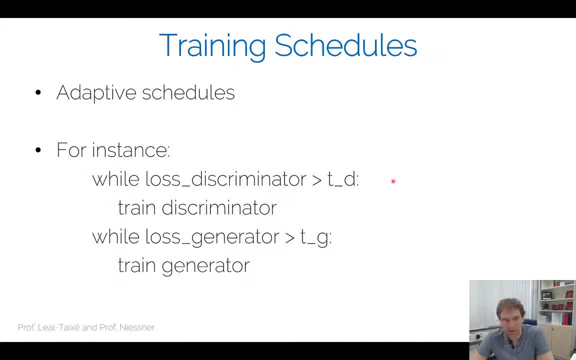 We have to train discriminator and generator. I mentioned this in the alternating schedules. Basically, what you do is you have these thresholds While those discriminated greater than threshold train discriminator While those generator greater than threshold of generator. train generator right. Again, this is not always what's happening today. You can train them at the 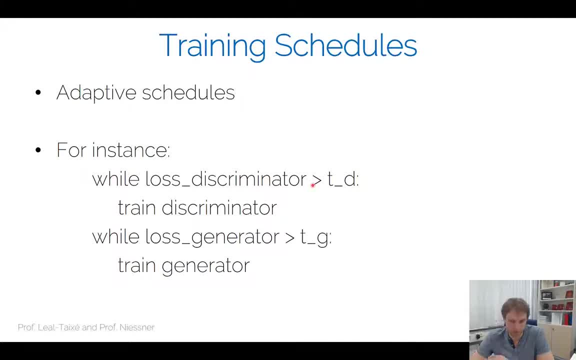 time, if you fit in your model, if your batch size can be large enough for whatever you need, and so on. And yeah, there's a lot of different things, how you can balance these two things. So this is basically the one thing that you have to play around with, and it's you need to get a bit of. 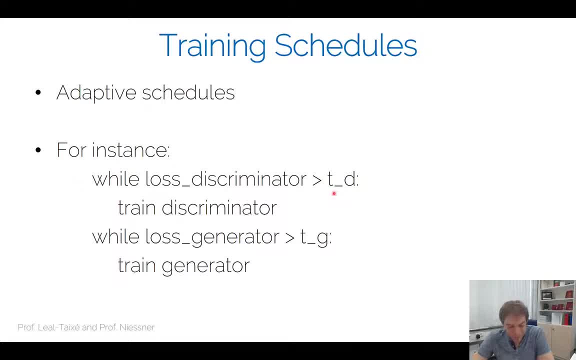 experience, which setting to use, and the problem is, of course, depending on your problem statement. these settings will be completely different. So yeah, one thing I want to discuss a little bit about the strength of the discriminator. So what is the strength of the discriminator going to do? 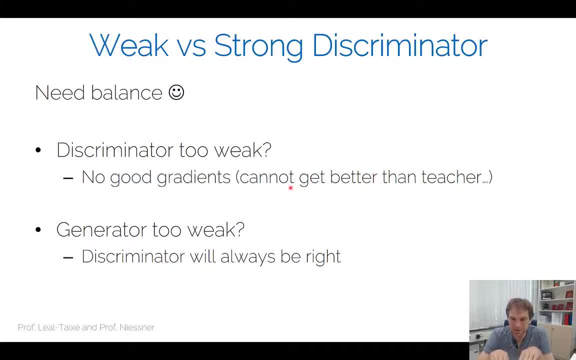 Well, the whole point of a GAN is that we have this equilibrium, right, but these two things, they balance each other out and none of them collapses, Because you could say, well, my discriminator is weak, it's not a big problem, right, because my generator cannot generate great. 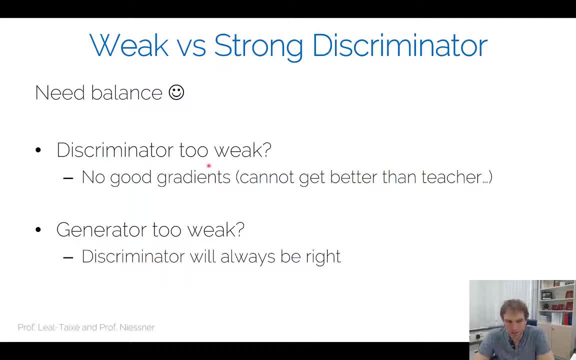 images. But my problem is, if my discriminator is too weak, I'm getting not very good gradients to train my generator. Again, there's no explicit law of the law. So if you have a discriminator that is too weak, you can't train your generator. But if you have a discriminator that is too weak, 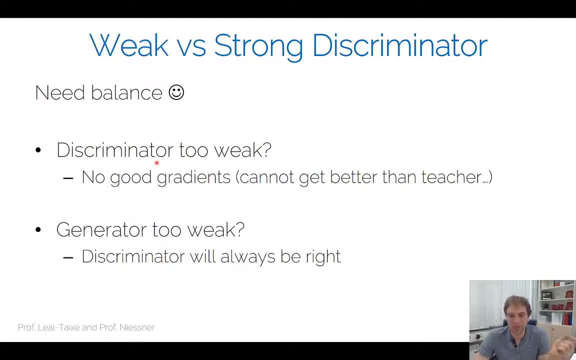 you can't train your generator Again. there's no explicit law of the law, of the law. So if you have a discriminator that is too weak, you can't train your generator Again. there's no explicit law on the generator aside from training the discriminator at the same time. 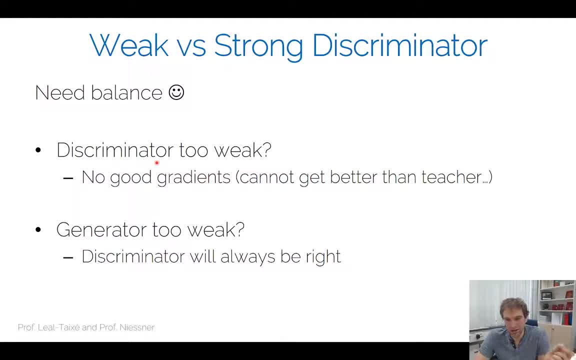 So if my discriminator is bad and I just say everything is kind of wrong or everything is kind of right, I'm not getting a signal for my generator to generate better images. So you cannot get better than the teacher. If my discriminator is too weak, I have a problem, right? It has to be strong enough to tell me what to do. 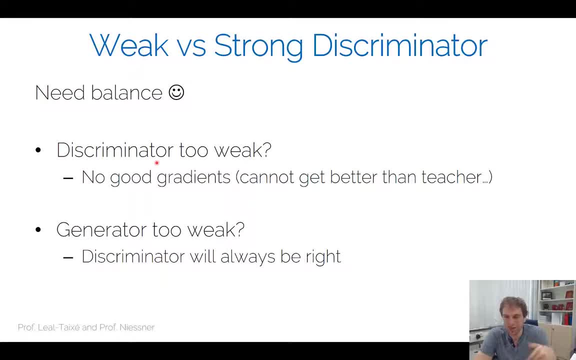 And tell me what to do means it has to discriminate and give me gradients how I get better my myself, right? this is like how this process works um. on the other hand, if my generator is too weak or if the discriminator is too strong, right, i mean, these are obviously synonyms um my discriminator. 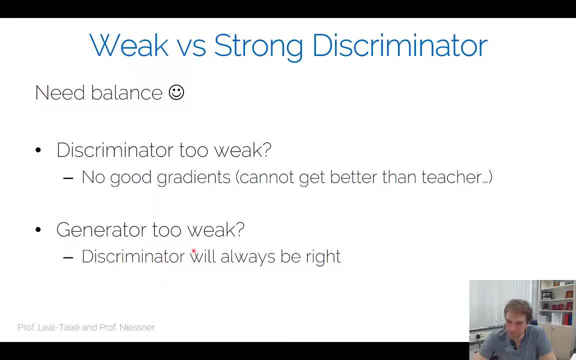 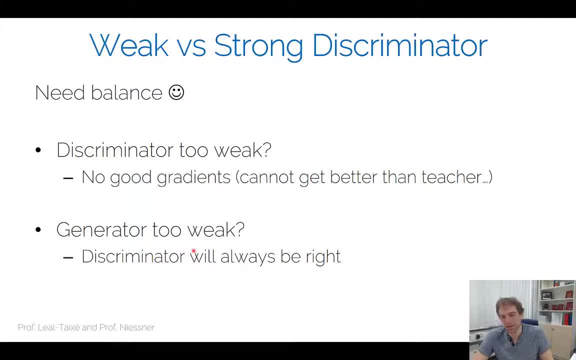 good balance. and good balance means roughly well. discriminator generator should have a similar capacity. it depends a bit on the problem, you know there's. there's a diverse set of problems where you could say, oh, sometimes the generator needs to be twice as big. um, but it's. 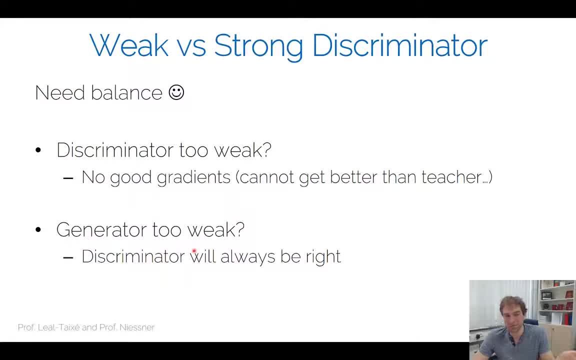 unlikely. you see something like: oh, my discriminator is like 20 times as big as my discriminator, so generator discriminator should roughly be in the same scale. if you find that the discriminator gets too strong- and this is something that will happen- um, you have to figure it out with the right. 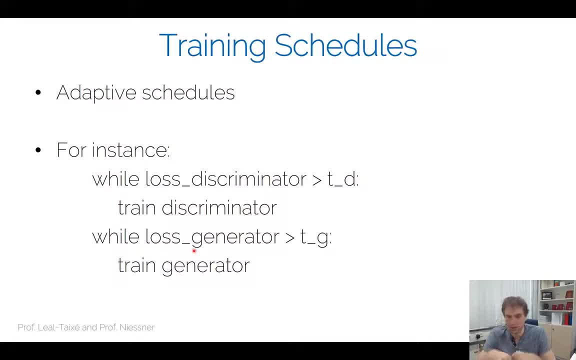 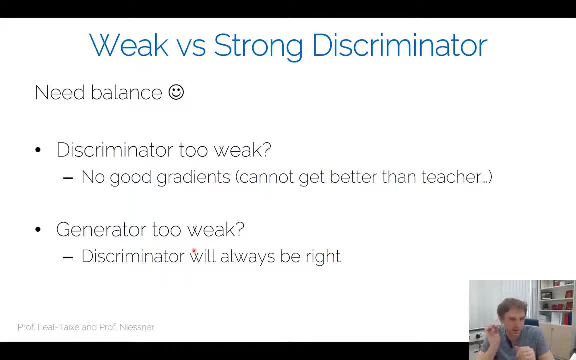 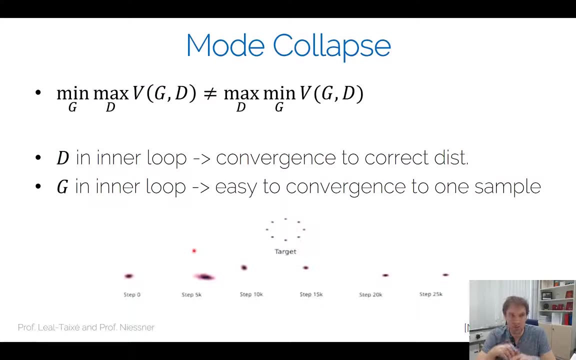 uh, training schedule- right, you have to go back here and check how to do that, possibly how to have different regularization and so on, but in practice you want to have roughly the same capacity. so that's very, very important. um, the next point i want to mention is mode collapse. i mentioned it. 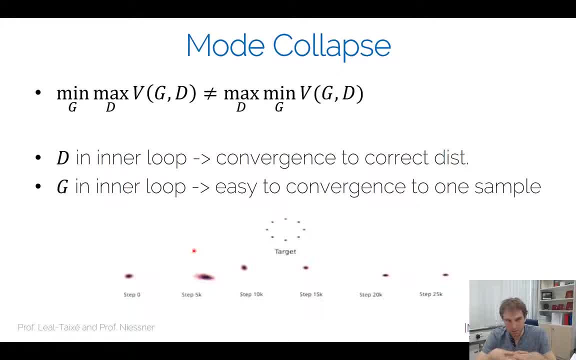 already, and mode collapse is the problem when we only generate a small number of good images. generator is generating a small number of good images and the discriminator says: well, they look like real images. seems good to me, but you don't have enough variety, so you need to have enough. 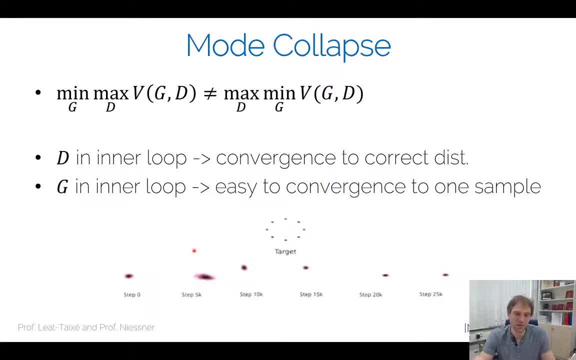 variety, and this is a problem that happens often very early in the training process, and this is a real issue. and there's this fundamental difference right now how we're ordering our training if we have the discriminator in a loop or the generator in the inner loop, right, if my discriminator is in. 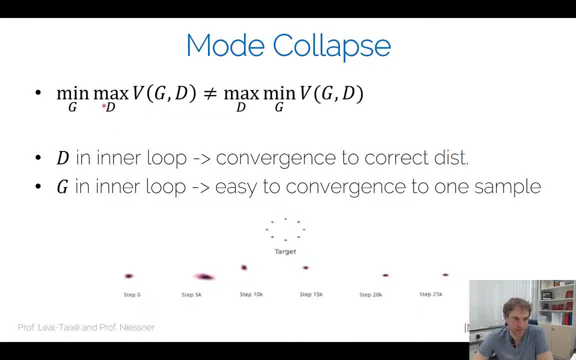 so let's, let's see what's happening here. right, i have here. i maximize the discriminator- this is my inner loop- and minimum minimize the generator in the outer loop, right there. here's the other way around. here the outer loop is the discriminator. maximize that one and generate in the inner loop. 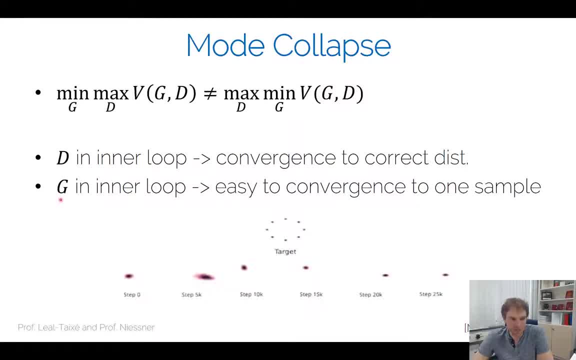 um, if my generator is in the inner loop, which is this case here, it's very easy to converge to one sample, because what i'm going to do is i'm going to. at the moment, i have a given discriminator and all i want to do is i want to fool that one. 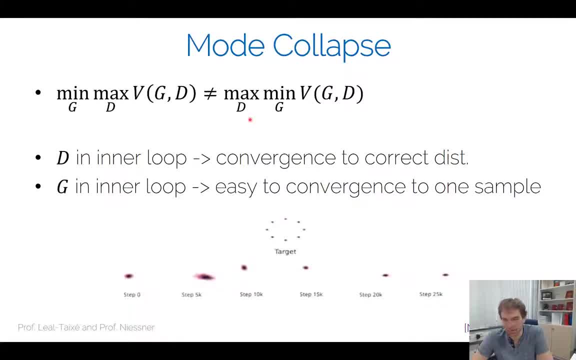 discriminator. if i always generate the same right sample that the discriminator thinks is okay, i will not get a very good distribution. so this will always- not always one example, but it will converge very likely to a small number of samples if you have the discriminator in the inner loop. 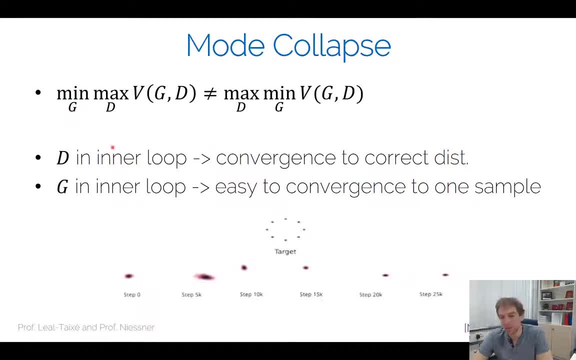 and the in the generator, here in the outer loop, then you should supposedly converge to the right distribution, right and that's very important, right. that is a very important thing because in this case i have to always be. this guy will basically be trained while this guy is being trained right, and this is what i mentioned before in this vanilla. again, this is why you, you. 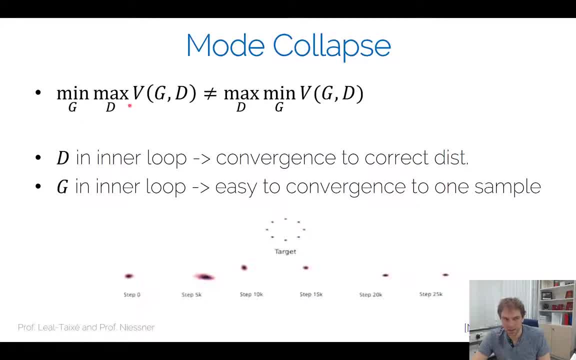 have typically first the, the discriminator loops, which is that one, and then the generator loops. however, you can still have different schedules, where you can train the generator a couple of times. here too, right, you can still do that. this really depends, though, but you have to be aware of this problem. 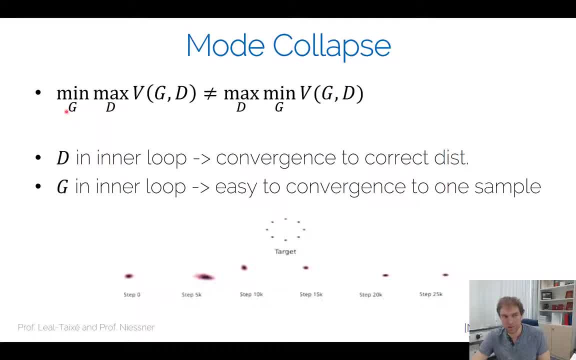 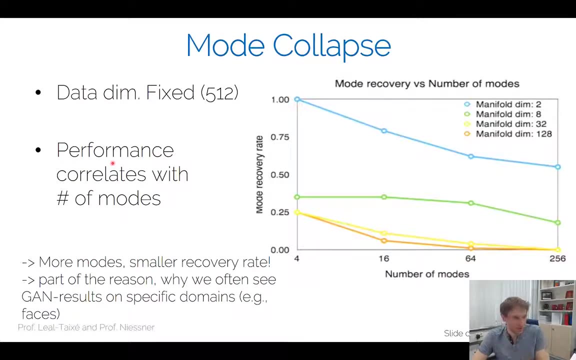 that it arises, um, if you're training this guy now in the inner loop, you will typically mode collapse and that's the thing to to consider. um, yeah, i'm going to talk a little bit more about more collapse. another interesting thing is the data dimension. what you're using so, um, so this is a a graph here. 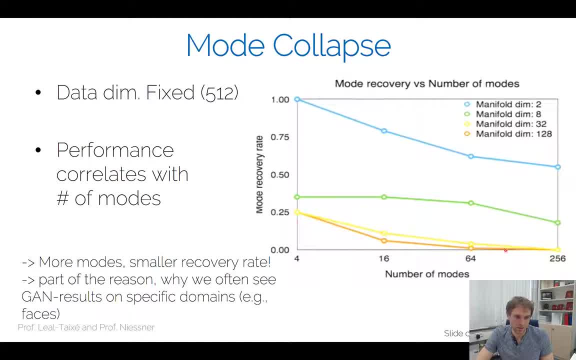 this year. um, these different curves are many fault dimensions, right? um? this one is the number of modes that we're trying to recover and this is the percentage, what we actually did recover, right? um? so if we're having more modes, it's, of course, harder to recover all of them, meaning that the 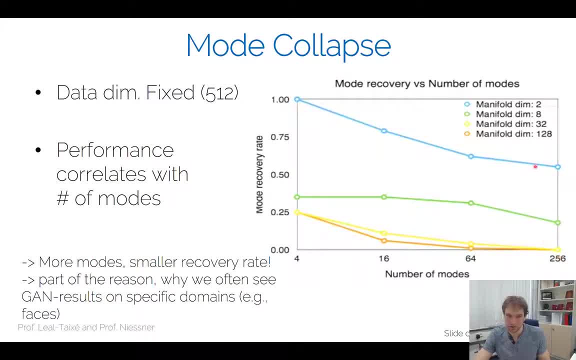 recovery rate will typically go down. now what we're trying to measure here is we're trying to have the mode recovery, with zero周 recovery, versus the number of modes. So the performance correlates with the number of modes. That's what I'm saying. If I have more modes, it will be. 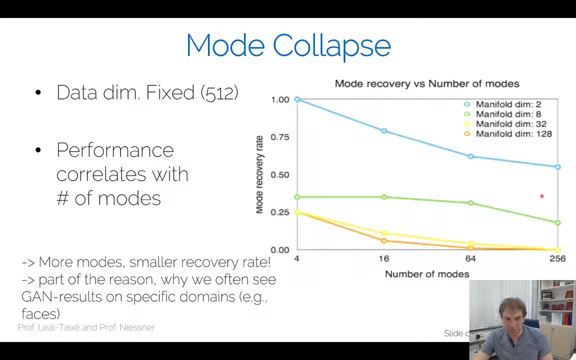 harder. If my manifold dimension is going to be high- this 128, then this is even more extreme. If my manifold dimension is lower, this is a bit easier. So the higher my dimension, the harder. Yeah, so part of the reason why we often 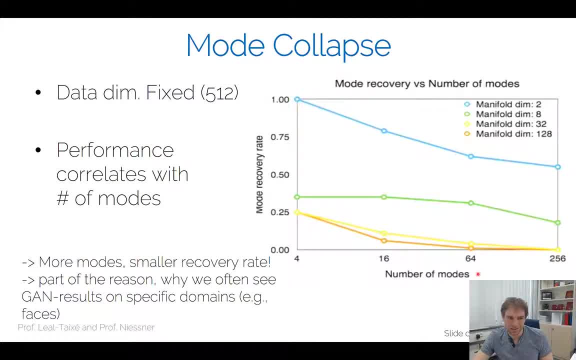 see GANs on specific domains- is because we want to simplify our distribution. We simplify our manifold, basically, And because of that I can most likely recover- well, I wouldn't say all modes, but I recover a lot of modes. 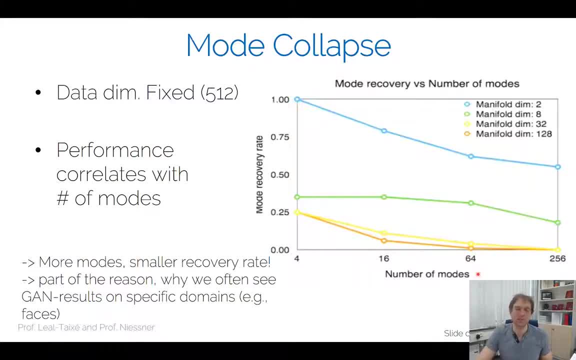 You never recover all of the modes, right, And that's unlikely. Well, this is a toy example, This is not a real image example, right? But in practice, if you're having a simpler domain, you can recover more modes because you can sample the full domain and then the 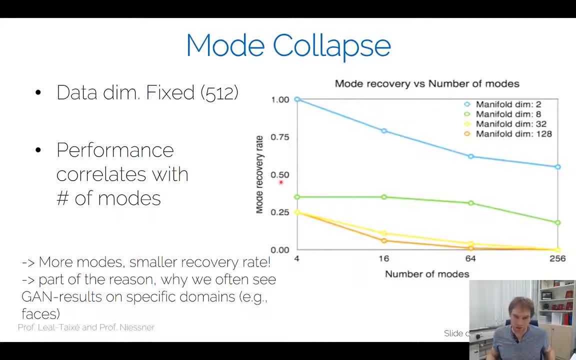 training becomes easier If you're having a larger domain. in other words, what could happen is my generator picks a pretty good sample, looks like a real image, it matches most of the other stuff, but then it turns the same image again. 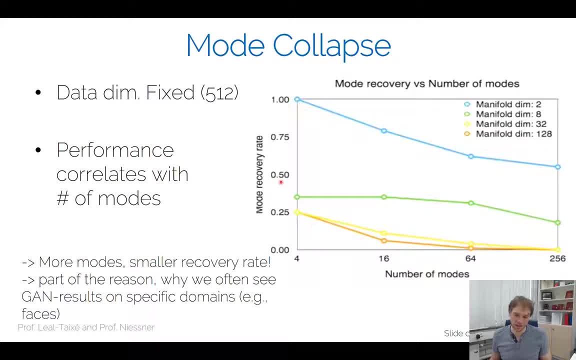 right, Then the generator and the discriminator can't tell it apart. So in practice this is. it's very important here that you're saying: number of modes makes my recovery rate lower, because it gets harder And often what we see is: well, we're seeing. 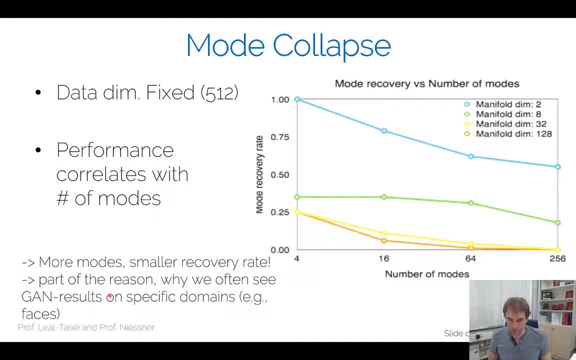 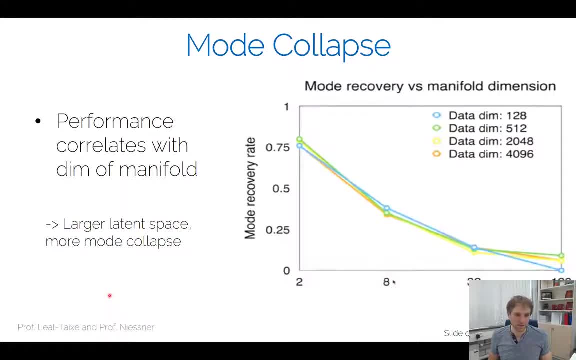 like smaller distributions, so we don't have to recover so much stuff. basically, This is why phases work pretty well and image net doesn't work so well. Let's have a look again at the manifold. Well, we had this partially from the other one. 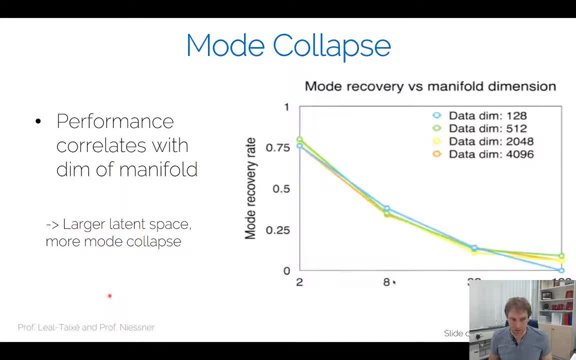 but if you're looking at the mode recovery versus the manifold dimension, a larger latent space means more mode collapse, which makes sense because it's harder for the discriminator to figure out this entire space at once. right, It can monitor it, so to say So. 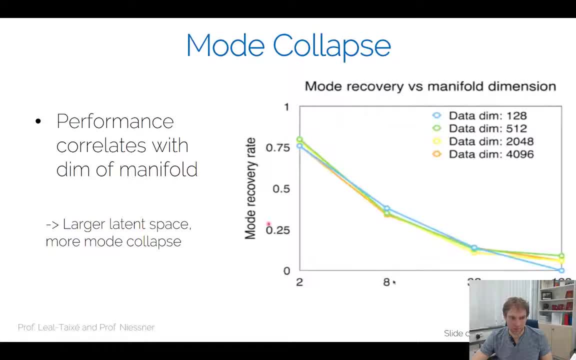 here. what we're seeing is: here we have the recovery rate again and here we have the manifold dimension right. We have also the data dimension, like manifold is like latent vector z dimension right, And this is the data dimension. The data dimension doesn't. 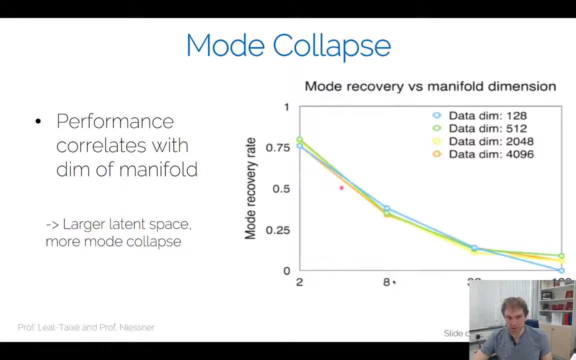 seem to matter too much here, But basically it goes down the larger the space. But you also want to have enough control eventually, so you want to have reasonably large space. So this is something you have to also consider, like how big you want to make that space. Yeah, the reason why I talked. 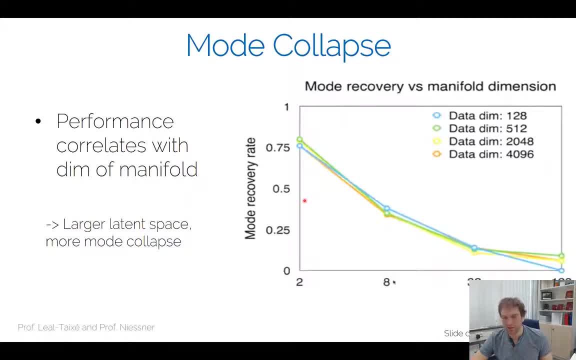 about this mode collapse. this is something you can and should figure out early on in your training processes. Again, how you do it: you just visualize a bunch of samples in TensorBoard and then you see how to divide them. I also want to mention some of the problems that GANs have And the funny thing. 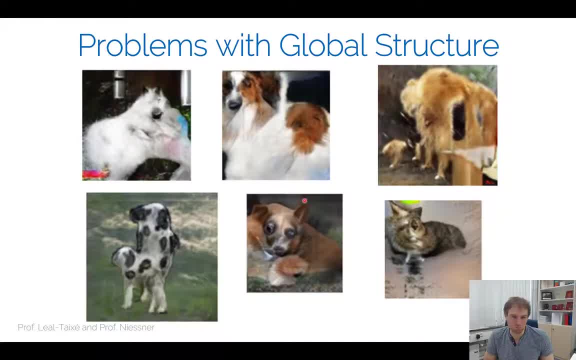 is these images? on the first glance, look kind of cool and look like a real image. We're getting fooled by this, maybe too. but what we see? they are not real images. If you're looking closely, I don't know what's happening here or here, right, It looks like a dog, like a bit of dog. 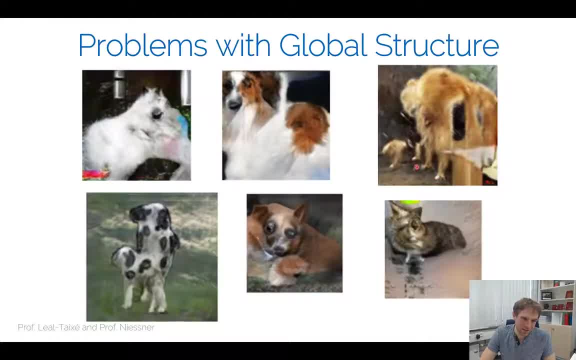 here a bit of dog. there looks like one, two, three legs. here Something went really wrong, But on the other hand they look kind of a reasonable color distribution. So the global structure is a big problem for GANs And it's not surprising that if I'm making my image dimension bigger and I have a larger 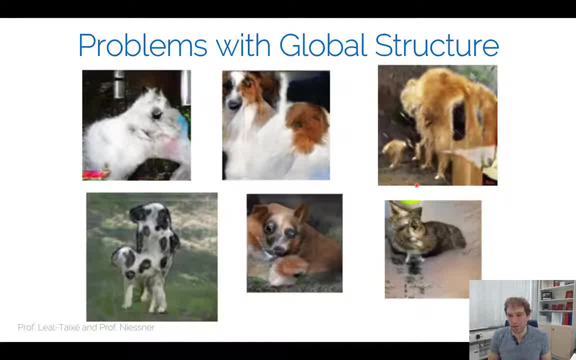 image to generate this global structure will even be harder to be achieved In practice. you have to train longer. in practice, you have to have bigger models. but the bigger your model, the longer you have to train, the more likely it is to have things like 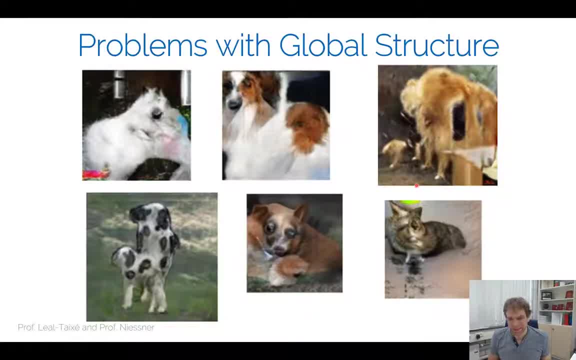 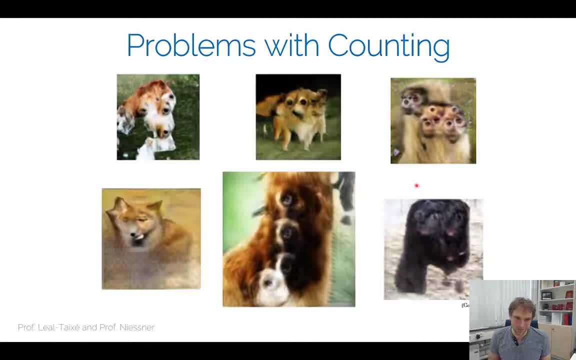 mod collapse or your losses diverging, So that's an issue. Generally speaking, with this structure, one common problem is you have often problems with counting. These are fun samples. You have a lot of eyes sometimes Here, a lot of eyes, I think. 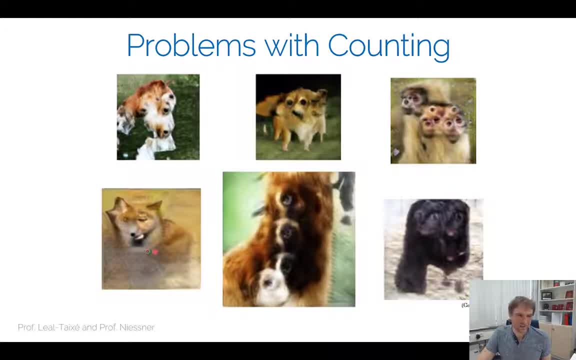 I don't know what's happening here or here. Something went really wrong, Like locally, the features are okay. If I'm going to give you this little patch here, it looks perfectly fine, But the global counts are just wrong. One thing: 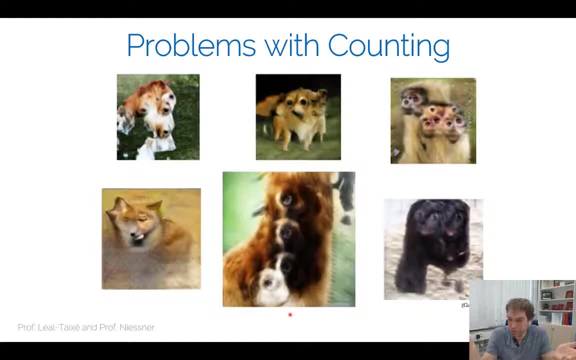 You have to also consider, like theoretically, what we're doing. GANs are perfectly sound, We have this generator and we're learning kind of this implicit distribution. Now the problem is: implicit distribution is still being represented by a series of 2D. 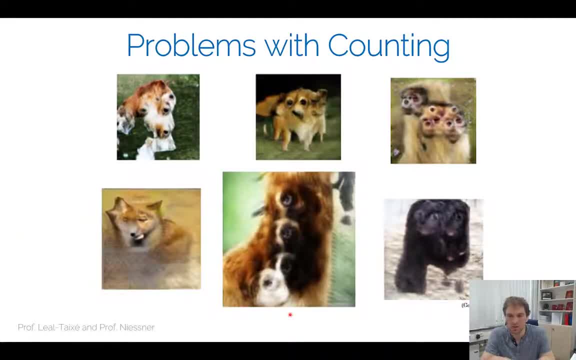 deconvolutions. You have a bunch of 2D operators that have to encode the whole space of images in the training set And convolutions are inherently a local operator. Local means well. I mean I have a 3x3 conf. I can locally check what's going on. 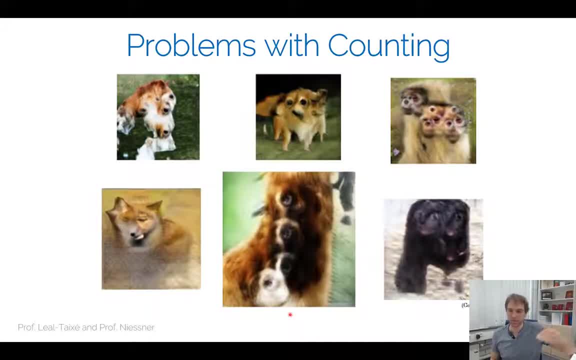 And in order to get a larger receptive field, I have to have a series of convolutions, And that's a thing that is very much exhibited in these cases here where you know the larger it gets, the more global the structure has to be, the harder it is for ConfNAND to do. 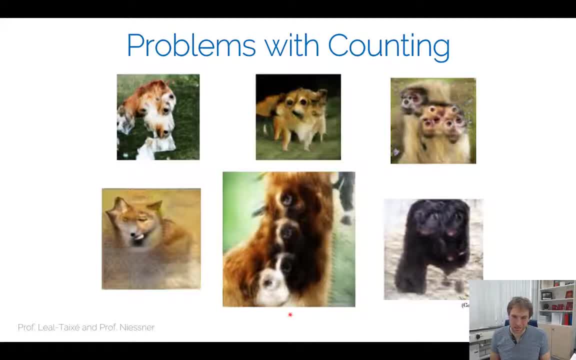 it. Yeah, it's just how it goes, Yeah, Okay, So these are common things, when we see where we have problems. I talked a little bit about it, what you can do when you train GANs and how to evaluate it. 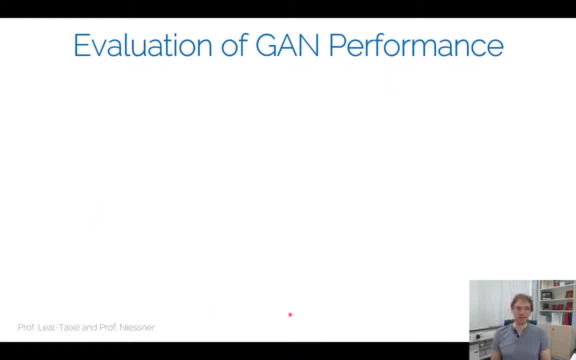 The question is: how do we quantitatively evaluate the performance of GANs? We already noticed that, yeah, the loss function is not going to cut it for us, right? The loss function is not going to be so easy to look at. 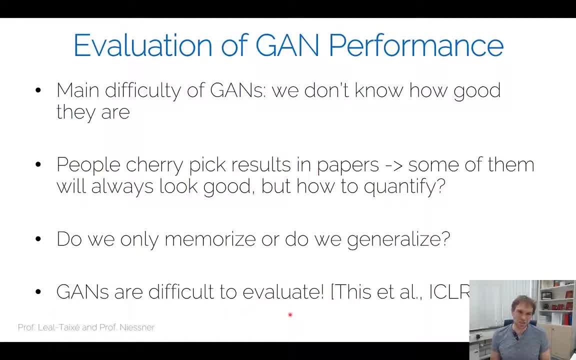 The main difficulty that we have with GANs is we just don't know how good we are. We don't know whether they converge, we don't know whether we need to train longer, we don't know whether it's not working right now and it will get better, and so on. 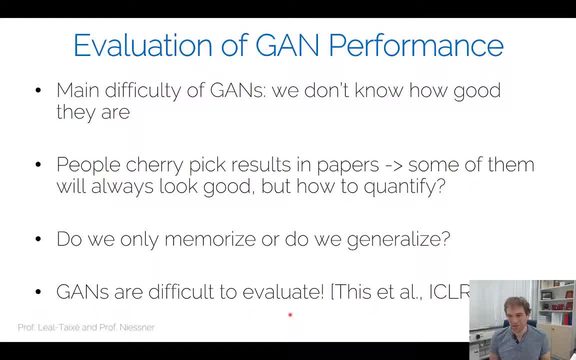 But it is a very, very difficult problem- And the research community. I'm a researcher, I can say that I'm part of this community. but one weakness of the community is often in papers you see very, very good results And what you can do is you can just sample a couple of times and take the good results. 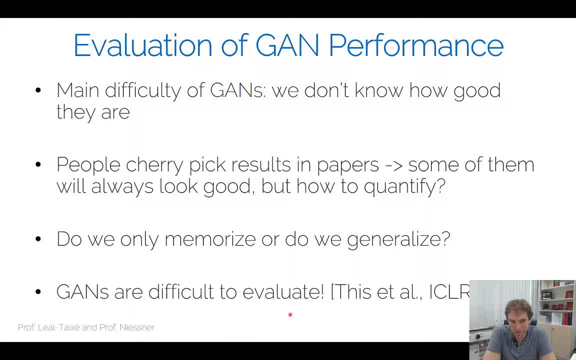 and cherry pick them. And that is a problem, right, Because we would love to quantitatively evaluate, but it's very difficult. So does it always look good, or is only some of them being good, right? What are the good? 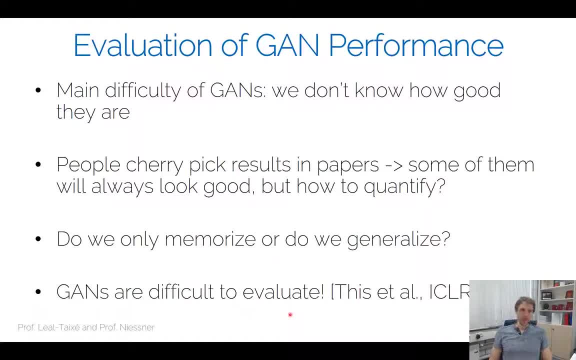 What are the bad cases? What are the hard? I can't put it so easily in a table. The second question is: do we just memorize? do we generalize, right I mentioned? oh well, we have a training set in the real samples. do we just memorize? 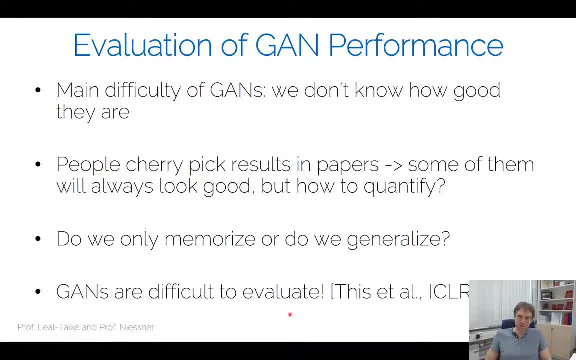 a bunch of them. If we're memorizing these ones from the training set, my discriminator- by the way, if I'm perfectly memorizing it, my discriminator- can't tell them apart. there's no way. So the idea is, my training set has to be big enough that my model capacity can fit in it. 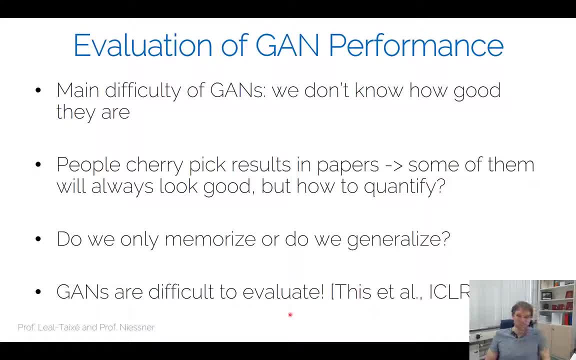 That's still the same thing. you can still have overfitting problems here too. Yeah, But it's difficult. It's very, very difficult. So what do we do in practice? Well, in practice, one thing I told you: we look at the images, we're looking at the human. 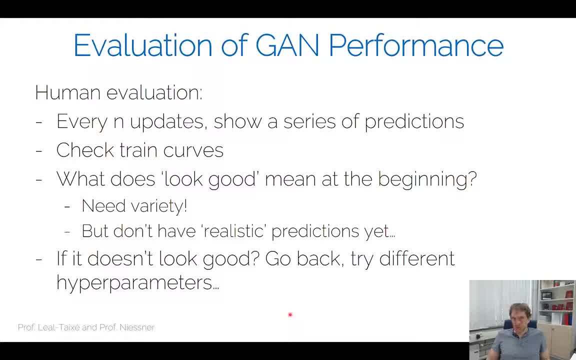 evaluations. Every update steps, you show a series of predictions. These predictions typically should be from the same latent code. right You have? maybe you're showing like eight by eight images, but they're always the same latent codes you're visualizing. 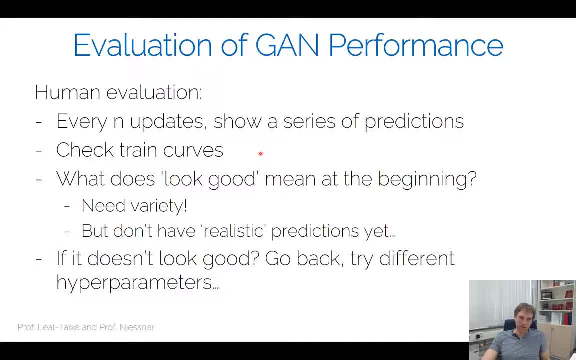 Check the training curves If you're diverging, if discriminator is collapsing Here, check two, Okay. Check if it's getting better or check if you have mode collapse. These are the things you can do. At the beginning it doesn't look very good, but you can check if you have enough variety. 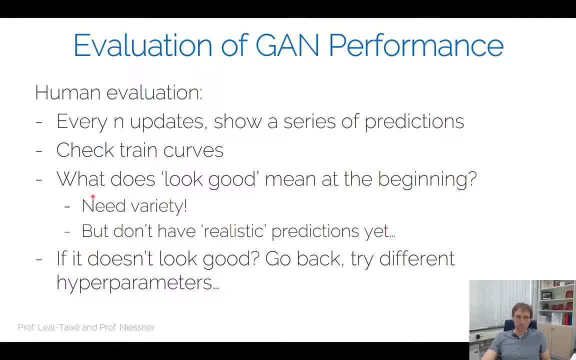 If you visualize eight by eight images and you only have like three different types of these eight by eight images and you have a lot of duplicates in there, even they don't look very good and you have a lot of duplicates, it's a problem because you just mode collapsed. 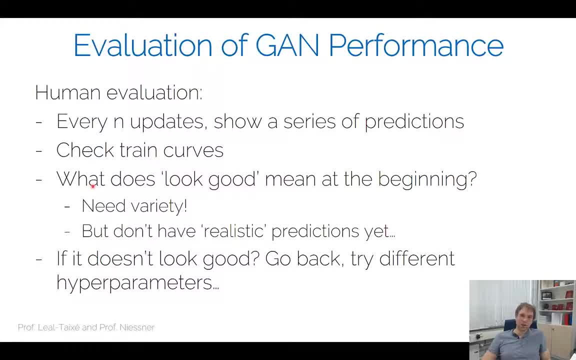 right. This one you see very much early on. If this one goes wrong at the beginning, it'll never recover. That's just a big issue. Yeah, If it doesn't look good, what do we do? We go back to different hyperparameters, different networks, different learning. 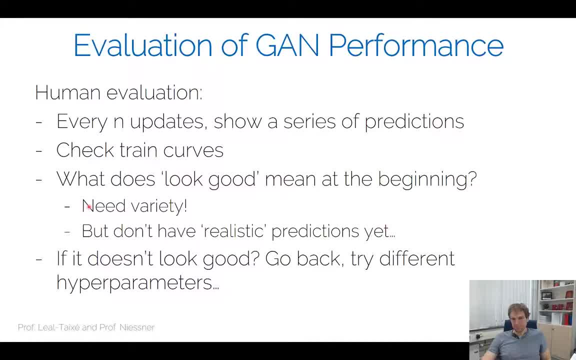 Most of the time, the learning schedules make a big difference. That's one of the number one things you can try. Okay, This is human evaluation. There's also some ideas of doing quantitative evaluations. Okay, Let's see, Let's do this. 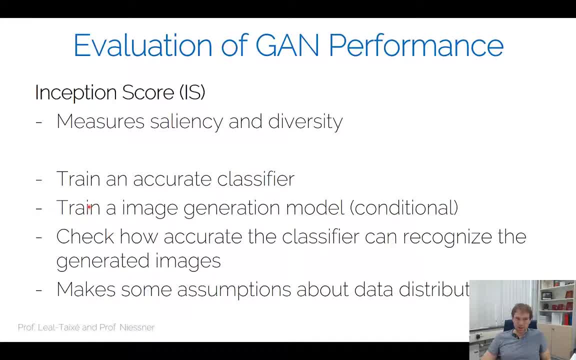 One of the most popular ones is called IS Inception Scores. I can already say there's a caveat. The Inception Scores: they're not perfect, They're not telling you 100% what's going on. The Inception Scores: they measure saliency and diversity. 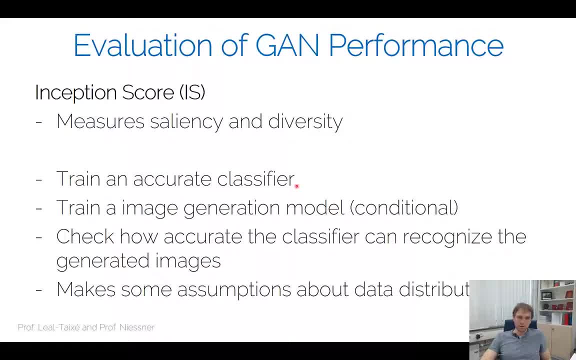 Typically the idea is that you can do a lot of things. You can do a lot of things. You can do a lot of things. ixo can do far more than that. You can do a lot of things. The idea is basically: you train an accurate classifier. 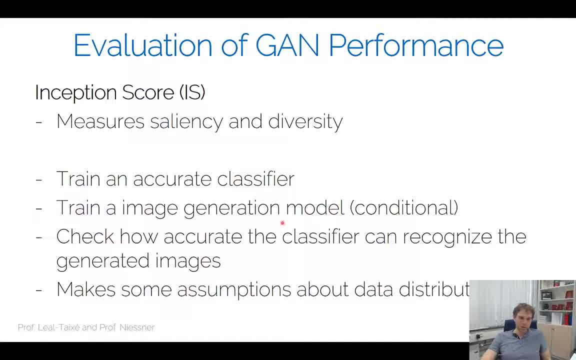 You train it in an image generation model and then you check: how accurate is the classifier? Can you kind of recognize the generated image? That's kind of a high-level idea. You make some assumption of the underlying data. What do we want to do is – let's say I'm going to generate images from 10 different 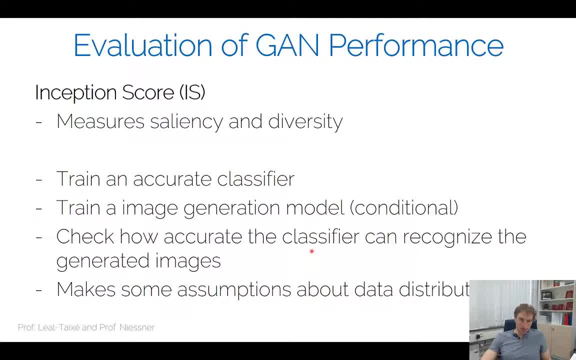 classes and I want to make sure that my classifier can answer those. What do we do? can associate each of the generated samples precisely to one class. So let's say I'm generating cats and dogs. If the classifier tells me it's a dog, 100% dog, I'm good. 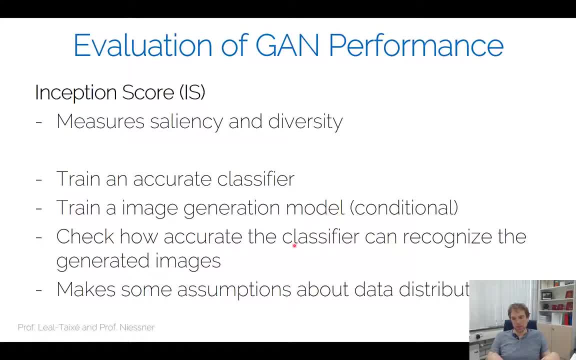 If it tells me it's 100%, it's a cat, I'm good. If it's half dog, half cat, they're not so good. Then I generated something weird. right, That's kind of the idea, And this is called saliency. 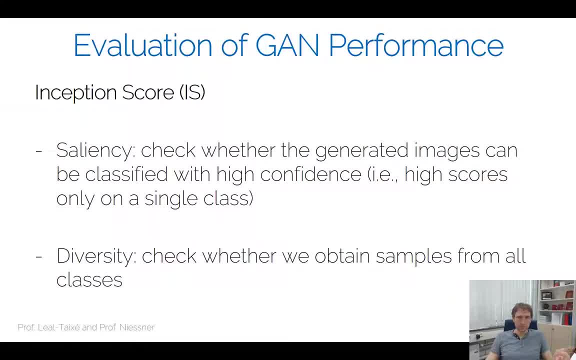 This is the first term we have to consider, So check whether the generated image can be classified with a high confidence, And high confidence means you just look at the classification scores. Really simple idea Works to some degree, right, I mean, of course that's important. 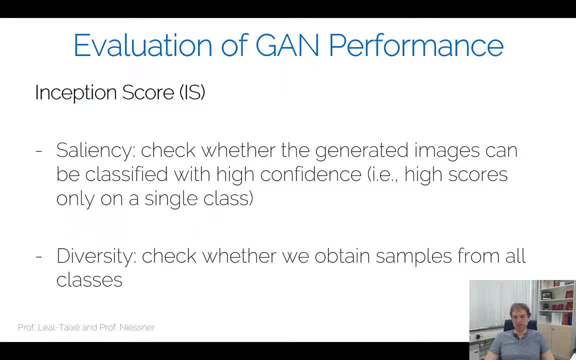 We need, however, a second part, which is telling us we need some diversity. It doesn't help us if we only generate good dogs but no cats. It's not good to think, So we need to check that we get a uniform distribution of all classes. 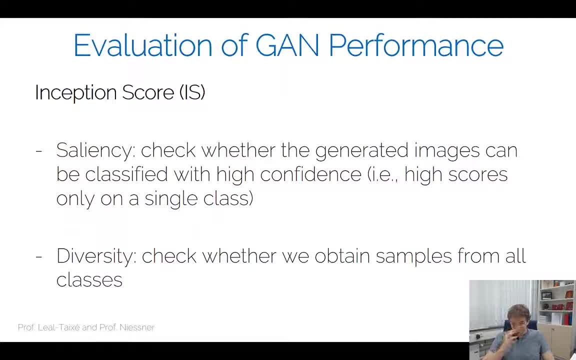 This is what our evolution matrix should tell us. Yeah, because we want to have both right. We want to have diversity, we want to have saliency. That's what the Inception scores are measuring. There's still a problem. 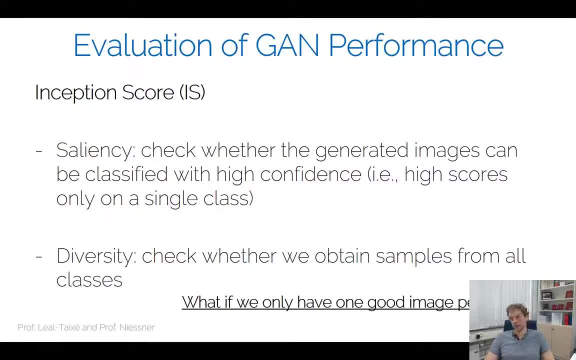 And one problem is what happens if you have only one good image per class And if you have enough classes and we have one image that is good per class but every other image per class is not so good or we don't have a lot of other images, we might still be mode collapsed. 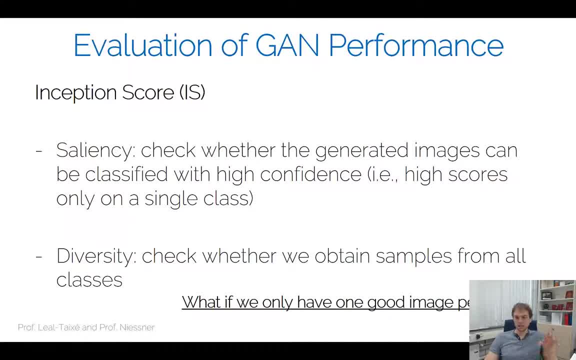 And we might not notice it so well With Inception scores. So even though Inception scores might be high, diversity might not perfectly be covered right. So the short story here is: Inception scores is what people use to quantitatively evaluate it. 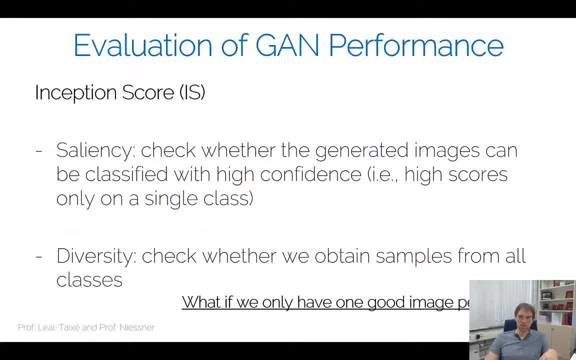 There's a couple of variations of this, like FID scores and stuff like that. They're all very similar, But I can already tell you they're not perfect. None of them are perfect, So we have to still look at it. This is a difficult problem, right? 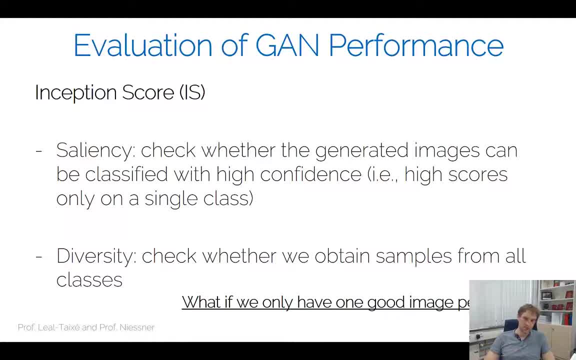 It's basically like: oh, look at a picture, Tell me how realistic is the picture? Like that's the question we had at the very beginning, when we said: well, we need to have a loss function to reconstruct or generate images. right? 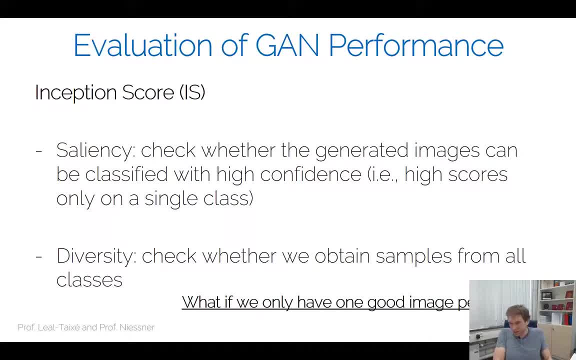 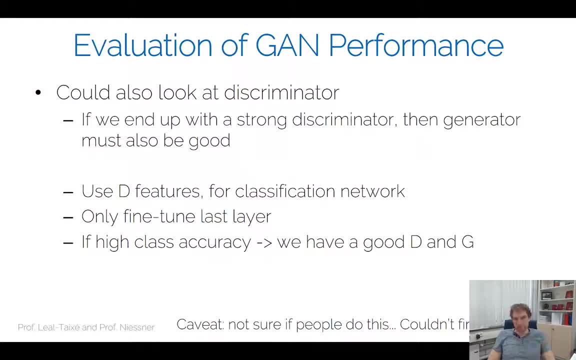 That's what we're learning with the GAN, But the GAN is learning and we have to develop it again now, So it's very difficult to do this by hand. There's a few tricks you can do. You can check the discriminator. 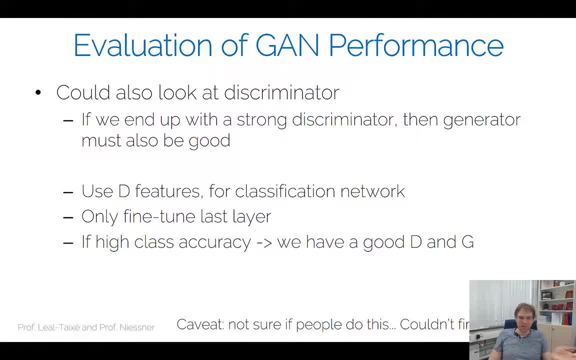 If the discriminator. By the way, it's a good debug. Whenever you start training again, always train the discriminator first, Check if it's going down to zero. Of course you're not getting reasonable results, but you're checking that the discriminator can go to zero. 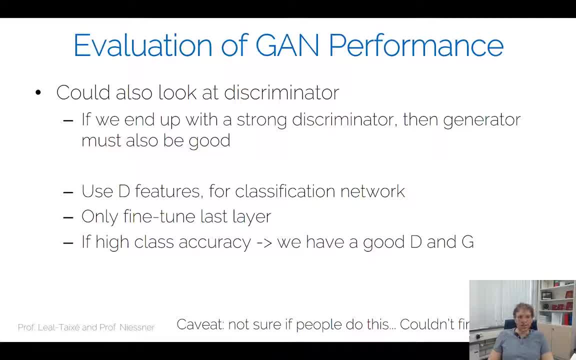 If that one doesn't work, then you're something is wrong. But one idea what you can do is you can train the discriminator in a GAN. You can take the features of the discriminator, can put this into a classification network as a pre-trained feature learner. 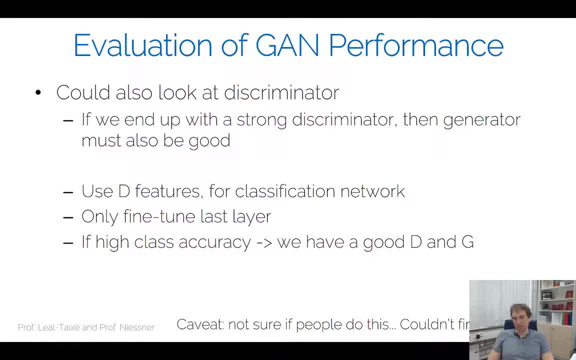 fine-tune it a little bit and see if you get good features for that. If that is the case, then you would assume you have trained a good discriminator because you got good features out of it. If that happened, if you got these good features out of a discriminator, you would assume the generator must be also good. 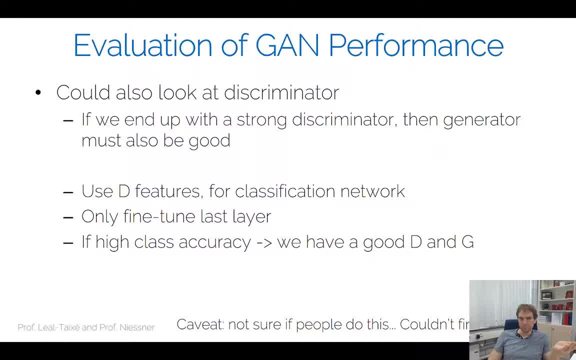 It's just how it goes. If the generator- Yeah, the generator- must be good, in that case, That's the thing I feel is a bit hacky, but it's at least one way to figure out: oh, do we get good features or not? 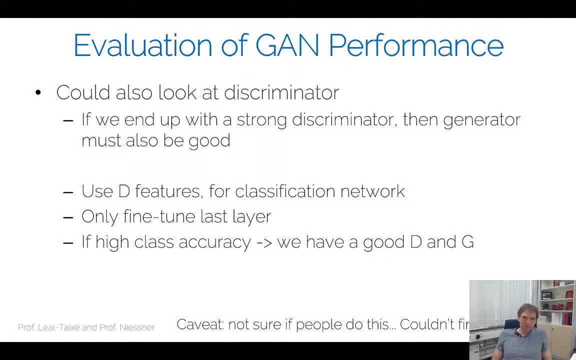 Okay, That's for now. it for how to evaluate GANs, but in practice, I can already guarantee you it's very tricky to train them. So I wanted to talk a little bit about what can we do to make GANs work in practice. 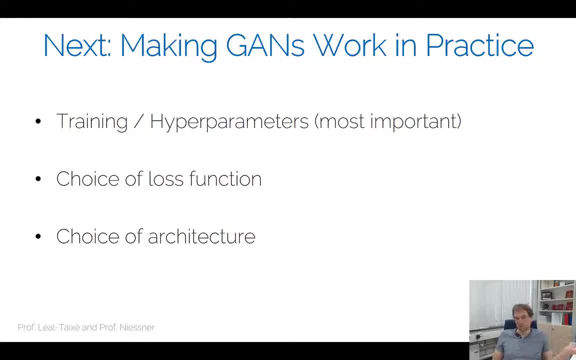 In practice, there's three different things you can do. You can fix hyperparameters right Training schedules, learning rates- possibly optimizers, possibly optimizers, possibly samplings, possibly data distributions, training sets, stuff like that. That's the most important thing we're going to look at. 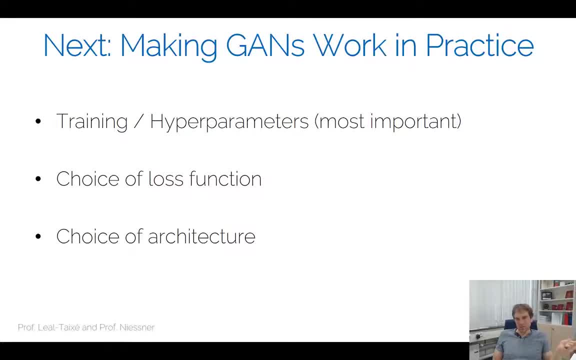 There's a lot of other things we're going to look at. There's a lot of other things we're going to look at. There's a choice of loss functions. We have seen two loss functions so far. We have seen the standard, minimax, GAN, right. 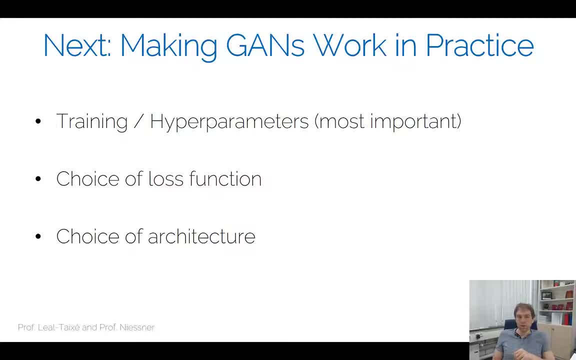 We've seen the heuristic method. We'll introduce a couple of more. And then there's a choice of architecture. What deconvolutions do you use Stuff like that? For the most part, we're only going to look at this one to debug. 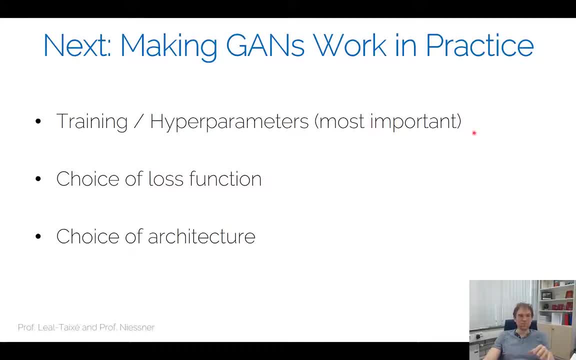 This is the most reasonable thing to look at In practice. people always look at the other two, which I don't understand why. So they're changing the loss functions all the time, Because nothing works. change the loss function, That's always a thing. 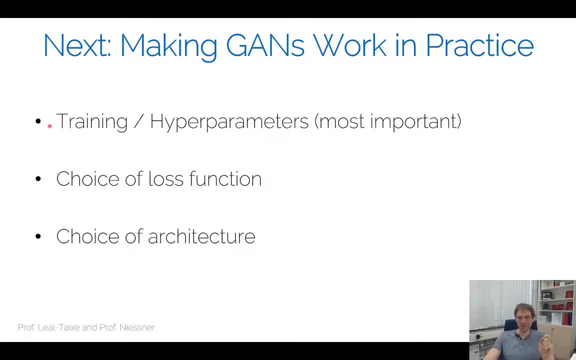 But I think it's a terrible advice. You should always look at these ones here first. In practice, starting with the heuristic method here is a good idea. Architecture: start with the DC GAN. That's why I mentioned it. It's also a good idea. 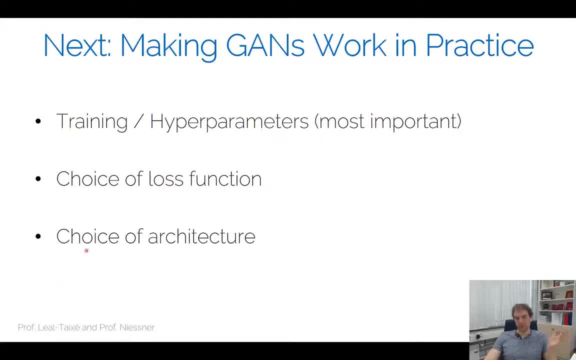 They might not be the best ones, They might be better ones, But these things they work if you're choosing the right hyperparameters. Okay. Yeah, let's have a look at a couple of practical things that people have been looking at. 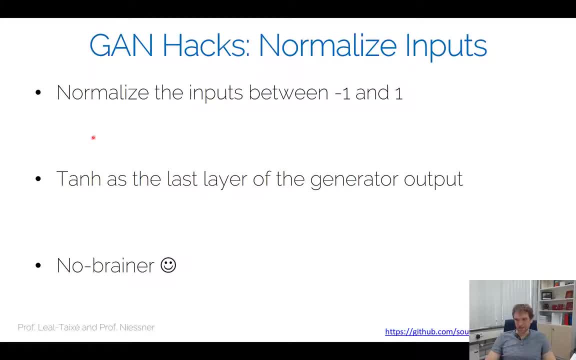 And there's this cool website called GANHex. Some of the stuff might be a bit older now, Older like two years old maybe, But there's a couple of cool things on this GANHex website, So I wanted to quickly go over it. 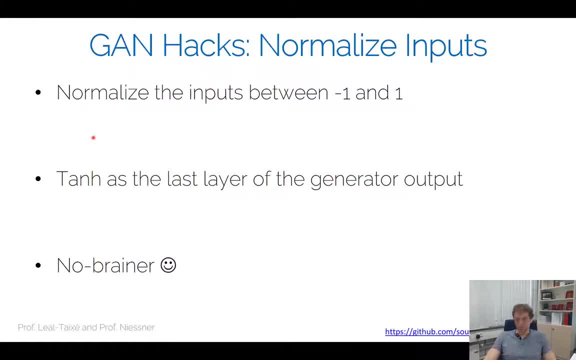 There's a few things you want to do: Normalize the inputs, That's a no-brainer, Because you want to make sure your distribution is within a reasonable space, Like if you have. If your distribution is bad, then it's very hard to learn. 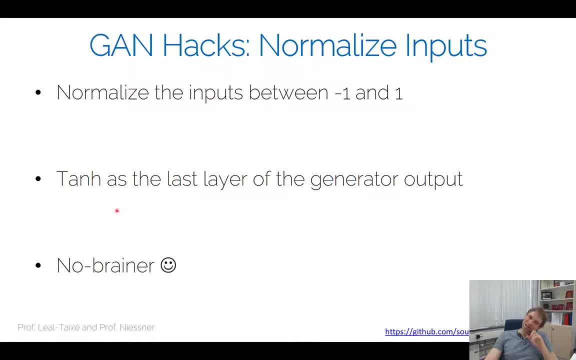 What's very important- and this is a general thing, by the way- check out your last layer of your generator Most people use. If you normalize it here between minus 1 and 1, you have a 10H that maps it between minus 1 and 1.. 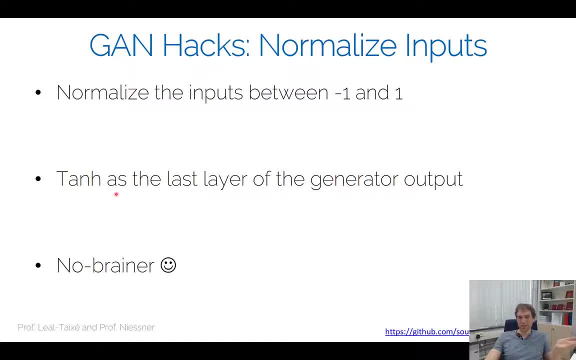 So, by definition, your generator will generate samples that lie in this distribution. Let's say, for simplicity, I'm going to go ahead and I'm going to use, instead of a 10H, I'm going to use a sigmoid. A sigmoid will map my values between 0 and 1.. 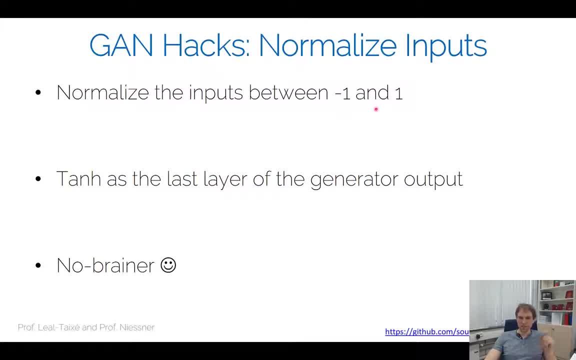 But if my inputs are between minus 1 and 1, I think my discriminator has a pretty easy thing to say: well, if there's no negative numbers, it's all fake. So these are common problems that people have. Or if you have a relu. 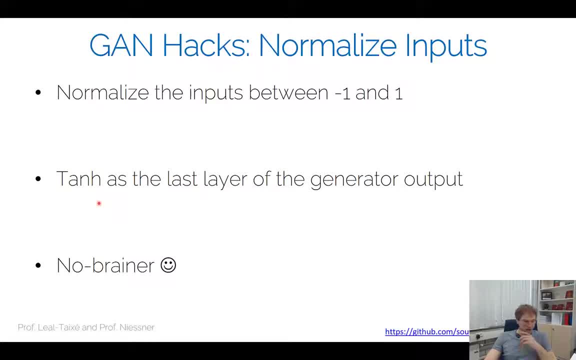 Oh, by the way, this is the most common bug that people have. They just say: in the last layer of the generator they have a relu and this one is some weird normalization that goes negative. So make sure these two things match each other. 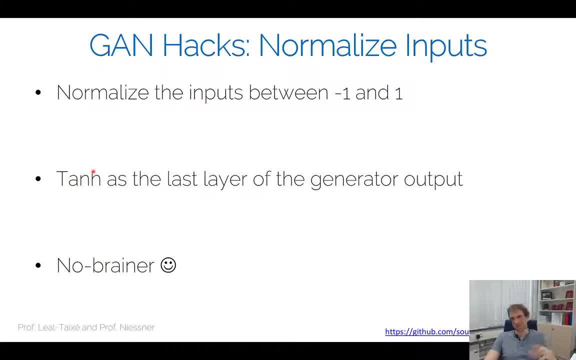 If they don't, you've got a problem. by the way, Obviously, you don't learn anything. Your curves will just immediately collapse. By the way, try it out right. I mean, just do something like this and use a relu here or a sigmoid. 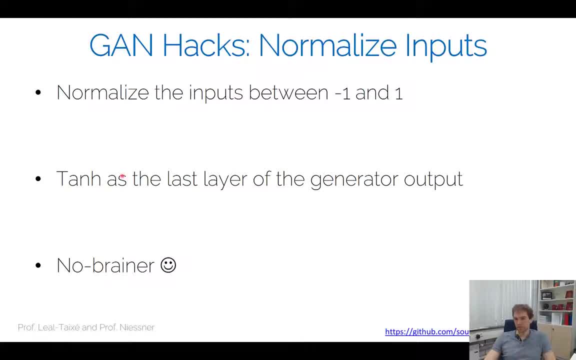 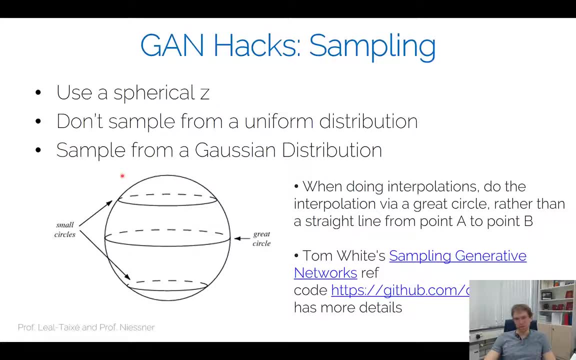 I think your discriminator should just go immediately to 0,. right, It's just straightforward Sampling. What kind of samples do you use? I mentioned before, people can use a uniform distribution. Most people use a Gaussian distribution to sample in the latent space. 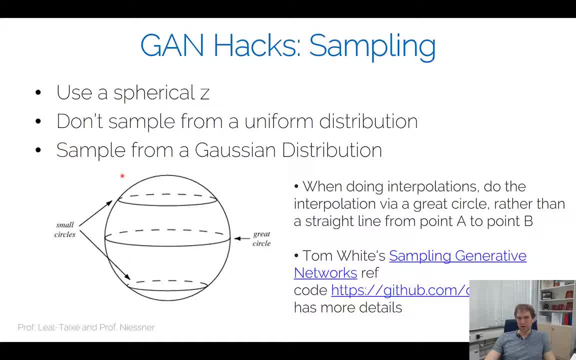 What people often say is: use a spherical sampling, And spherical sampling means it is a Gaussian sample but it lies on the sphere, So the length of the vector is always going to be 1. So you just normalize your sample space. It makes it a little bit easier. 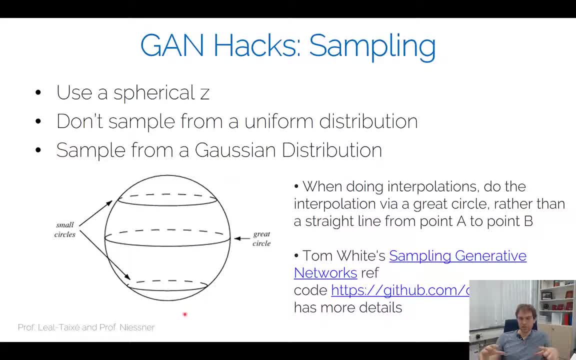 The reason is you, just You still have the same control in terms of the dimensionality, but the number of the dimensionality, Sorry, your effective parameter space goes, It becomes a lot smaller. Okay, And when you do interpolations, you can interpolate on this spherical sample here. 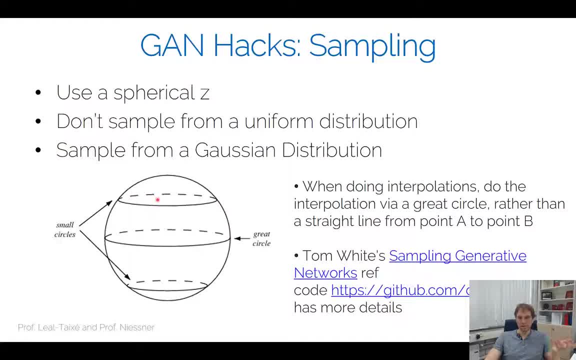 You can say, oh, you have to check on the grade surgery right, Like how you interpolate from one sample to another one. There's a lot of literature, by the way, how to do the sampling. You can normalize it to make sure it's on a sphere. 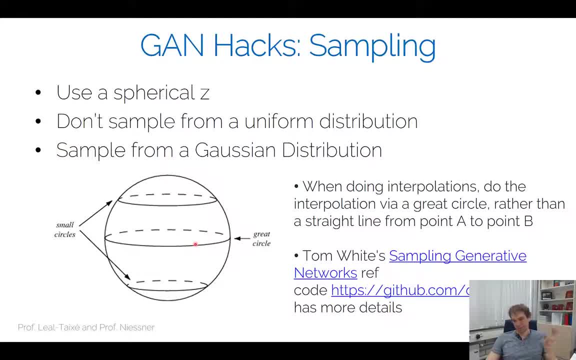 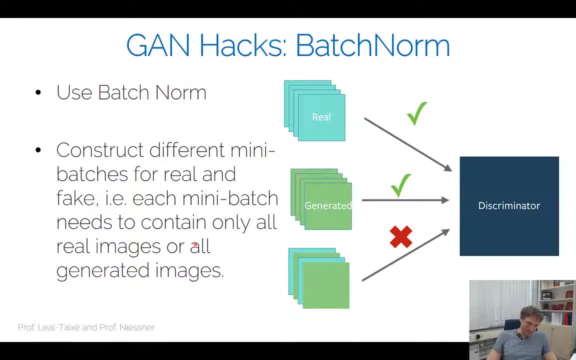 You can also not do it. There's a lot of different things. It depends a little bit on the problem. Batch norm is a fun thing. This is a thing I would take with a bit of a caveat. A lot of people say, oh, don't use batch norm anymore. 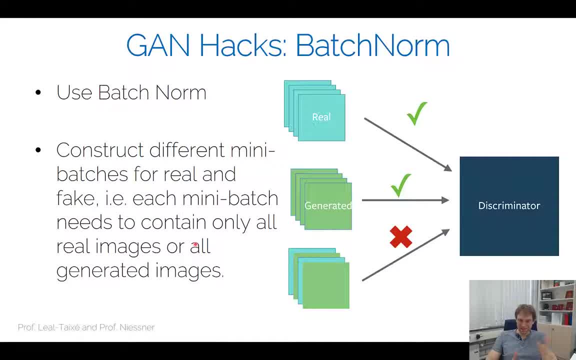 I would say it depends, but it's one thing you can play around with at least. Sometimes you also just need a few options With without batch norm. that's one thing. Typically, people use batch norm. That's what they recommend here too. 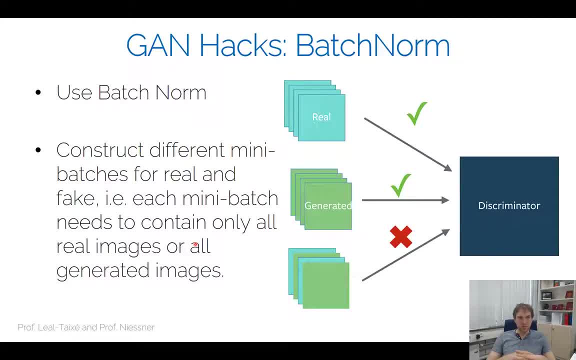 It depends a little bit on the problem. What you can do is you can construct different mini-batches for real and fake, Meaning that you can say One mini-batch contains either all real or all generated images. That helps to stabilize the training a lot. 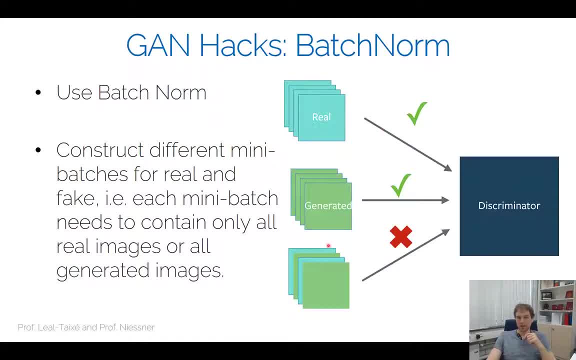 The reason is basically you're getting all gradients for real or all gradients for generated. That makes especially for the discriminator. it makes it much easier to train. That's the thing typically people do. It depends a little bit on the batch size. 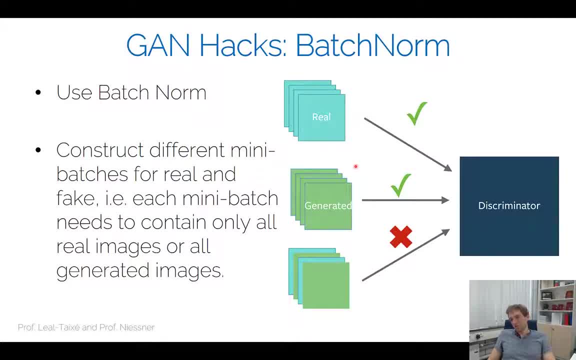 I don't have an advice here. One problem is- We'll see this later in the next few lectures- There's two state-of-the-art GAN methods. One of them is the style GAN line from NVIDIA and the other one is the big GAN. 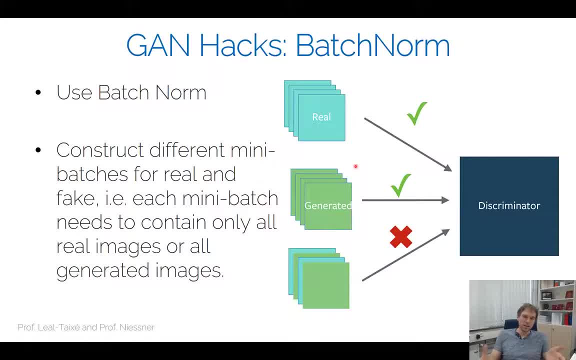 I think that's from Google. These two are probably leading groups like training crazy big GAN models for weeks, basically, and try to get good results. One of them uses small batches, One of them uses big batches, Which is contradicting the settings. 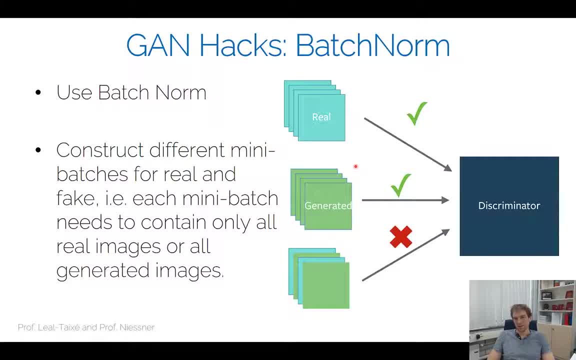 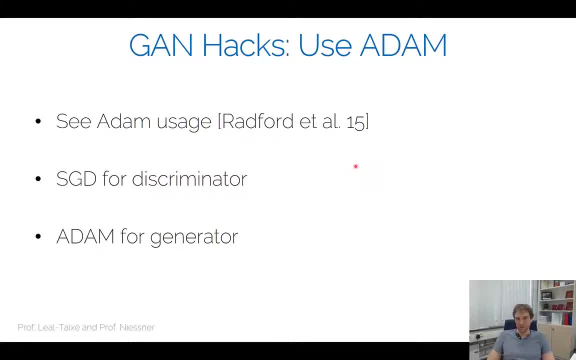 But they both get good results, But in between nothing works. So that's It's an interesting thing. The optimizers people typically use Adam for the generator, SG for the discriminator. That's a thing you can play around with. 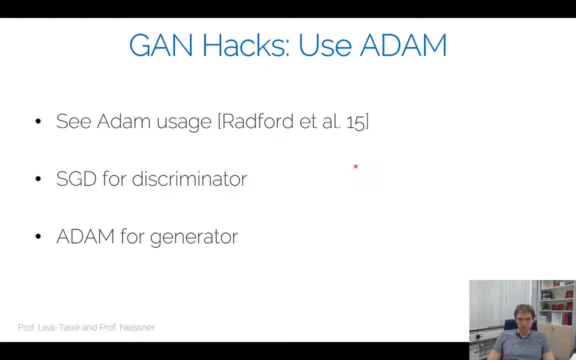 This is the standard thing. I don't know. You see this very quickly, based on the training curves. If the training curves don't look good, you can change stuff here. That's the first thing I would always do: Check your training curves. 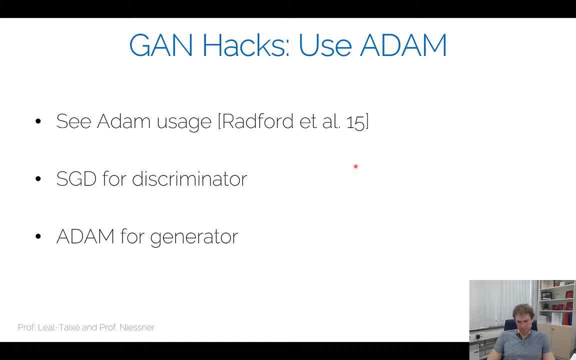 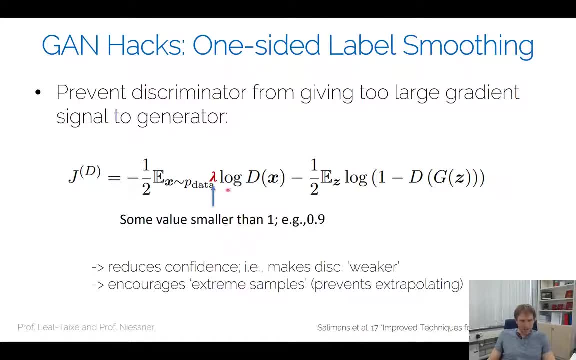 And you see this after a few minutes. basically, One thing is one-sided label smoothing. That's an easy one. You can say in the discriminator, right, Like for the real samples. you just penalize that part a little bit, Right. 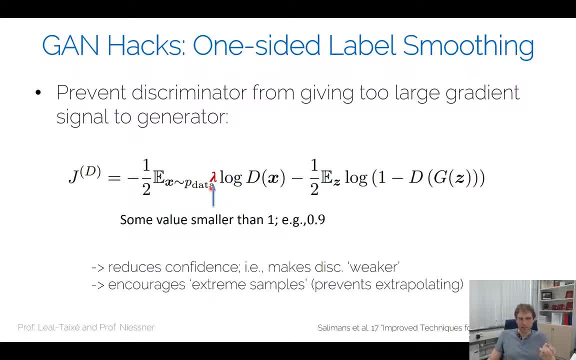 So you have a lambda function here that makes the discriminator here a little bit weaker in terms of the confidence Gives it like 0.9 or so. Yeah, this encourages a bit more extreme samples, Which is good. Right, It doesn't always try to be on the safe side. 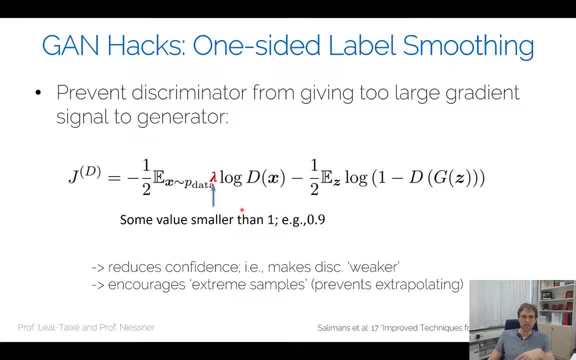 So it makes this part a little bit weaker. So it reduces the confidence here of the discriminator, Which is good By confidence, right? Obviously, what you're getting now your score functions for the real images will just be a little bit lower. 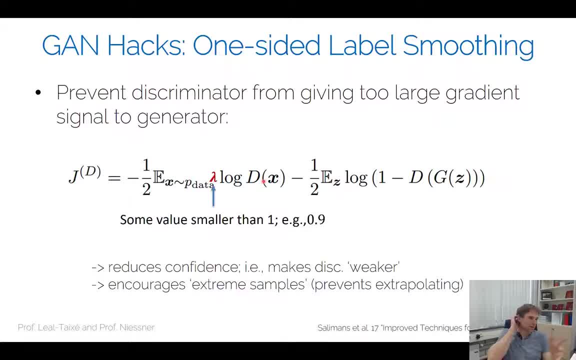 That's all you're doing here. This is this one-sided label smoothing. This one works reasonably well. Can't do it too extreme. of course. 0.9 is a reasonable number. here what people use Seems plausible. Another thing people do is they use historical generator batches. 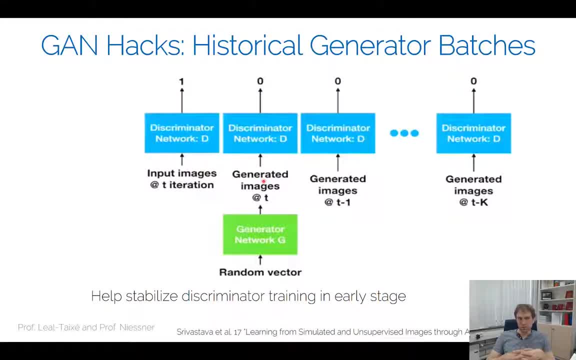 So What you do is you have a discriminator network and a generator network, Right, And what you can do is you can generate stuff over a history of iterations And you can just mix your generated samples in the current batch So your discriminator will see not just the results of one discriminator. 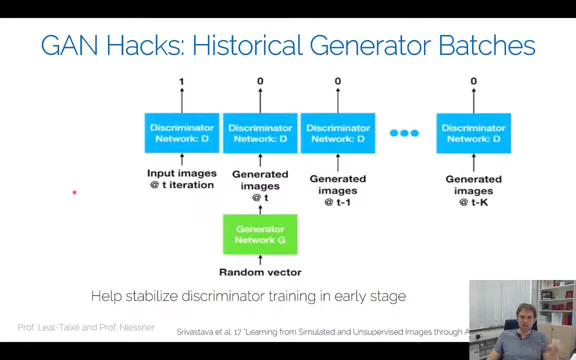 So it will basically see discriminator samples from multiple iterations, Especially at the beginning. this is very important. Well, it's not important. It's a very good idea Because you will actually stabilize the discriminator a little bit right. It's not so heavily overfitting to one type of generator. 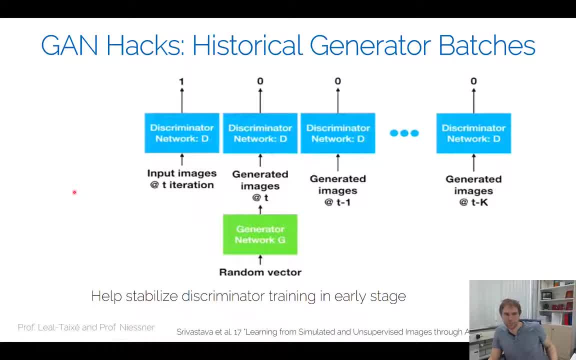 But it's spreading it a little bit out. So it's learning kind of distribution of a specific generator, But learning a distribution of all generators- Well, not all of them, but the last N or something like that. This is a relatively good idea. 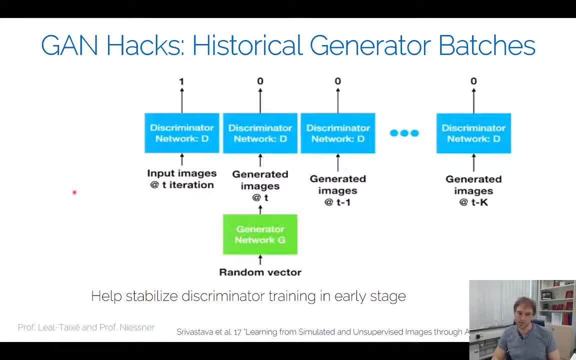 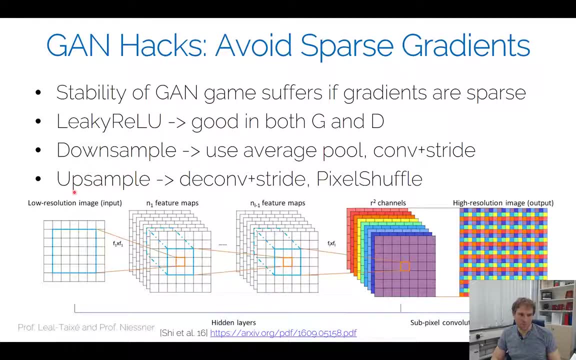 It's an easy implementation And it seems to help quite a bit at the beginning. Another thing is sparse gradients. Stability of the GAN game suffers from gradients of sparse. That makes sense. That's the same thing for every other neural network right. 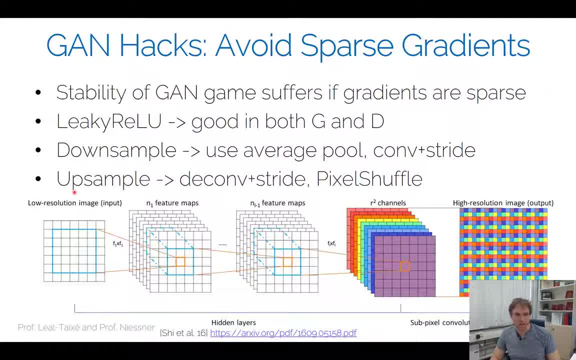 If you have no good gradients, you're kind of screwed. Leaky reloads is a thing that people often use for both generators and discriminators. I've also seen parametric reloads. actually, Leaky reloads seems to be a good compromise, what people use. 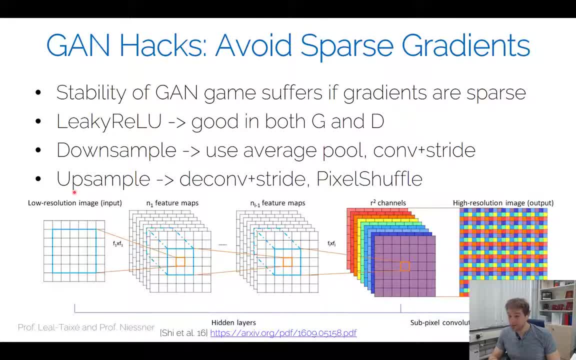 Still, high-level advice is: just use DCGAN to start And then once again. once you get this one to train, then you can play around with these things. This one will not make or break it right away if you have a working architecture. 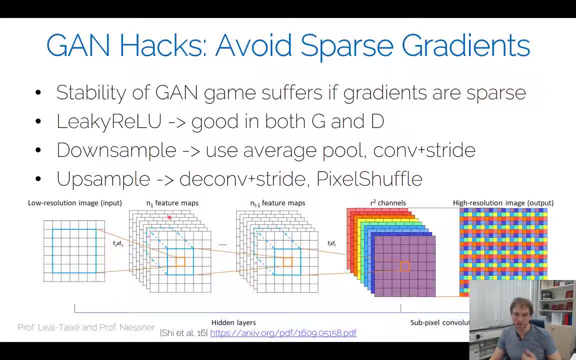 Downsampling: use average, pooling conscious strides. Upsampling: use the conscious stride And so on. There's things like pixel shuffle you can do. It helps a little bit. But yeah, I mean, this is something you can actually debug. 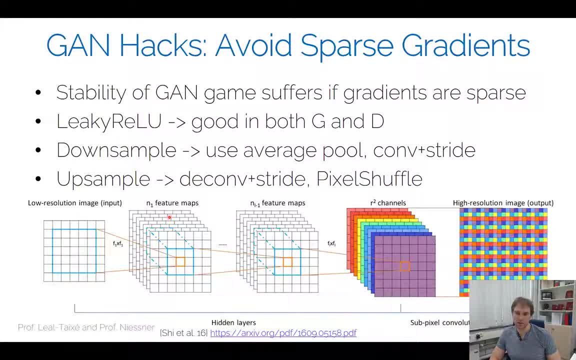 You can go ahead and literally visualize your gradients, right. You can see how good your gradients are. If your gradients go crazy, then something went very wrong. This is something you should be aware of, But you can see that actually, right. 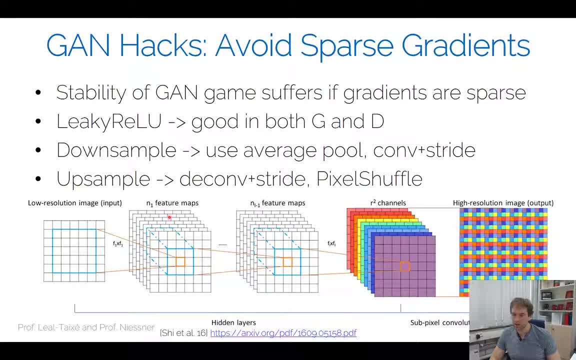 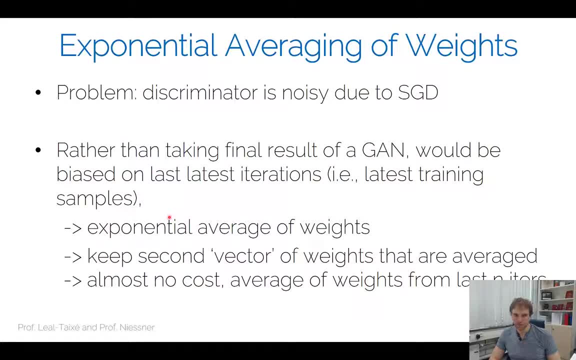 You can check your gradients. If they go too crazy, then it's a problem, And you see this also relatively early on. Another idea is exponential averaging of weights. One problem is well discriminator: can be noisy due to SGD, which makes sense. 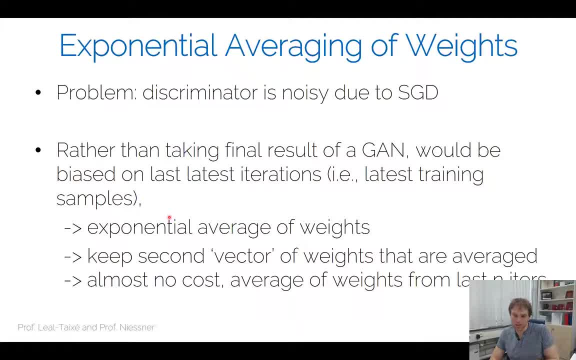 The problem is what you have at the very end of your training process. You're going to have a lot of impact from the last iteration right. There's a lot of noise there. So one thing people do is they take basically an exponential average of the weight of the neural network. 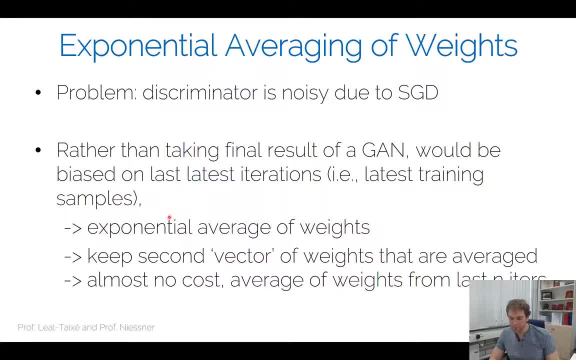 So what I'm going to do is I'm going to store- Let's say I'm going to run my network for a million iterations And I'm going to take my network and take an average of the last 100 iterations and just average the neural network weights. 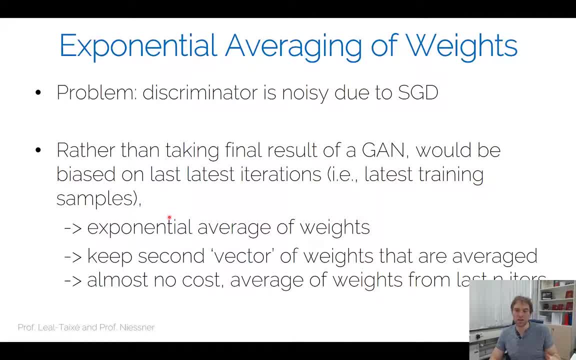 And you can of course not just do a simple average. You can do an exponential average, You can compute this running average while you optimize it, And this is very good at the end, because then you don't have these outlier samples anymore, these noisy things. 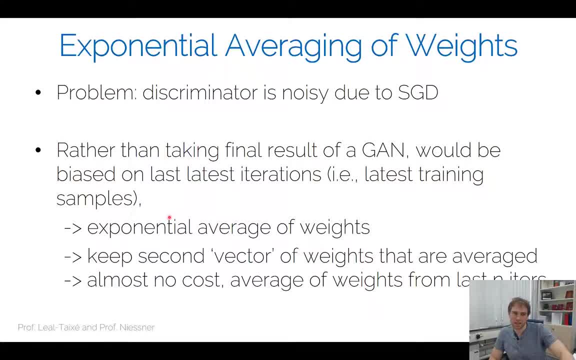 So you kind of want to avoid this bias towards the last iteration. And this exponential average is easy to implement. You just keep a second vector of the weights around. You just have one update there. Almost no cost Helps a little bit. This here is not helping your training too much. 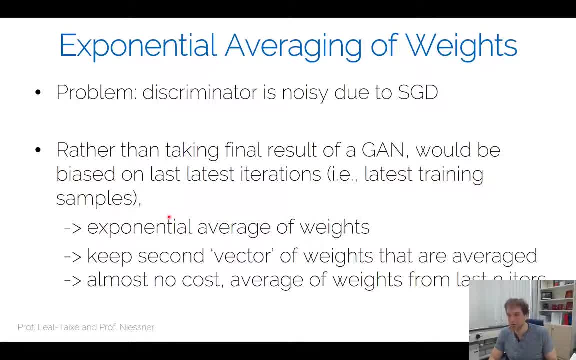 But it will help you. It will help your overall results potentially a little bit. It's not going to do a major leap, But it's still a good idea for your final deployment. Okay, So these are the things you can play around with. 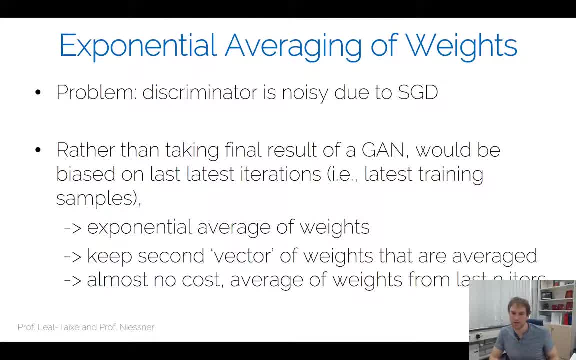 I gave you a lot of options. There's no guarantee that one or the other will fix or make or break it Right, But at least you want to have a bunch of options, what you can play around with. What I could always recommend is start very simple. 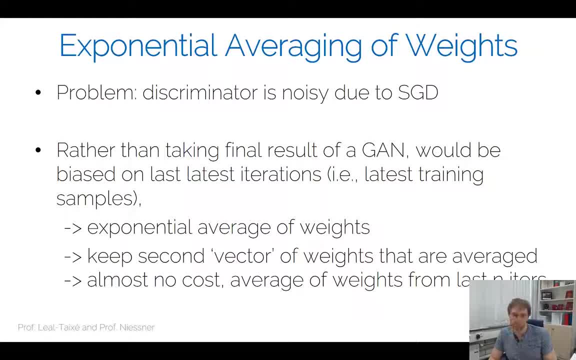 Have a simple architecture like this again. Try it out in MNIST first, Then go to a cell of A, Play around with that and see how your GAN behaves. Now I still want to introduce a bunch of objective functions of the GANs. 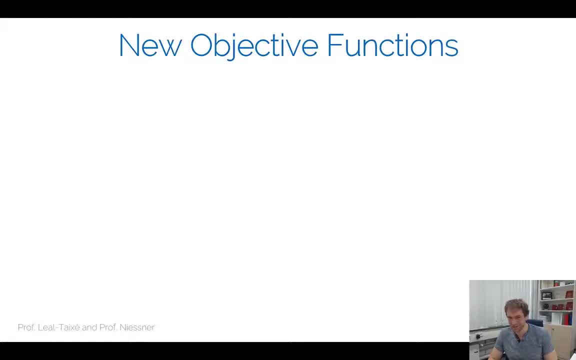 There's a couple of. Actually there's many objective functions in GANs. I'm not going to go over all of them With the caveat right now that don't change the objectives too many times. Typically just use the heuristic method. That's a good idea. 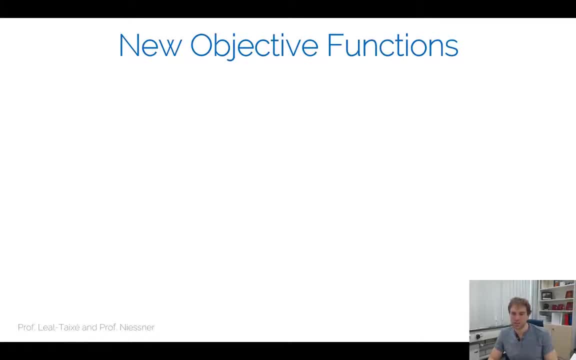 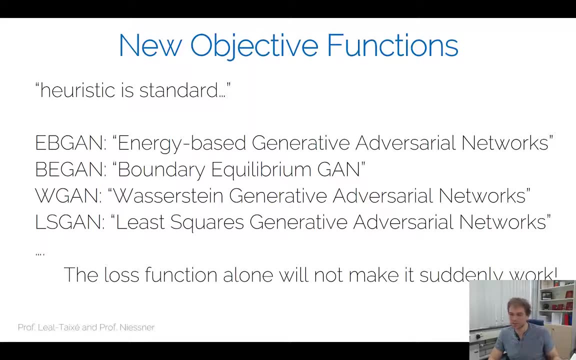 I want to show you the implications of changing the loss functions. But most of the time your GAN will not just suddenly work because of a different loss function. I mentioned heuristics as standard. That's the easiest way. It's not necessarily standard for deployed networks. 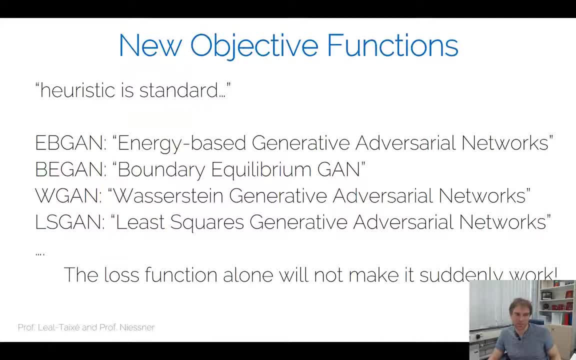 But it's something you can always start with. I want to go over a couple of them. One is EBGAN, BEGAN, WGAN and LSGAN. The loss function again alone won't make it work. I want to quickly go over these. 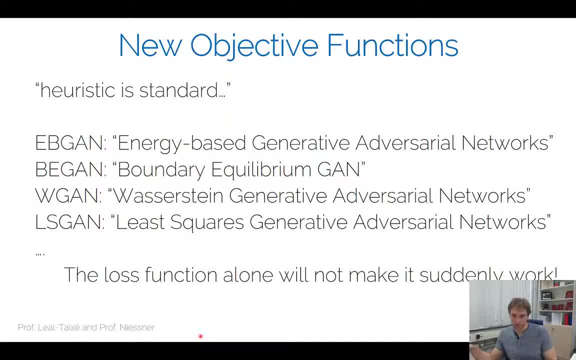 I would encourage you have a read afterwards at these papers. I might go a bit quickly over it. I don't want to spend too much time on it, But I think it's interesting when you read these papers what people thought about their insights. 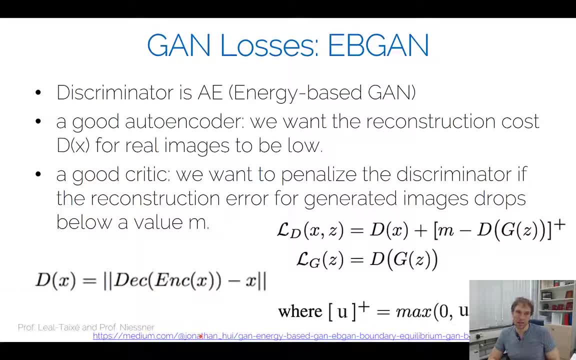 Let's have a look at the EBGAN paper. The EBGAN paper is basically EB stands for Energy Based GAN. The idea here is the reformulating the discriminator. So basically they're saying: my discriminator takes some sample X And the idea is: 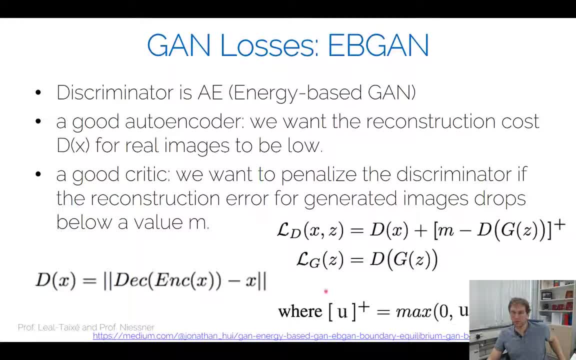 I want to reconstruct this image perfectly. This is just an autoencoder formulation. My discriminator says: I want to have a good autoencoder function. This is what my discriminator is going to do And I want to, basically for real images. I just want to say I have good reconstruction. 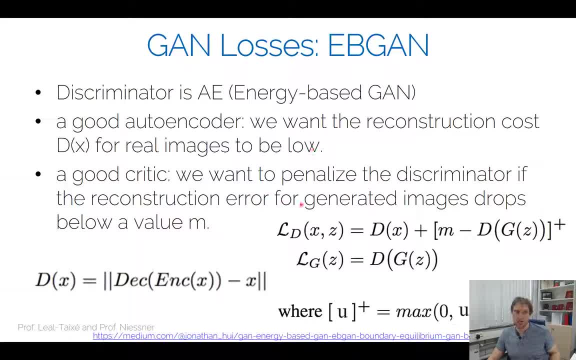 That's it, Autoencoder. We want good reconstruction. Now, what we're doing is We want to say, if we're having a good reconstruction here And we pre-trained this guy, Then if it's a good reconstruction, Then it was a real image. 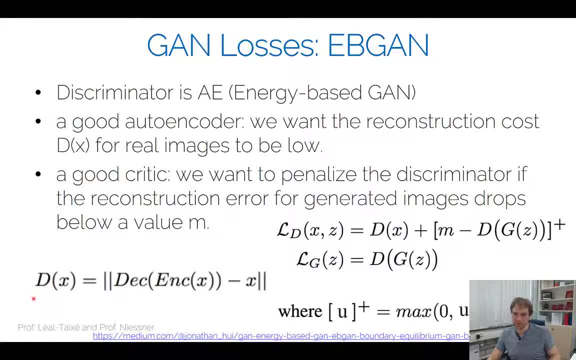 If we have a good discriminator trained on real images here And we're feeding a new image in And it doesn't have a good reconstruction, Then it's not a real image because it wasn't reconstructed well. That's kind of the high level idea. 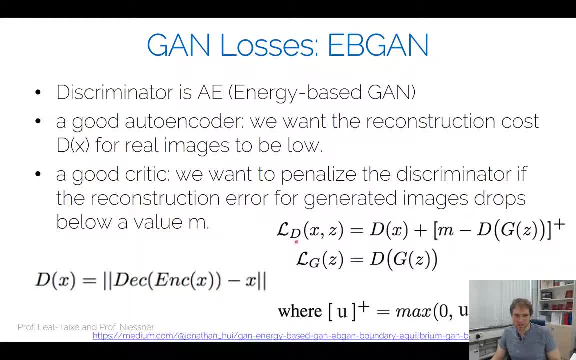 And the way you do this is you simply say: Well, when I'm training the discriminator, I'm feeding a real image and a fake image Or a latent code in there. Well, let's start with the generator first. So generator gets latent code. 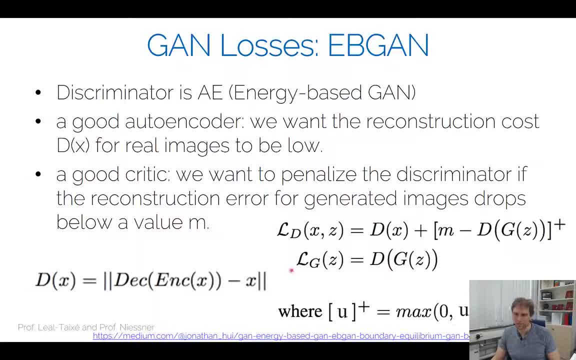 Generates image, It's being fed into discriminator Going to optimize for that function. The generator tries to make sure that In the same way the discriminator could reconstruct stuff, In the same way you could reconstruct stuff with the generator. That's what I'm saying. 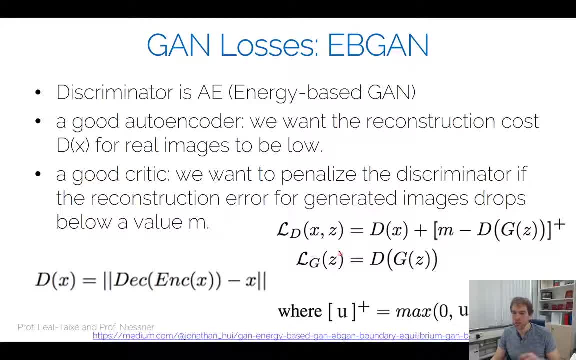 There should be no difference in the reconstruction quality, If it's a real or if it's a fake image. The discriminator, however, Now says: Well, I'm going to train the discriminator. That's this part. That's the first part of the loss function. 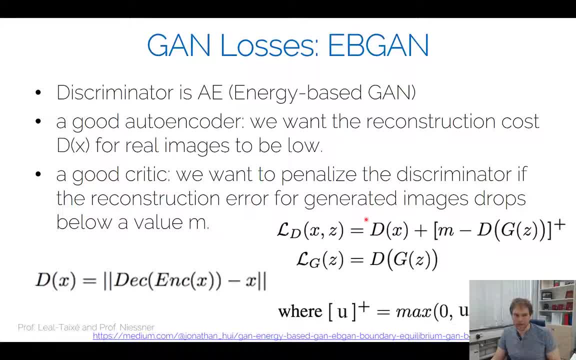 And now I'm going to say I want to penalize the discriminator If the reconstruction error for a generic image Drops below a certain value. So I'm just going to penalize it and say, Well, okay, look, I want to drive you apart. 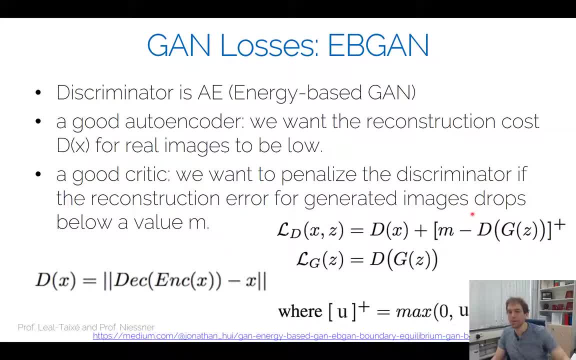 I want to say You were a fake image. You should not be well reconstructed. But I'm only going to do this up to value n. That's kind of what the eBegan is doing, Right? So I'm not going to train these two jointly. 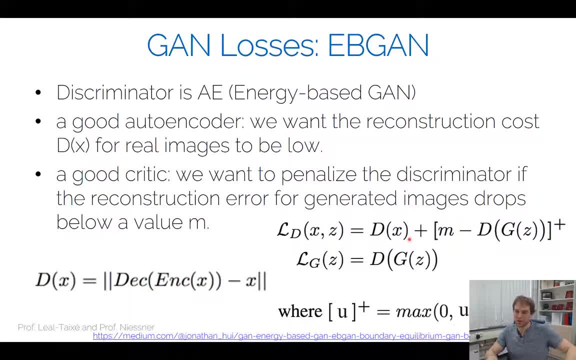 And hopefully I will drive these two apart. I will get a latent encoding for real, I will get a latent encoding for fake, And the idea is, If I train both of them at the same time, My generator will figure out how to move them together. 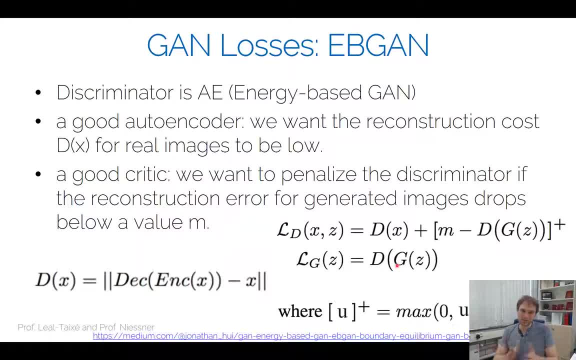 And the discriminator tries to move them apart. So we're trying to get these latent spaces Separated out, Or together, Depending on whether you discriminate or the generator. It's a little bit reformulated. Beegan Has a similar idea on that. 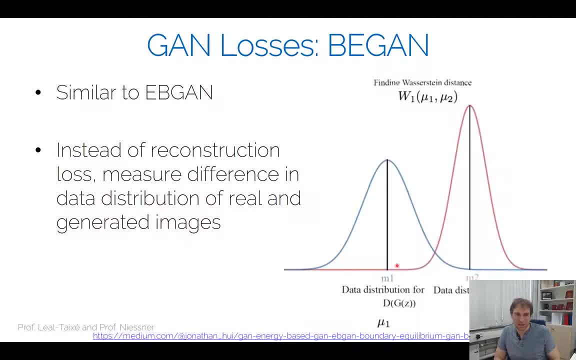 So Beegan Is similar than eBegan, Except Now, instead of reconstructing a loss, We measure the difference in the data distributions of the real and the generated images. In other words, we're going to go ahead And we have a real distribution here. 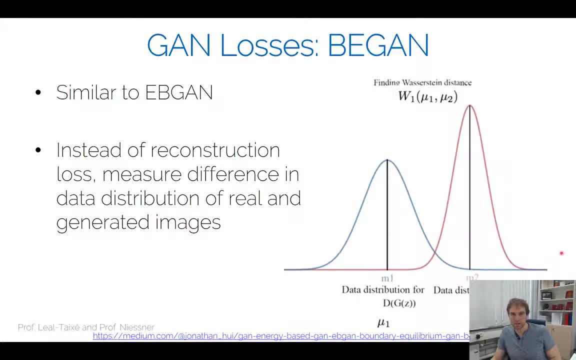 We have a fake distribution here And we're trying to measure the difference between those two. There's various ways of measuring these differences. A very common way- what people are doing- Is looking at The Wasserstein distance or the Earthmovers distance. 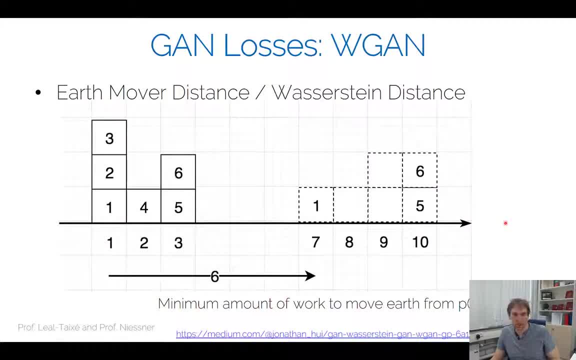 Same terminology And this is this W again, Which is essentially It follows out of that. The idea is: I have a distribution here, There's a bunch of blocks, And I want to reorder these blocks And move them from here to here. 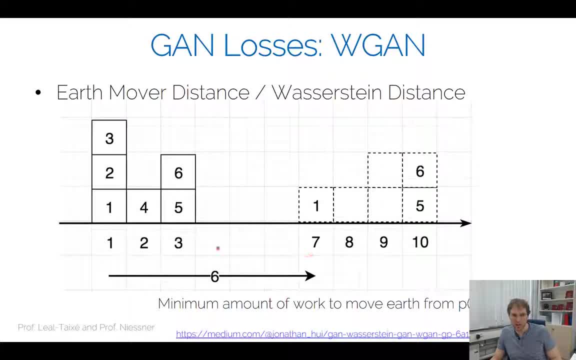 So I have a distribution P And I have a distribution Q And I want to figure out How different are these two distributions? And this Wasserstein distance Tells me how different. they are Right, And how different are they. Well, I want to figure out. 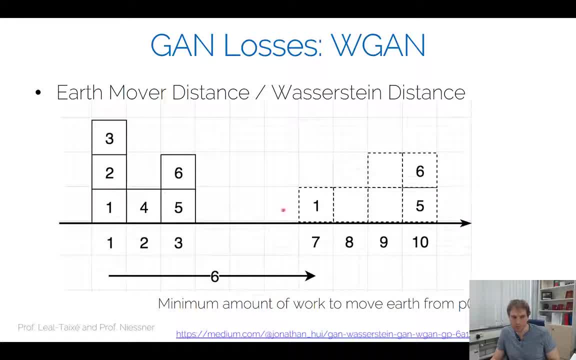 How much work do I have to do to move this one from here to here? This is: I have to move this block from here to here. six: Moving this five from here to here Costs also some work, right? So everything you're moving from here. 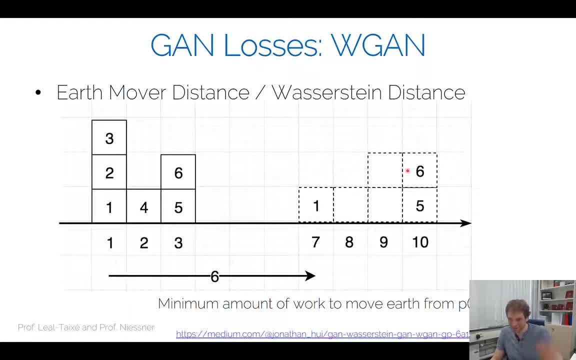 Moving the Earth from here to here Costs you some effort And That tells you how different. If I have n samples here, I have n samples here, I can figure out how different are these two distributions. This works for discrete cases. 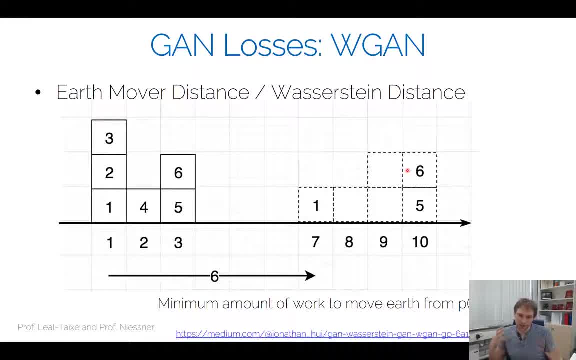 You can formulate it on continuous cases too, For the sake of the theoretical framework. here We're going to think about continuous distribution, Right, But it measures the difference between these two distributions. One slight problem here is: This is a very costly operator. 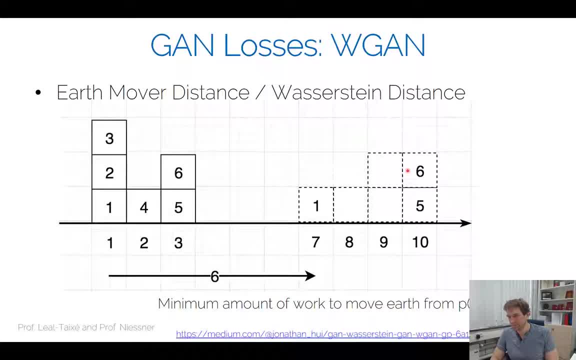 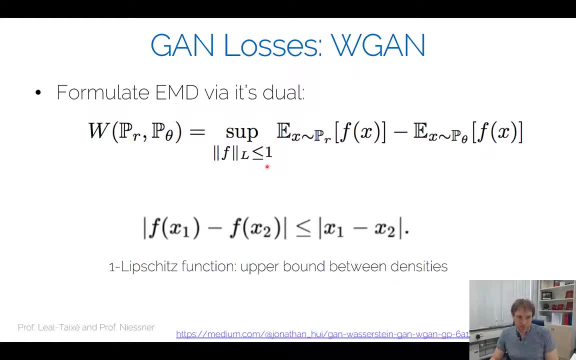 Right Computing Wasserstein distance Very, very costly. There's a few ways how to reformulate this problem Right. What you can do is You can say you have these, You have a function f You want to figure out. basically. 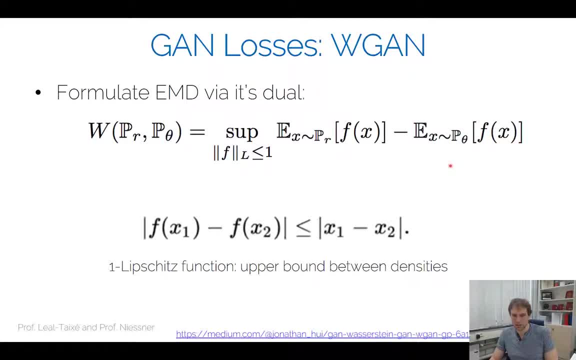 Samples from one And samples from another distribution And you want to figure out what the difference here is. And the EMD, The Earth-mover distance, can be formulated As the supremum Of the difference between these two functions. Sorry. 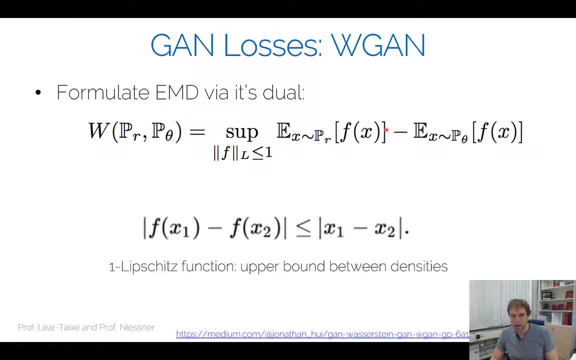 Between these two different distributions And This one, however, Only holds If this function f That we used for the sample x Is one Lipschitz constant. It's a one Lipschitz function, By the way, If you go over Lipschitz. 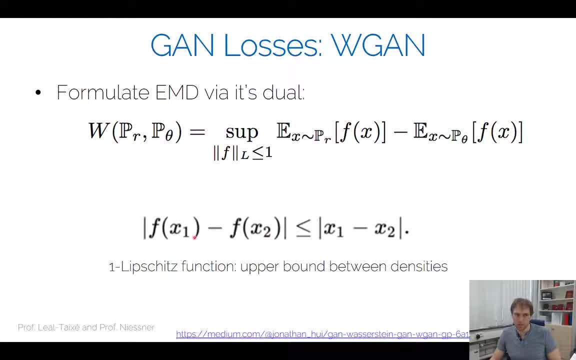 Lipschitz means If you have the difference between the two functions Between x. So if you have one function f, You're feeding in x1 or x2.. The difference between the function values Is smaller Or equal in the difference. 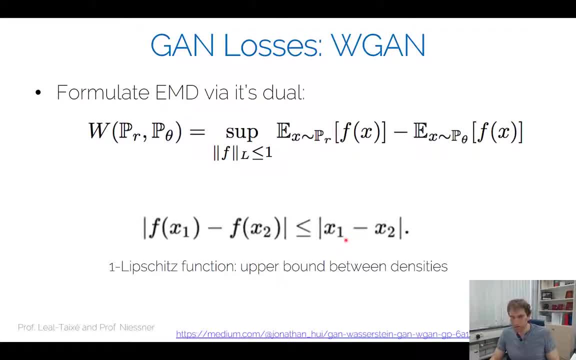 The absolute difference between The parameter values you fit in. So it's an upper bound between the densities. I'm not going to go into detail How this one here is derived. This takes a little bit more math. You just have to believe me right now. 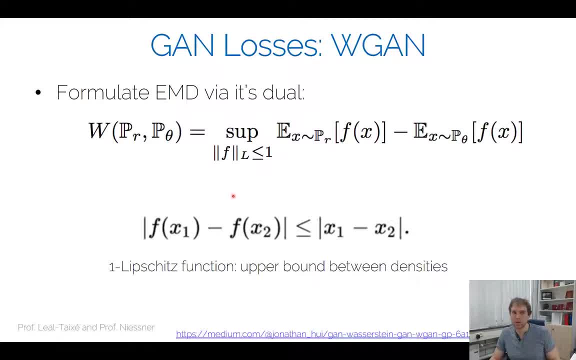 Taking that estimate here, The supremum Will measure. It's basically the dual Of the Earth-mover's distance, And this is something we want to look at And The challenge what we need now is We need to find a function f here. 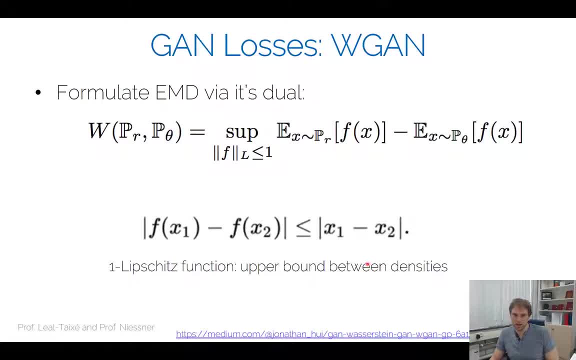 That fulfills the Lipschitz constraint And f, in this case, Is a critic function That tells us the quality of x. Basically, The sample is from P- R And the sample here is from P- Q, And we want to figure out. 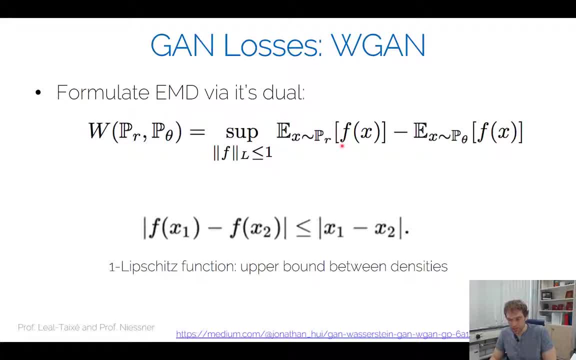 How far apart are these guys? And What would be nice If I had a critic that would tell me this right away, If I had a critic That told me this for every sample of the distribution. And here I have a critic. 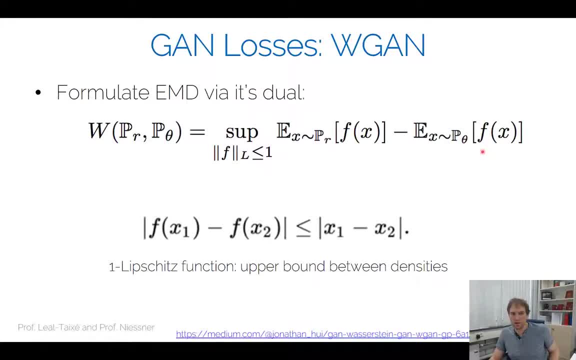 For every sample of this distribution And I'm getting the Expected values Of the difference here. Then I would know how close my distributions are. Now The problem is, This function is very hard to define Because, let's say, I have a bunch of images. 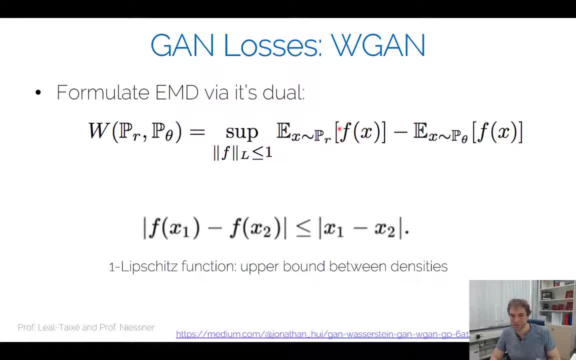 Who knows how close The distributions between these images are. I can do this on a per pixel basis, But computing this earth move distance, as we know, Is very expensive, Especially if you have a bunch of high resolution images. So we do what we always do. 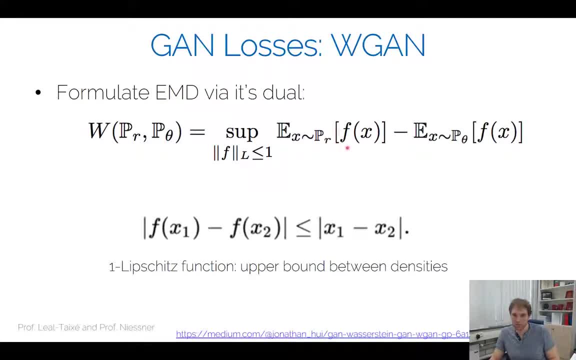 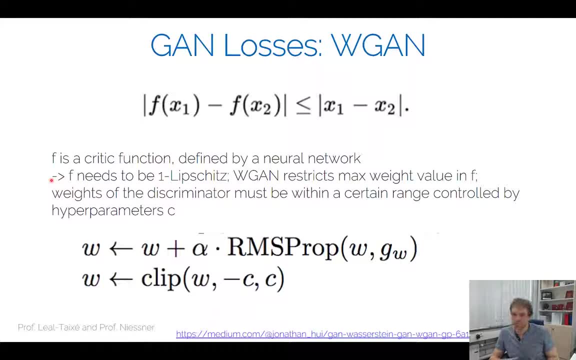 When we don't know it. Simply, we learn this function f, So we're learning this critic function, And In this case, f is a neural network, Because we want to learn that function. We don't know it right, So we have to make sure. 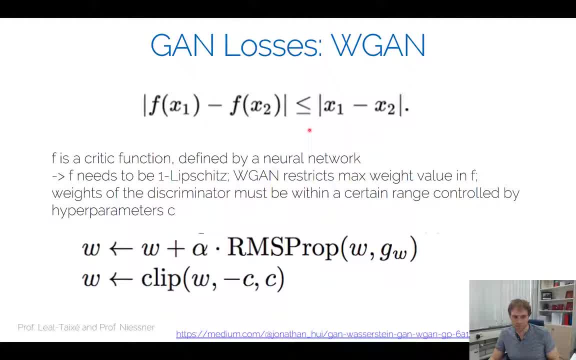 We don't violate this one Lipschitz constraint, So f needs to be a one Lipschitz constraint, And in the optimization process We just have to make sure That this Lipschitz constraint is not being Violated. So what we do is: 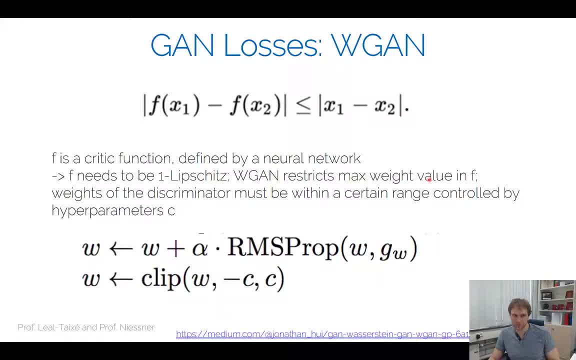 We restrict the maximum weight value in f, And the way we do this is The weights of the discriminator. We just control them By a hyperparameter scheme, And this is called weight clipping. We just say, Oh, my weights can't get closer or smaller. 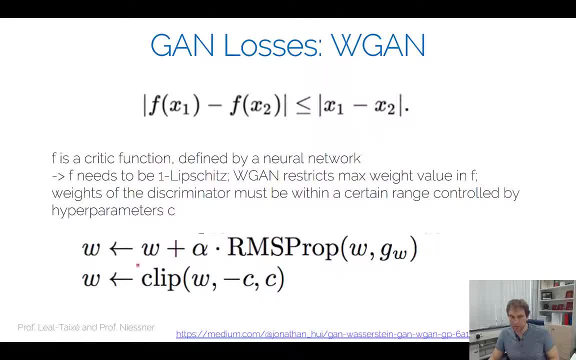 Than minus c and plus c. So we just restrict The function values basically. So we have a Lipschitz estimate with c. If I'm taking a bigger c, Well then I have, Then I'm more loose If I have a smaller c. 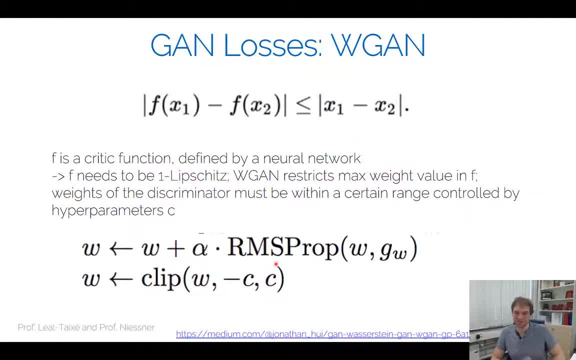 Then I'm more tighter And we go into this a second What this means. if you have a smaller and a larger c, Okay, So this is controlled by this hyperparameter c And the weights are still being updated Of this critic function. 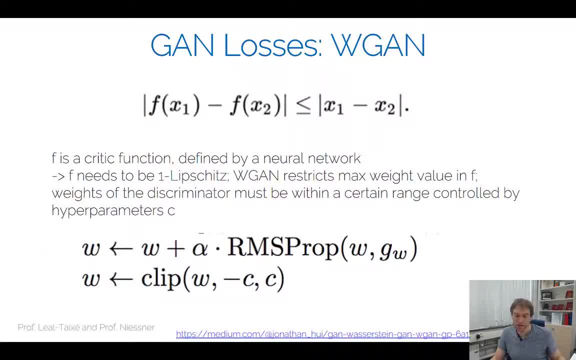 Again, this is just for the critic here. This f will become a critic function. Or is a critic function? now That we model at the neural network, We want to optimize the parameters of the neural network. By having rms prop, We do clipping. 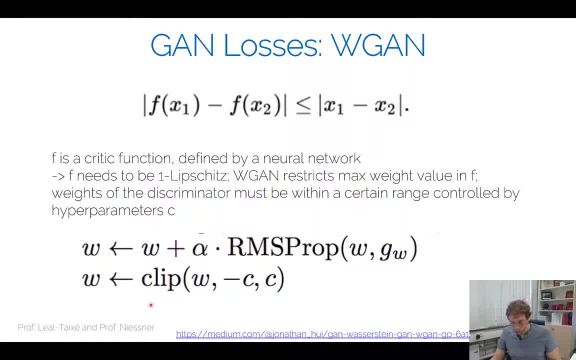 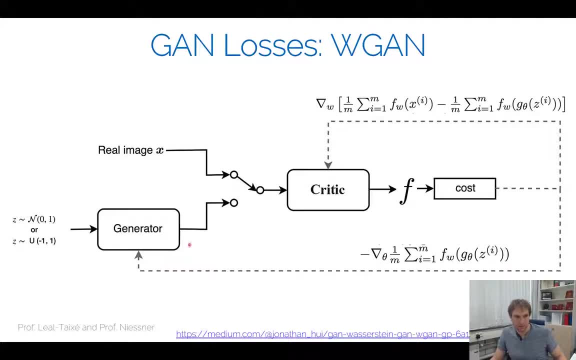 And What we're optimizing now is We're optimizing both the generator And a critic, And this is what's happening here. So here we have: We have a generator, We have a critic And the critic is trying to measure. 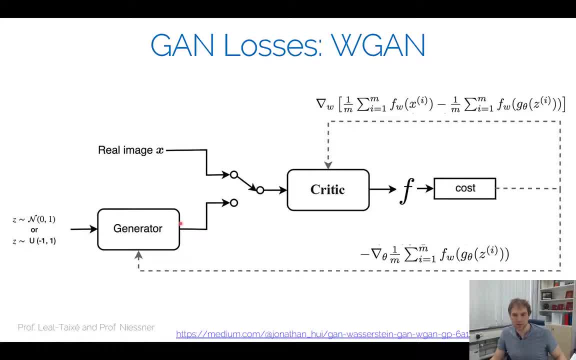 The distribution, The distance of the distribution From the generator And from the real images. Again, this is our function, that we have This supremum that we're optimizing for. Again, quickly going back, That's what we're optimizing for, So we're just taking a discrete number of samples. 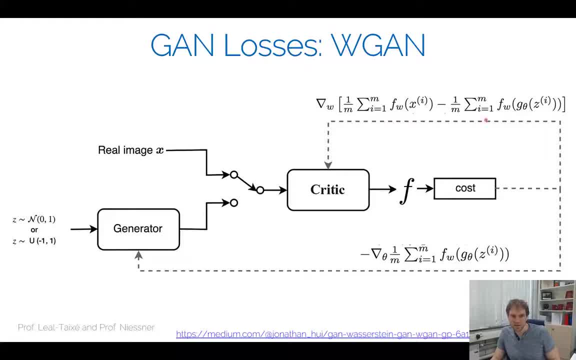 Which is m samples. here We want to make sure The distance between these two Is going to be minimal. At the same time, we have to optimize for f, Because f doesn't exist yet. f is a neural network. I don't know the function, how to. 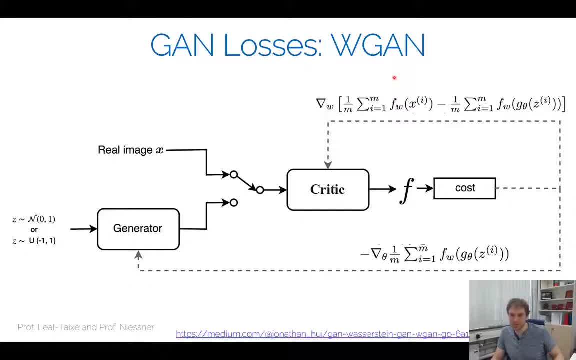 How to compute the earthmover distance between my samples. So I have to jointly optimize for both. The critic that tells me How close are the distributions, And I have to minimize the distance Between the two distributions. That's what Wasserstangen is doing. 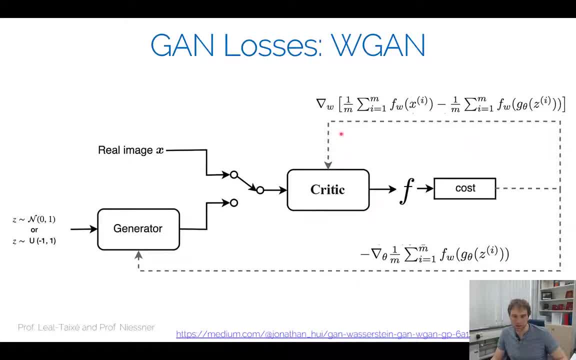 What we do here in practice is: We have here: We have the function f. Here's the real sample. We have the function f And here's the fake sample. Again, in order to optimize Our generator, We're optimizing these two together. 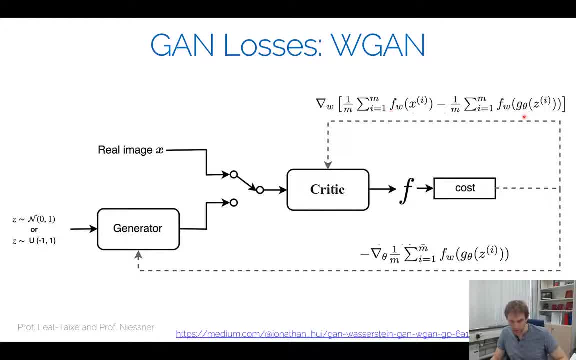 We're computing the gradients Of f and g- g has also weights- And at the same time, We're trying to make sure That we're getting a good critic function. If you're comparing this to the standard GANs And the reason why I'm going over the Wasserstangen GANs, 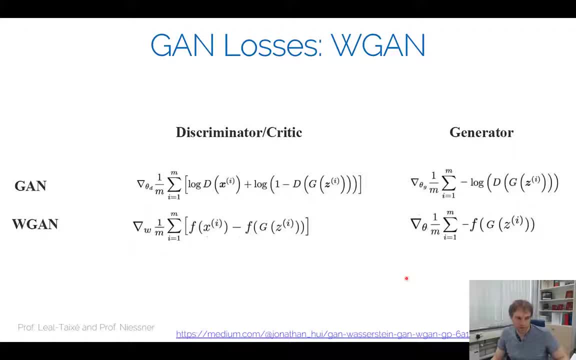 Is just in practice. If you're comparing this to the standard GANs, We're having here The GAN formulation. The GAN formulation, We had here The gradients here for For the discriminator was the binary cross entropy. Now, what we have 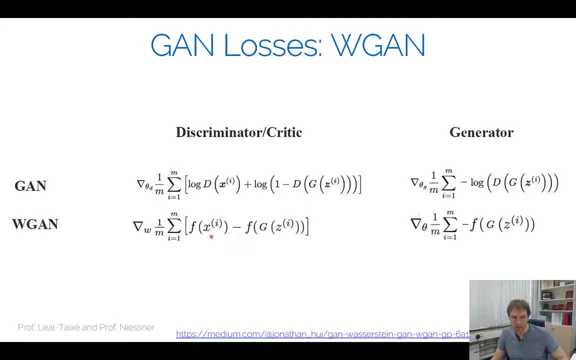 In the Wasserstangen for the discriminator. Is this critic that measures That uses a critic function? Tells me what is the difference between these two distributions In the GAN formulation For the generator? Well, I had this For the discriminator: log likelihood. 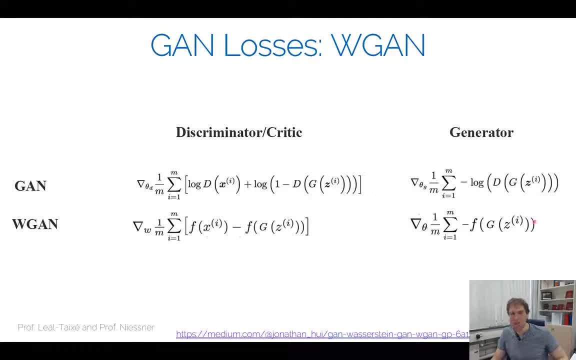 I basically want to make sure my generator produces stuff That the discriminator doesn't recognize, And here I have gradients that That optimize For f, Meaning that I'm basically saying that My critic tells me It's a good distribution. 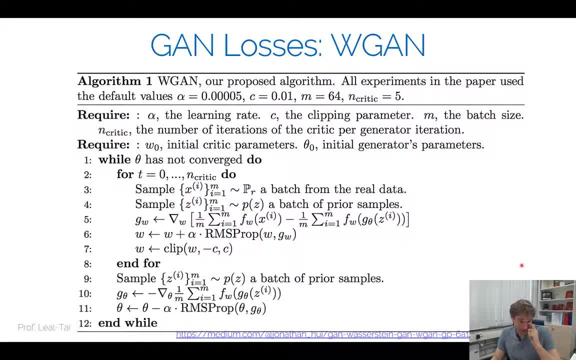 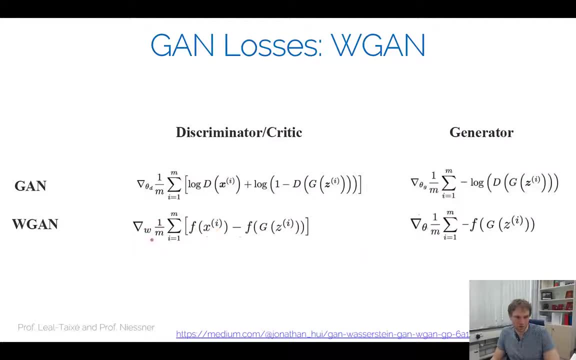 If you're optimizing that, You will get something like that. What do we get? We get a loop, Let's say, while we're not converged, And conversions will become a new meaning now Because, like here again, We're optimizing for this critic here. 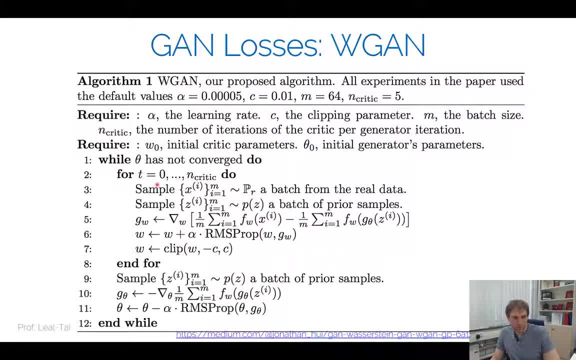 And Now what we do is We're optimizing for the critic. We're basically drawing samples from real data. We're drawing samples, We're generating samples with a latent vector z. We're optimizing the critic here, Right, And We're doing the weight clipping. 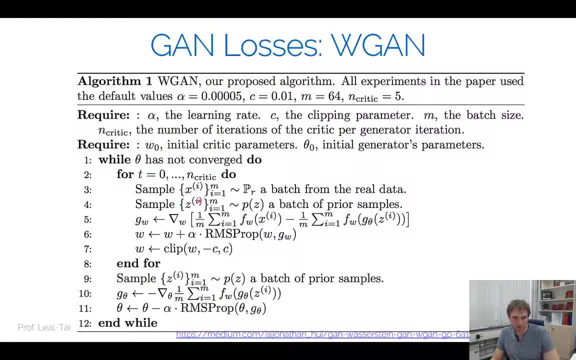 We do this a couple of times. Our estimates for f gets better. Then we sample from real And we're trying to make sure our gradient Generates stuff That with this current function f Can be distinguished From. Sorry, the critic says. 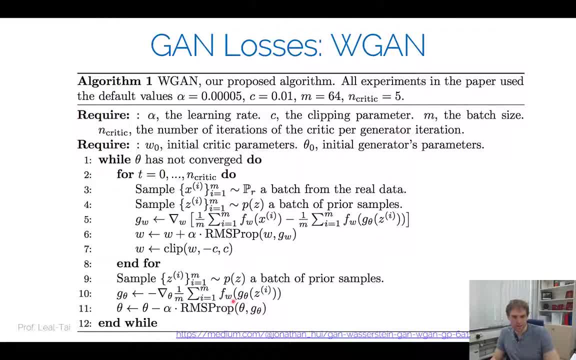 It's a good estimate, Right. And then you go ahead, And then you iterate. These guys set critic to 5. So this loop runs 5 times for critic optimization, And then only one: generate update. Critic update. generate update. 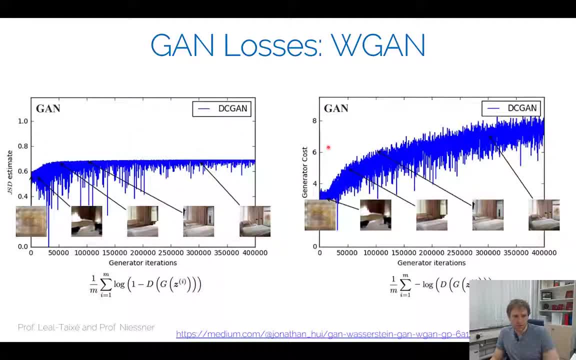 Okay, If you're looking at the GAN losses, You remember we had GAN losses That kind of stabilized like that, And we had this issue that it didn't- We didn't know when it converged. The nice thing about the Wasserstein GANs now is: 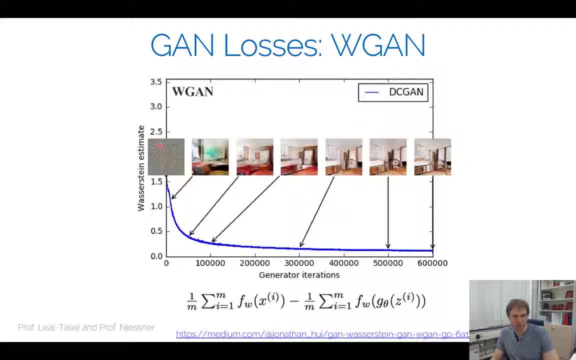 We're getting curves that look like these, Meaning that It goes down. actually, And why does it go down? It just means that this estimate here for the critic Is getting better and better. So, basically, having a good critic function f That can estimate the distribution between these two. 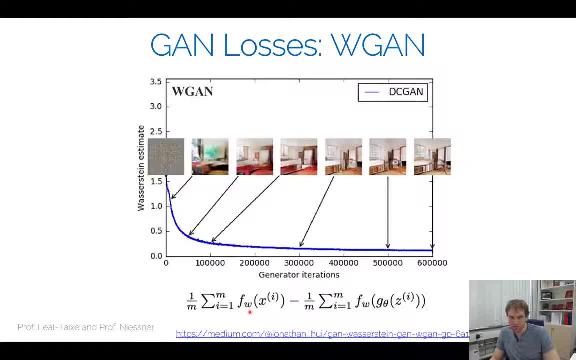 Set of samples, And this is being very small. This is our loss function. by the way We're plotting here, If this Wasserstein estimate becomes good, Then in principle, Well then, my two distributions are the same, And that's very nice about the Wasserstein loss. 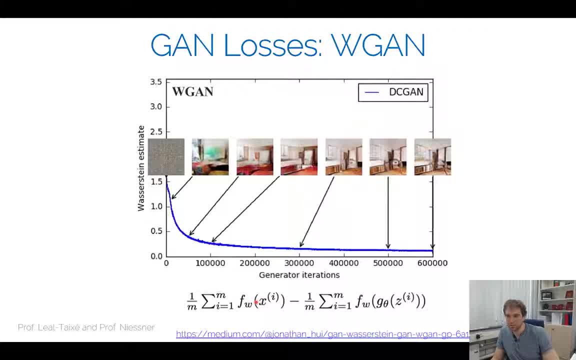 Is that it actually has a reasonable, A reasonable convergence plot. So my images At the beginning look bad And then they eventually look better and better. So that's the problem with the Wasserstein architecture here Only replaced with Wasserstein loss. 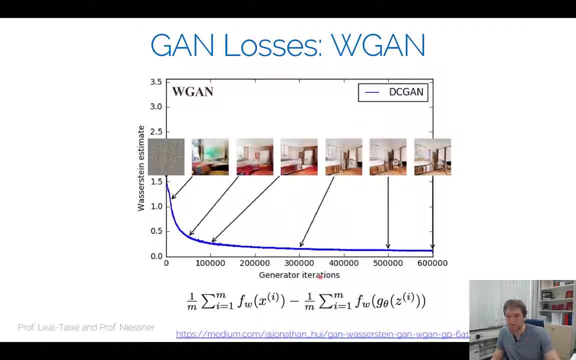 I'm not saying here That Wasserstein produces necessarily better results. There may or may not. There's a lot of discussion about that. But what I'm saying is It's very nice to look at the loss curve here, Because it actually goes down. 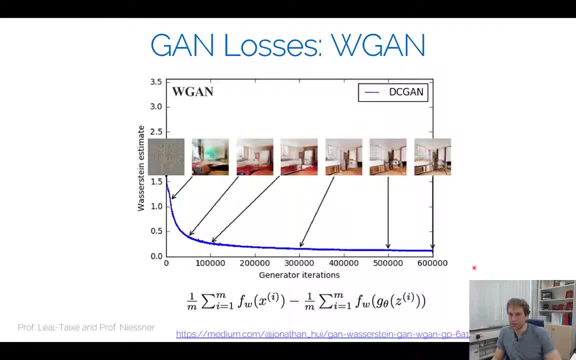 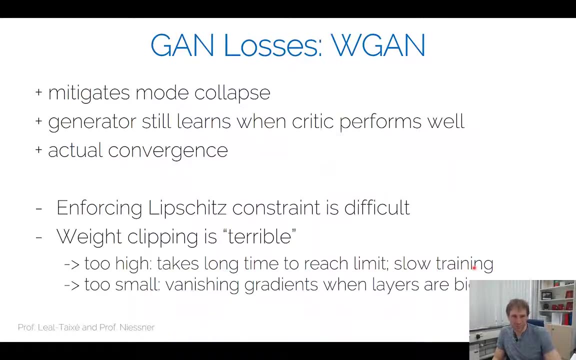 I mentioned this before: Wasserstein loss, Wasserstein GAN Is one of the things people do actually use a lot. Yeah For GANs. So either heuristic or Wasserstein. The other two maybe not, But this one is a very popular one. 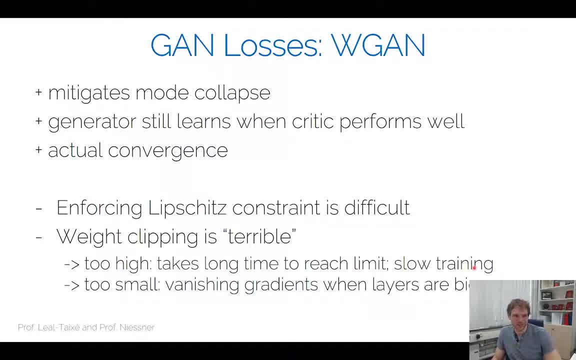 Wasserstein: GAN is great. Now we see what we're doing. So we have actual convergence. In theory, it should mitigate mode collapse. You can argue about that. Generator still learns when critic performs well. These two, they're not. They're not. 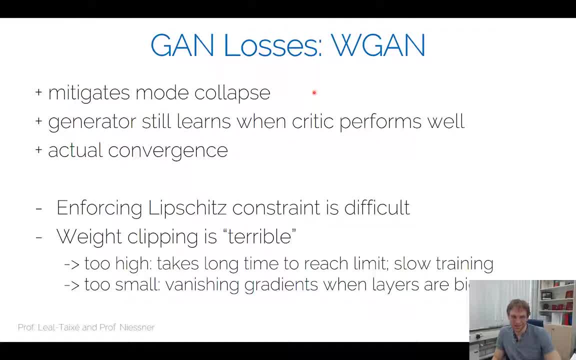 They're not necessarily competing. They are on the same side. One problem is This: Lipschitz constraint is difficult. Weight clipping is a dirty, dirty hack. This is not a good idea. There's a couple of variations Of whatever gradient penalty and stuff like this. 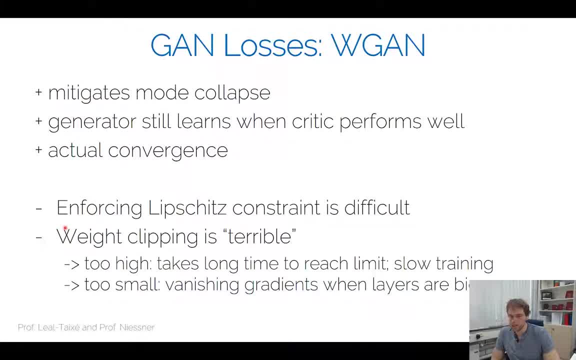 That people use. Weight clipping is not the best idea ever. If it's too high, It takes a long time to reach the limit. Basically, if you're allowing for too much of a variation, This Lipschitz estimate is not very good. 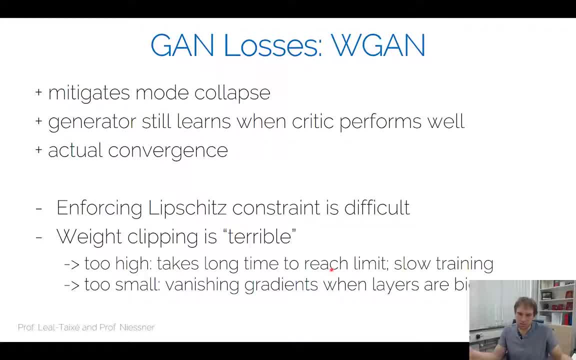 Because it's too loose. That's what we're doing. If it's too small, We often get weighted vanishing gradients Because we don't learn anymore. Especially when you have big networks, That's a big issue. Either one, you don't train a lot. 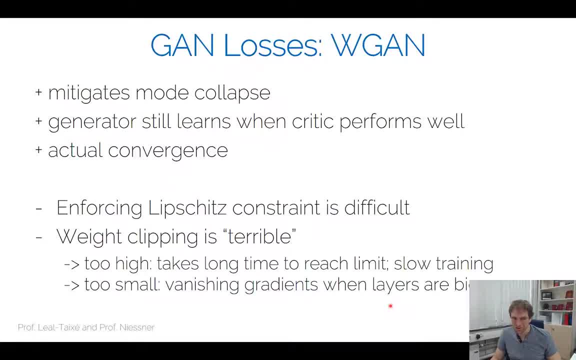 If it's too small Because my weights are being too small, Or my weight changes are being too small, Or if it's too high, Then my Wasserstein estimate is bad. Either one. These two are problems. Fixing the C parameter: here is a problem. 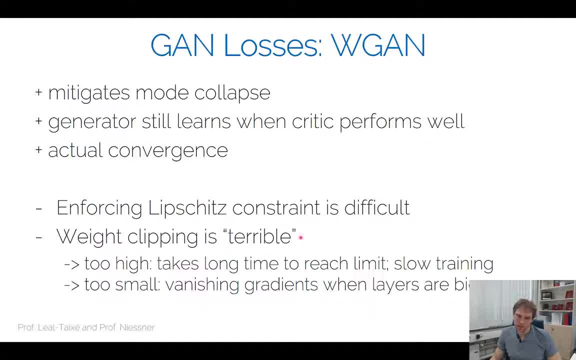 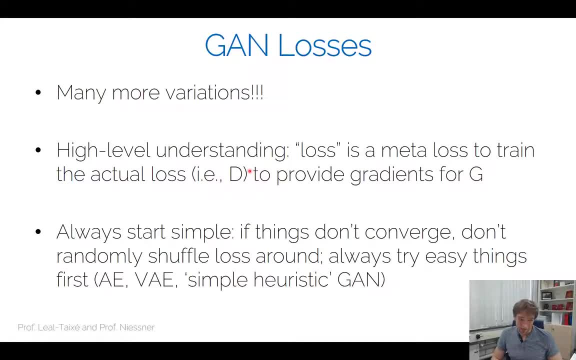 There's a couple of variations now, But this is a challenging task For the losses. There are a lot of variations of GAN losses. There's a high level understanding. There's a high level understanding in meta losses, Training and stuff like that. 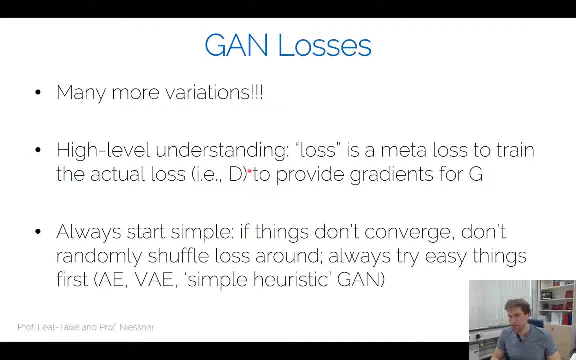 The practical thing is that D provides the gradients. D is our learned loss. We're motivated at the beginning. D is the learned loss that we use in order to train G, But there's many variations of that, of course. My recommendation is always: start very simple. 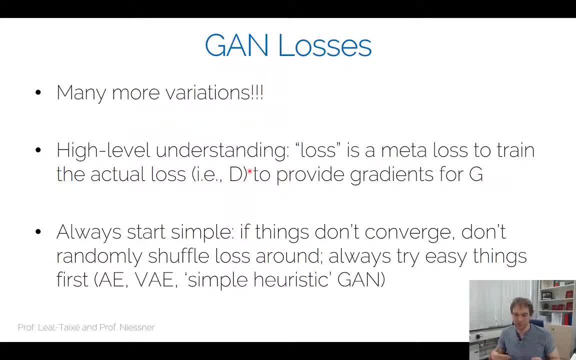 That's always my recommendation. Dividing concrete is key. We want to start simple, Get simple stuff to work And then we make things more complicated. Always start simple. If things don't convert, Don't randomly shuffle the loss around. This is what I've seen, unfortunately, many, many times. 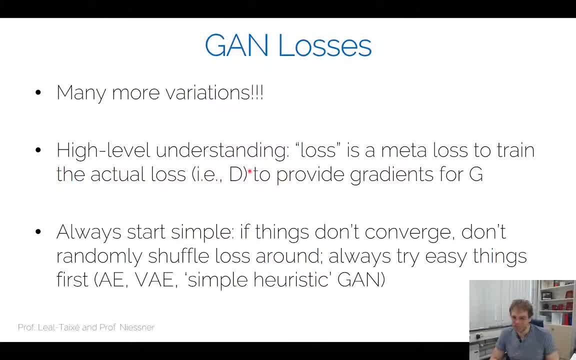 Changing the loss is the last thing you should do. I would always start with the heuristic first. That's the easiest one, Maybe Wasserstein, But that's about it. I've seen people trying to do 20 different losses. None of them worked. 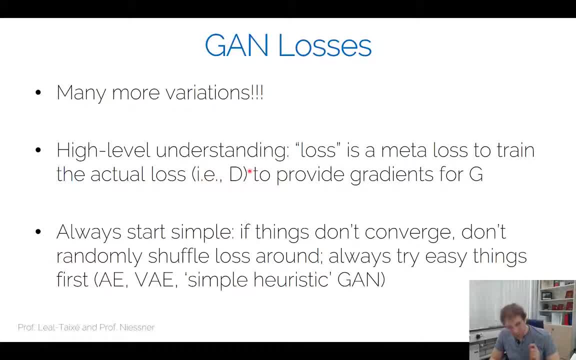 And they spent a lot of time on it. Always start simple. If you're doing GANs, I would always start simple. I would start with an autoencoder first, Without the GAN. Get this architecture to work. Use a variational autoencoder next. 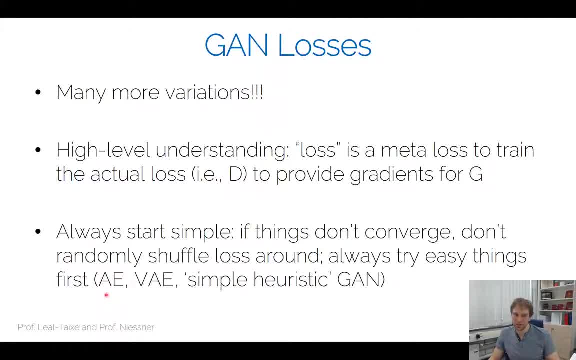 And then use a simple heuristic GAN And then you can compare the results of the autoencoder with the variational autoencoder and then with the heuristic GAN. This way you have a direct comparison. The reason why I'm mentioning this overhead is it's just very tricky. 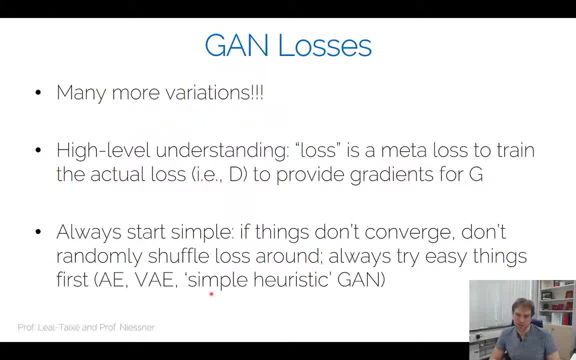 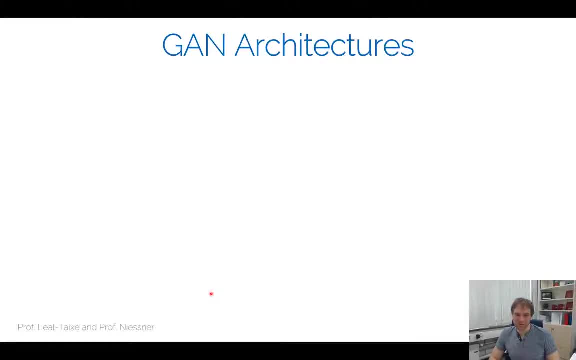 to evaluate or to see whether your GAN is working. I still have a few more slides, But I would like to roughly come to an end of this video Because we already have an hour and 38 minutes. I hope this was an interesting first introduction.